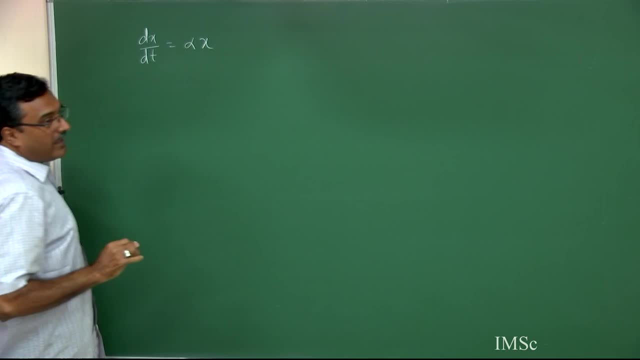 is equal to alpha x. Now, question: is that why this type of equations I am starting with? I am starting with this type of equation that is, first order linear equation or linear equation in two variables, only for the reason because, when we are interested to study the dynamics, 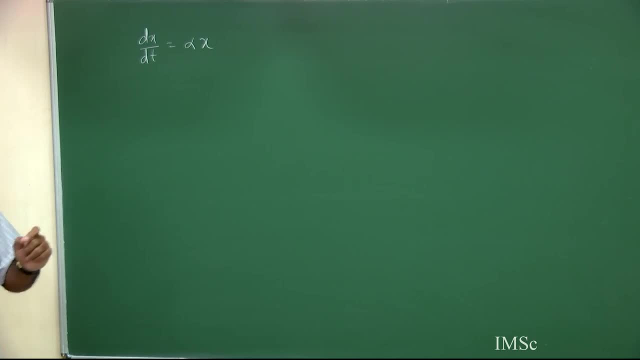 of continuous time population model, then these knowledges are very much important to understand the behavior of the system. That means how system works. That means how system evolves with the advancement of time. Now, in case of this equation, if you solve it, 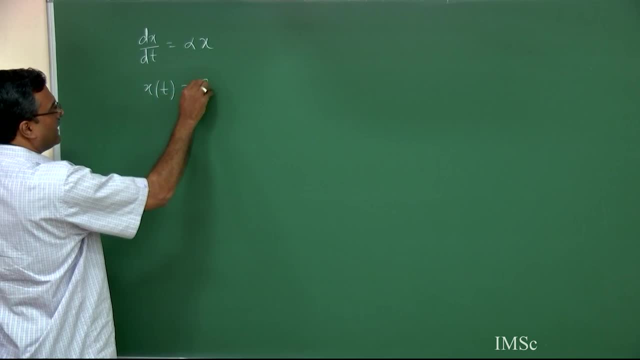 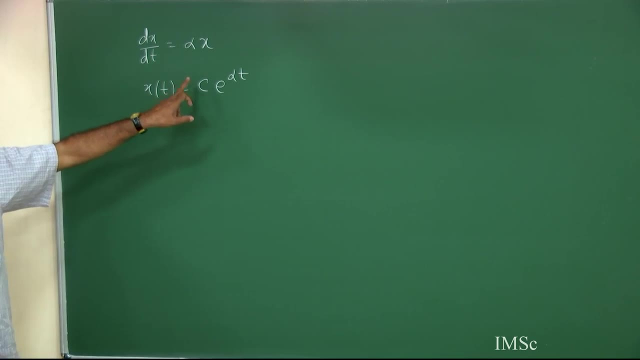 it is very easy to understand. the general solution for this system is given by c, e to the power alpha t. Now, if your this arbitrary constant, c is 0, determined by the initial condition. so you are having a trivial solution for this system. that is x, t equal to 0. Now 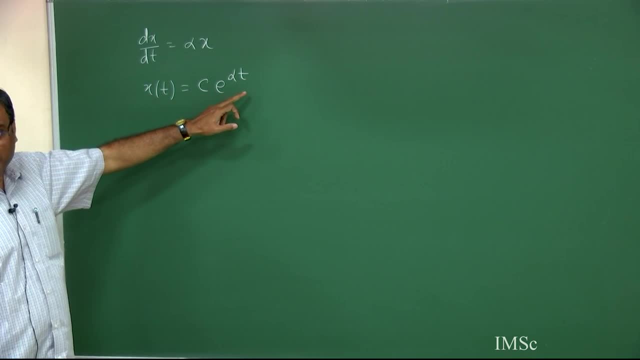 x will evolve with the advancement of time, either towards 0 or away from 0.. So the idea is that if your alpha is negative, then x t approaches to 0, irrespective of the condition that, whether c is positive or negative. But the idea is that if c is positive, alpha is: 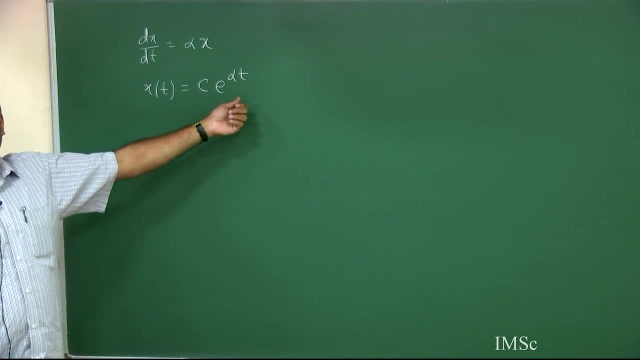 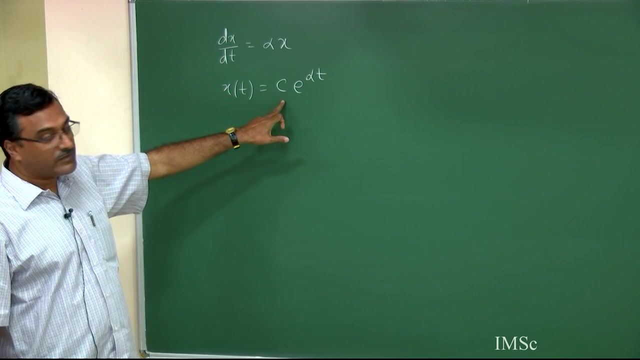 negative, then solution will be approaching to 0 through the values x greater than 0. And if, in case, your x 0 is negative because, whatever condition, you are substituting for t equal to 0 and corresponding value of x 0, that will determine what is the actual value. 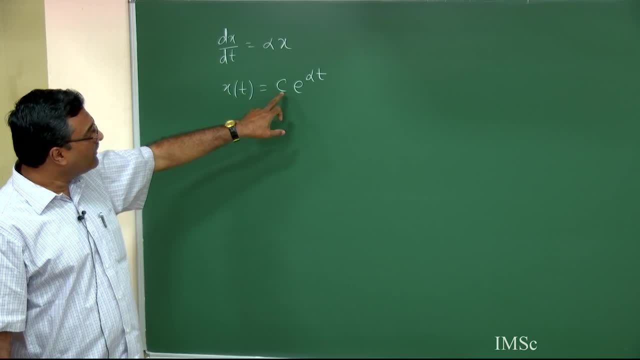 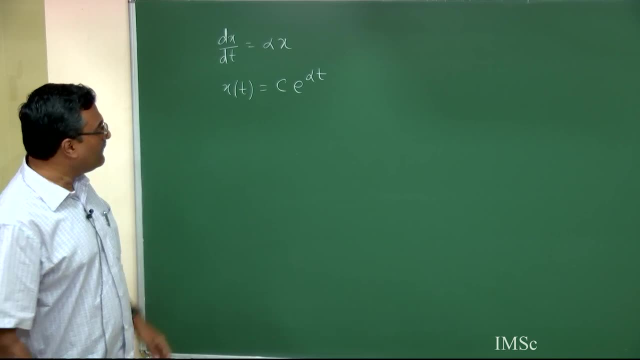 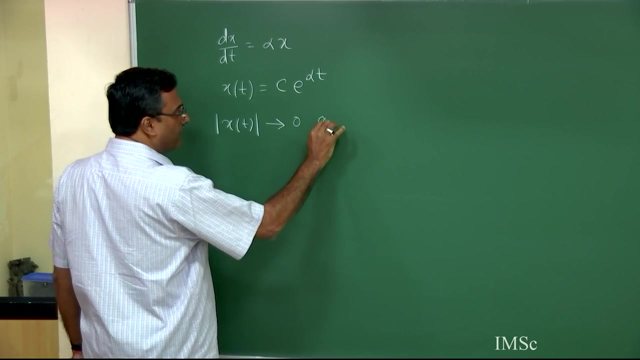 of c for the initial value problem, Then for c less than 0 and alpha less than 0, solution will be approaching to 0 as t tends to infinity. So come back to the question. So, combining this result, we can write that modulus of x- t. this approaches to 0 as t tends. 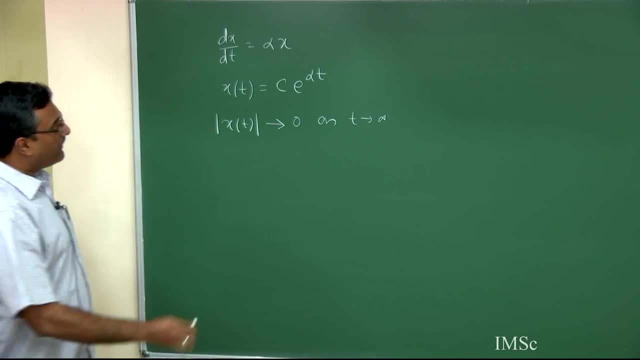 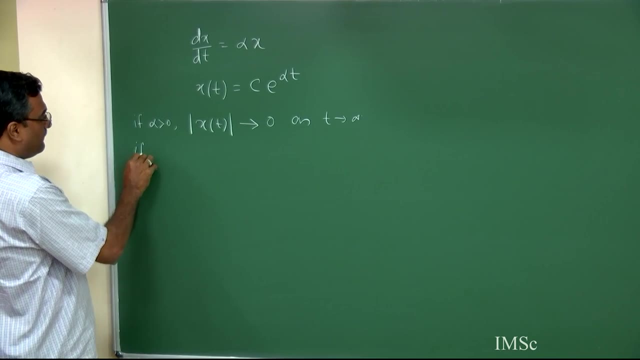 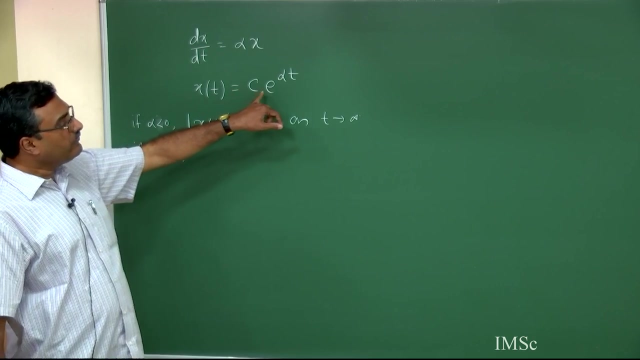 to infinity, whenever this holds, whenever that is alpha greater than 0. And in case if your alpha- sorry, extremely sorry- this is less than 0 and in case alpha greater than 0. So solution will be diverging either to plus infinity or minus infinity, depending upon the condition. 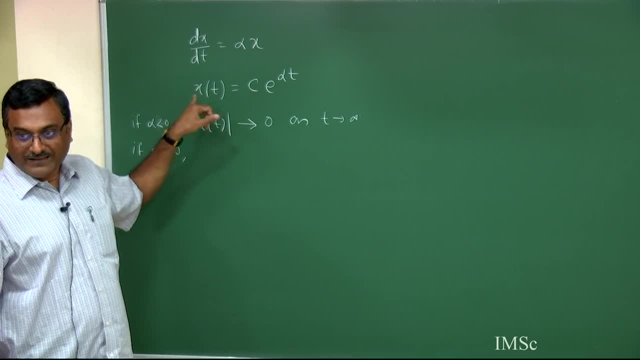 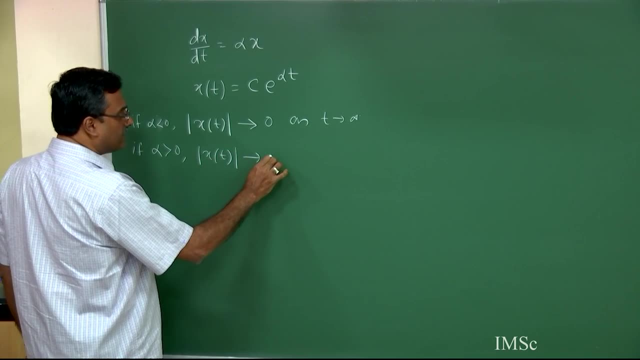 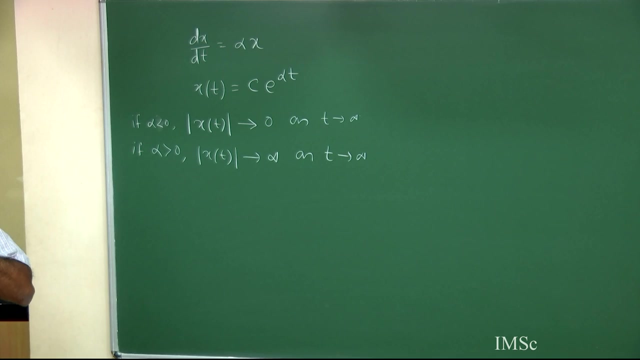 depending upon whether c is positive or negative respectively. So in case of alpha greater than 0, we will be having modulus x- t. this is going to infinity as t tends to infinity. So this is the only single variable equation, linear equation, and coefficient is: 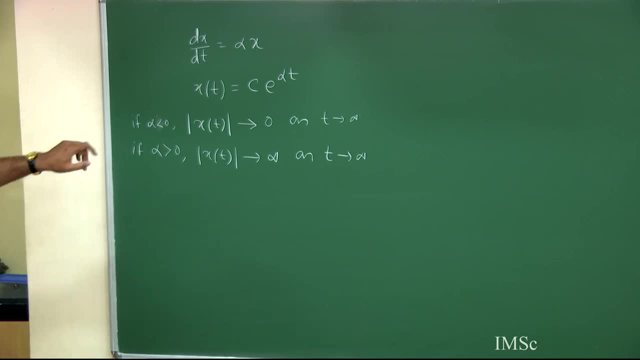 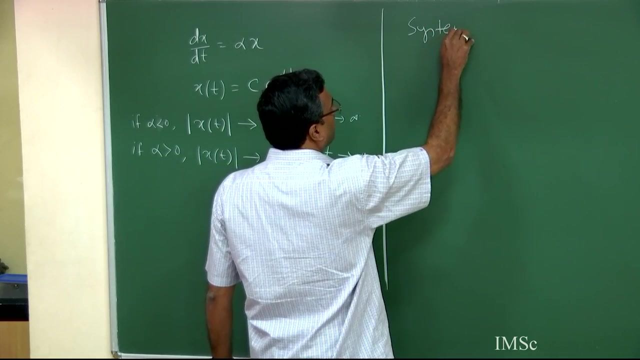 constant. So this is autonomous equation in the sense that the time variable t does not appears into the equation explicitly. So d, x, d, t equal to alpha x. Now we move over system of linear equations, system of c, linear equations in 2 variables. 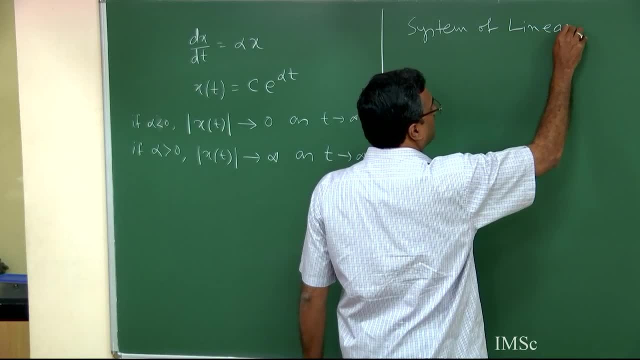 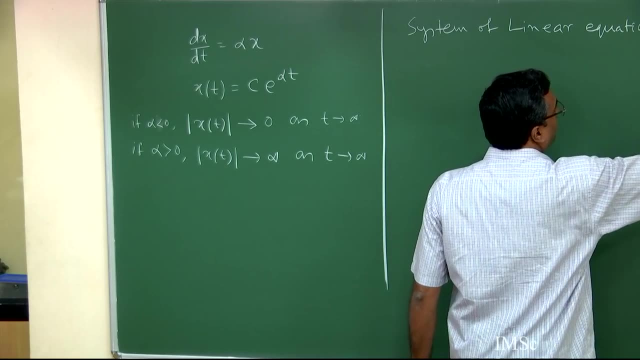 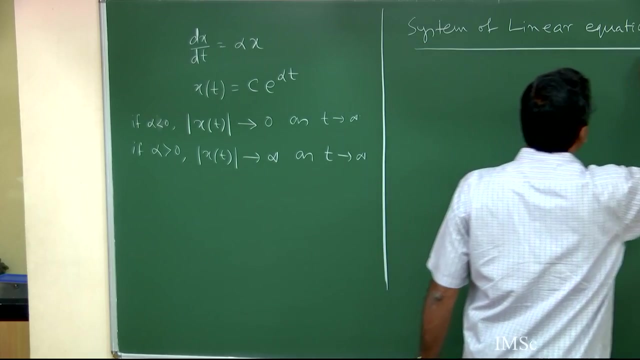 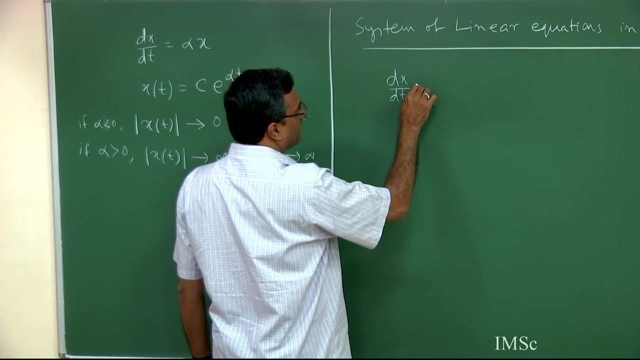 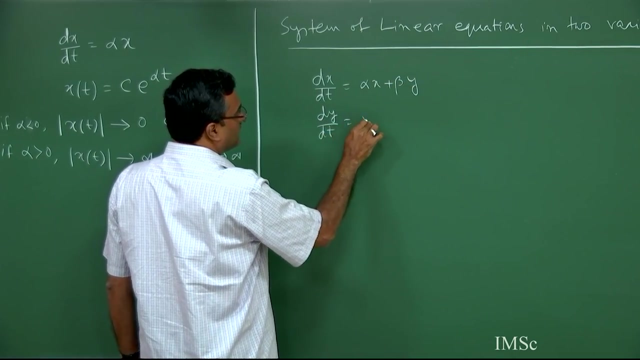 So the general form for the experimentation problem is a simple harmonization of ausion sequence. Okay, Yes, system of linear equations in two variables. we can write into the form that is: d x, d t, this is equal to alpha x plus beta y, and d y d t, this is equal to gamma x plus delta. 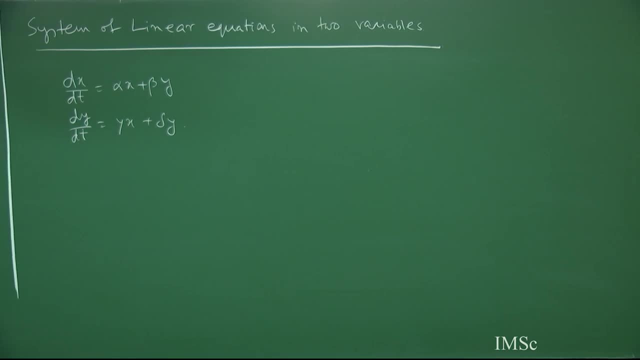 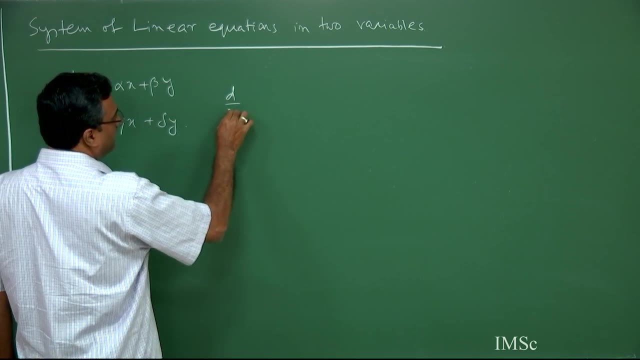 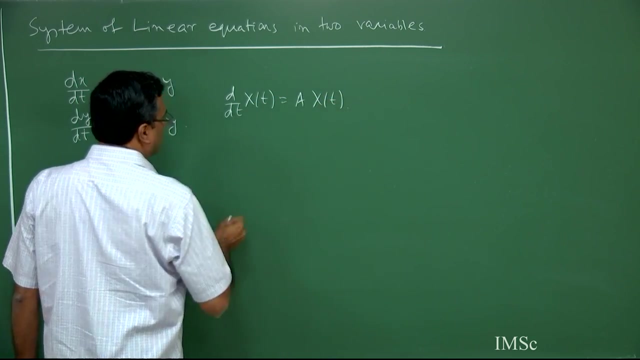 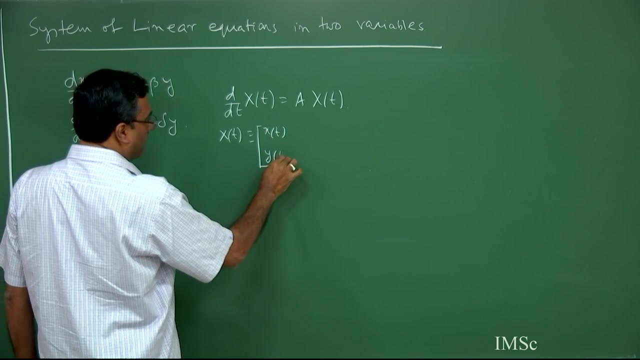 y. This is the most general form for the system of linear equations in two variables and you can put this linear system into a matrix form that is d, d t of capital, X t. that is equal to a of X t, where X, t, this is equivalent to two variable column matrix: X t, y, t and capital. 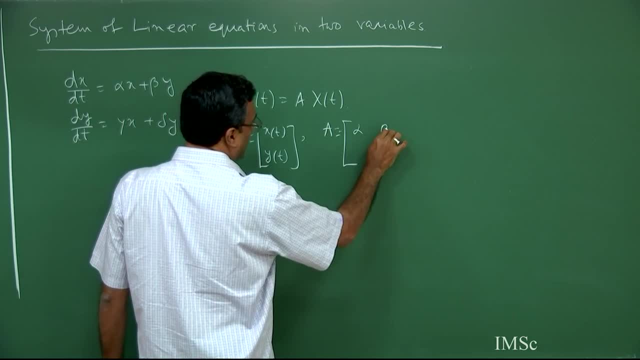 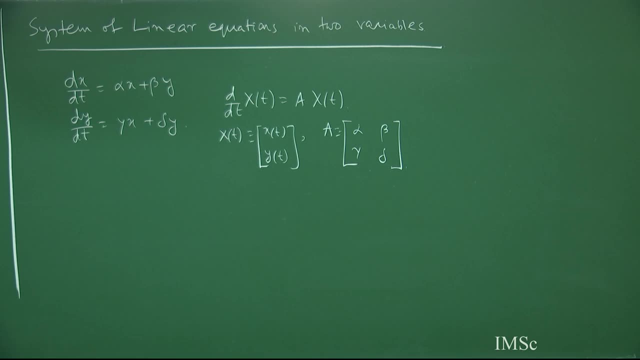 a is the 2 cross 2 matrix, alpha, beta, gamma, delta. So this is the two variable system. Now the question is that how we can find out solution for this system of linear equations. The idea is that, in order to find out a solution for this linear system, 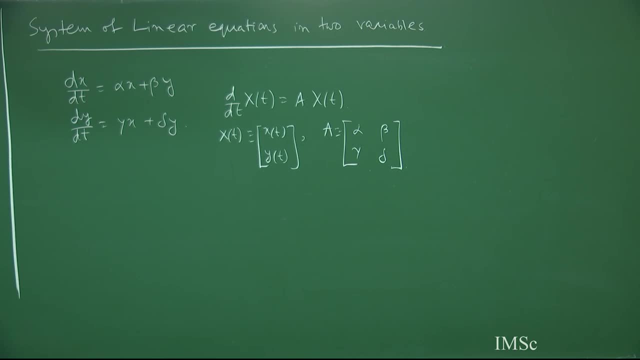 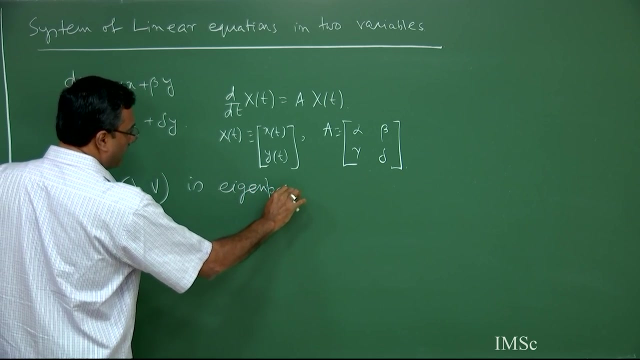 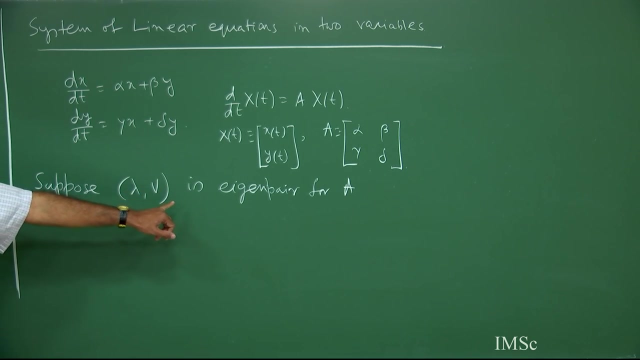 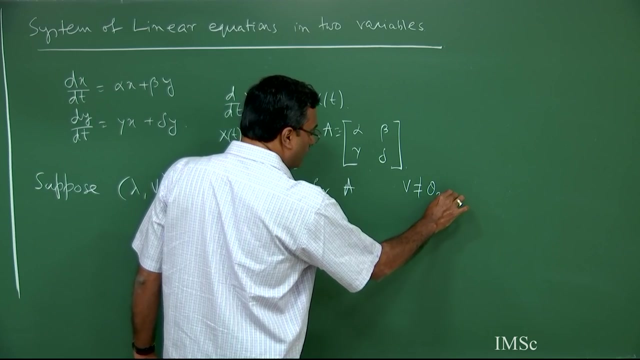 we use a very basic theorem. Theorem states that suppose lambda comma v is Eigen pair is Eigen pair for capital a. So that means lambda is the Eigen value and v is the associated Eigen vector. So it means that you have a non null 2 cross 1 matrix v, such that a v equal to 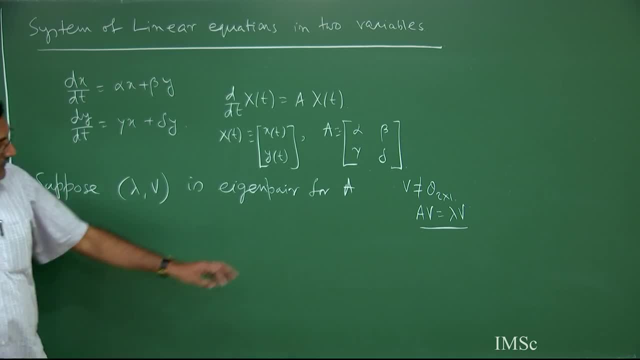 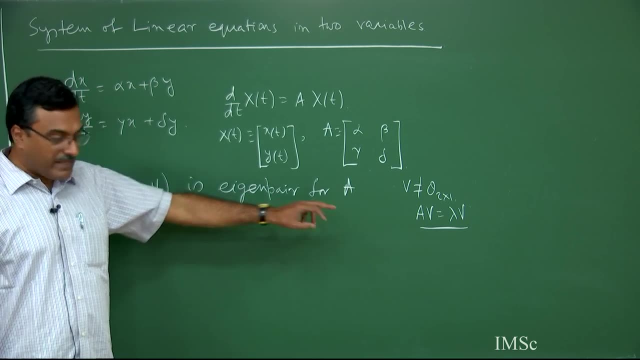 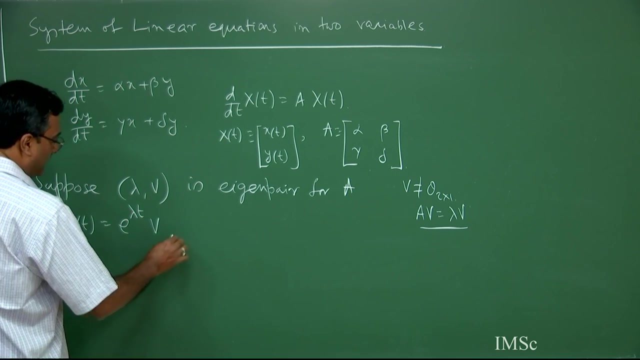 lambda v. this equation holds. So therefore, lambda is the Eigen value and v is the associated Eigen vector. Now, if this is a Eigen pair for this system, then X- t- this is equal to e, to the power. lambda t multiplied by v is a solution for. 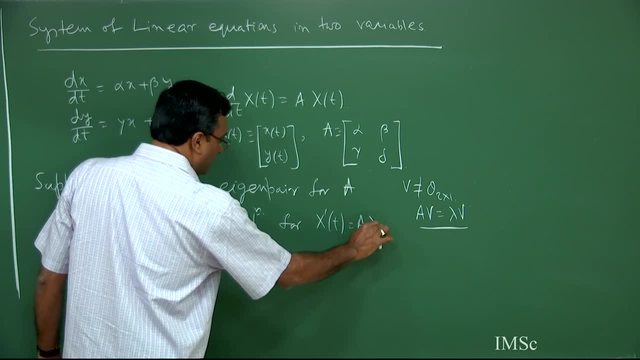 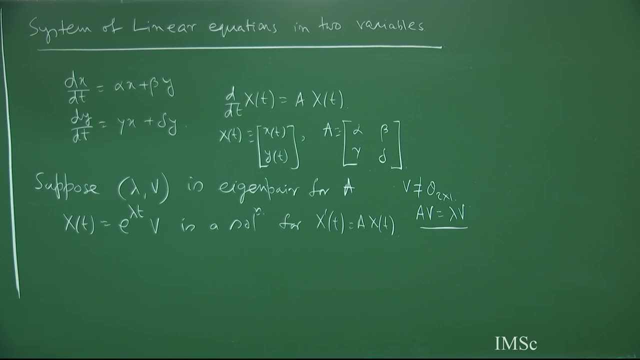 the system X dot t that is equal to a X t. We can explore this idea, or rather, we can say that we can utilize this particular idea in order to find out the general solution for this system of linear equations. Now, roughly, I will give you a quick proof of this result. why this? e to the power lambda. 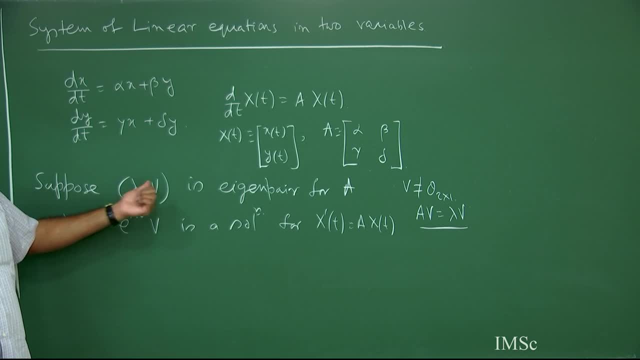 t into v is going to be a solution of this equation. So in order to prove it, we just need to show that this X, t equal to e, to the power lambda t into v satisfies this equation. Now keep in mind: v is the Eigen vector, lambda is the Eigen value, So lambda is a constant. 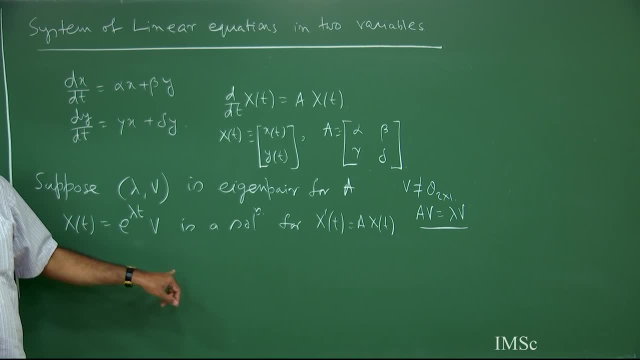 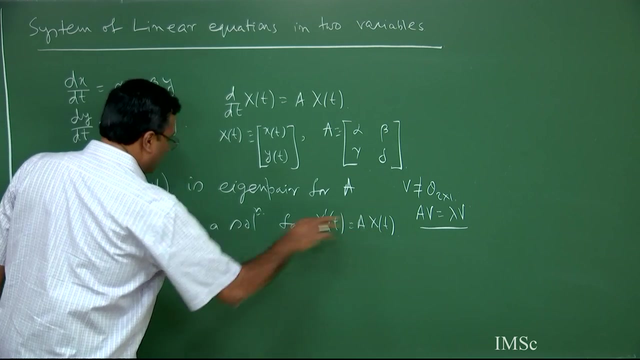 quantity and v is a two component column matrix. So if you differentiate X, t with respect to t, so that is X dot t, this will results in that is lambda e to the power, lambda t. this is into v. Similarly, if you replace X t by e to the power, 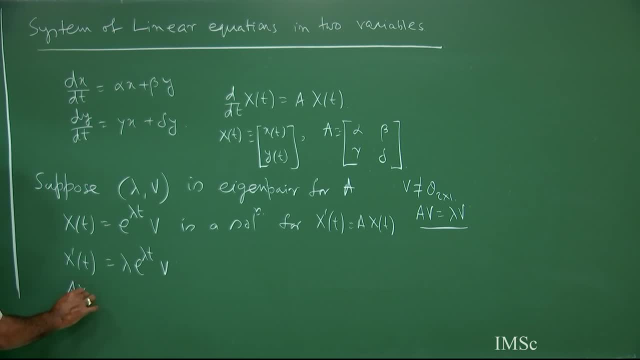 lambda t into v on the right hand side, then you will be having a X t equal to a times e to the power lambda t into v, So e to the power lambda t can be multiplied by v into a A x t equal to A times e to the power lambda t into v, So e to the power lambda t can be. 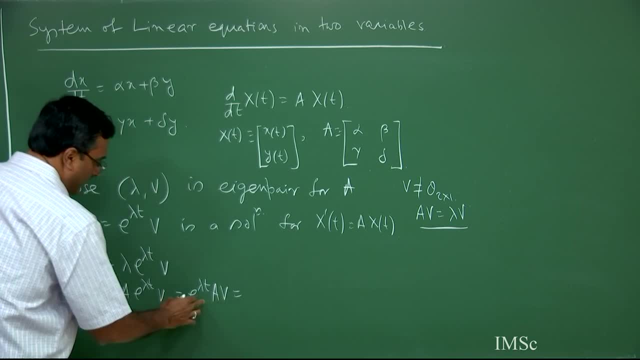 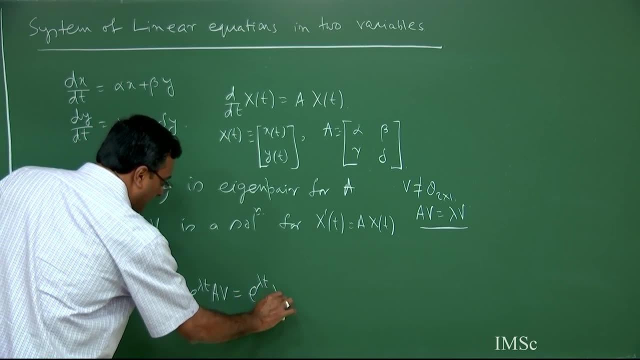 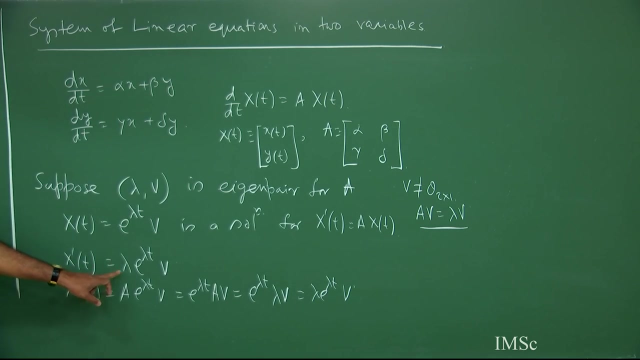 placed at the beginning, then multiplied by a v. Now v is the eigenvector with associated eigenvalue, lambda. So therefore you will be having e to the power lambda t times lambda v. So this is equal to lambda e to the power lambda t into v, So this equal to this one. 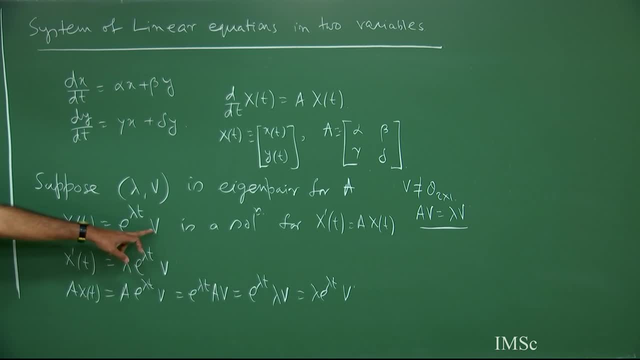 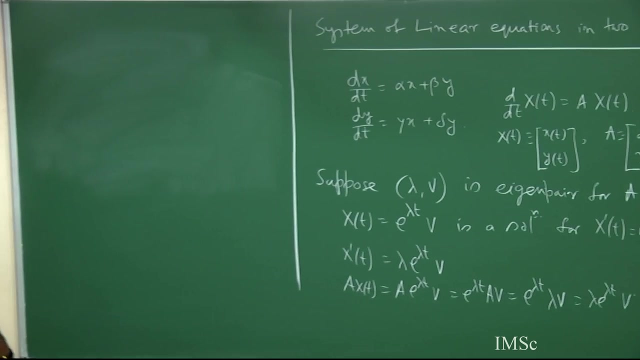 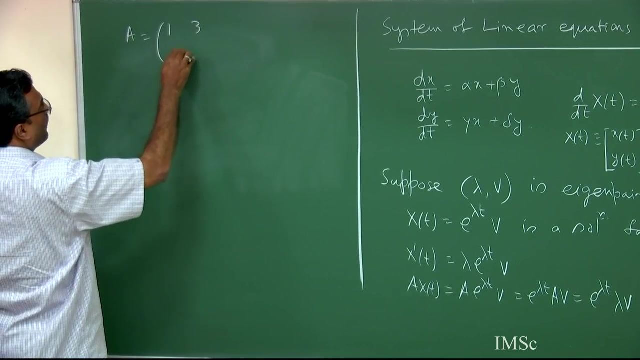 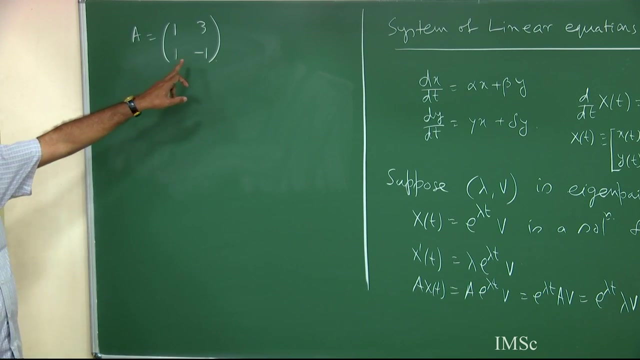 right. So therefore, e to the power lambda, t into v is a solution for this linear system. Now we can have a specific example for this system. A specific example is: you consider: A is a matrix, 1,, 3, 1, minus 1.. This is the matrix. Now you can find out the eigenvalues. 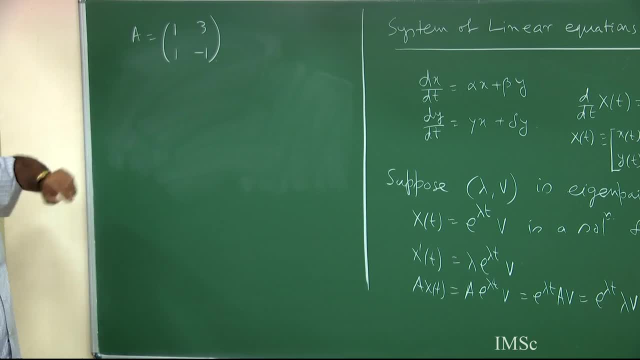 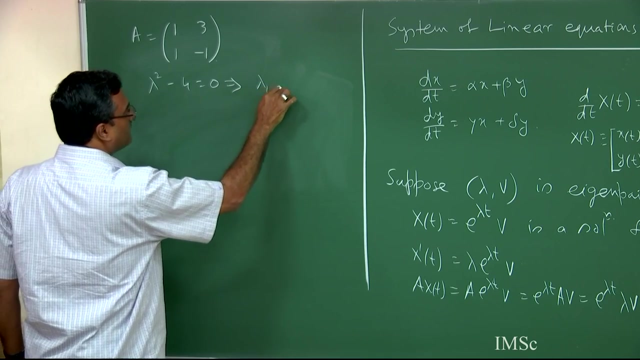 of this equation quickly. You can just check here: trace is 0.. A determinant is minus 4, right? So therefore characteristic equation will be lambda square minus 4 equal to 0, implying the eigenvalues lambda 1, 2.. These are 2, minus 2.. So these 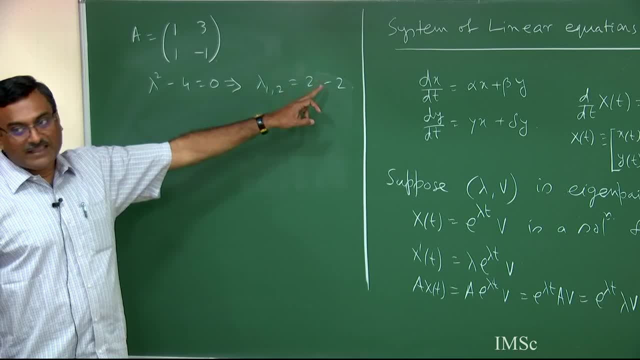 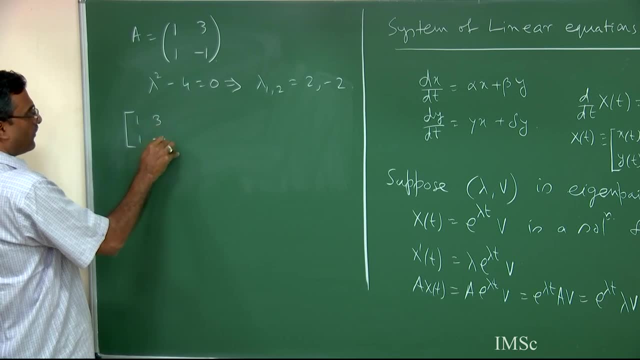 are two eigenvalues. So, first of all, we can try to find out the eigenvector associated with the eigenvalue 2.. So then, if you solve this equation- 1, 3, 1, minus 1,, this v1, v2. 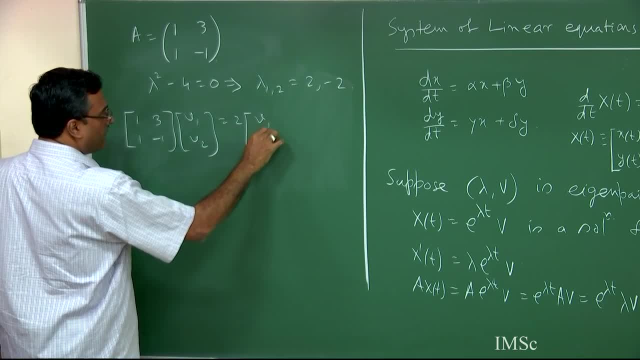 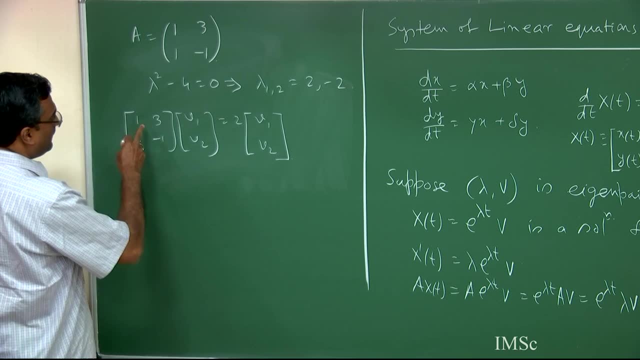 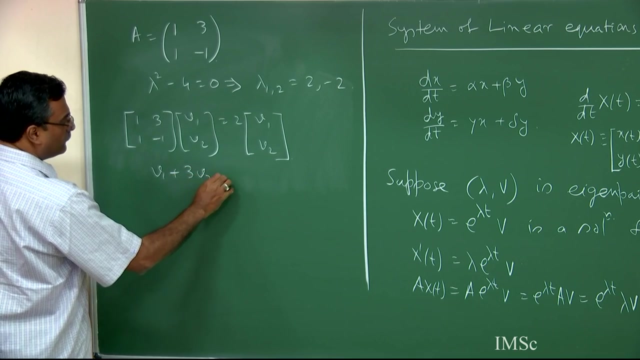 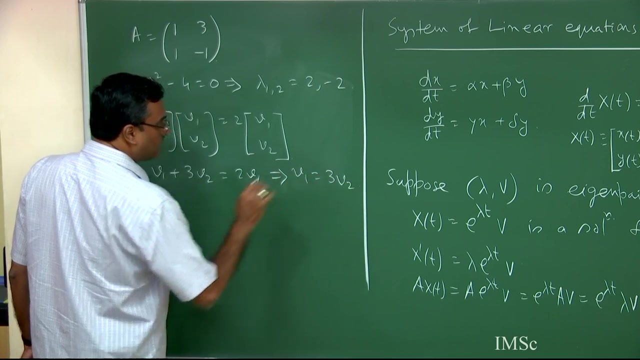 this is equal to 2 times v1, v2, this one. So then you can find out this first equation as v1 plus 3 v2.. This is equal to 2 v1.. This implies v1 equal to 3 v2.. Now, if you consider, 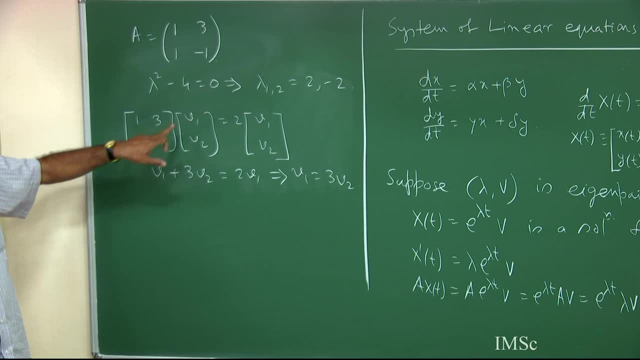 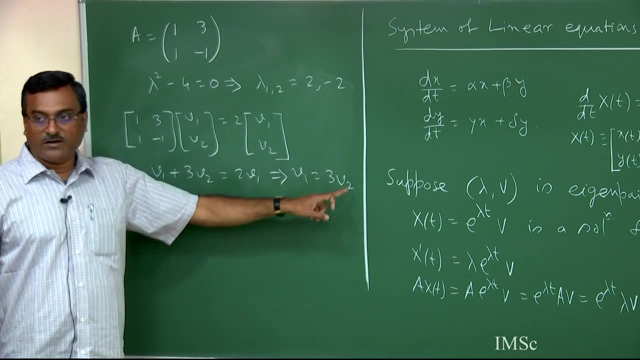 the second component. So you will be having v1 minus v2 equal to 2 v2.. So again, you will be having the same equation: v1 equal to 3 v2.. So the second equation is redundant here Now in order to 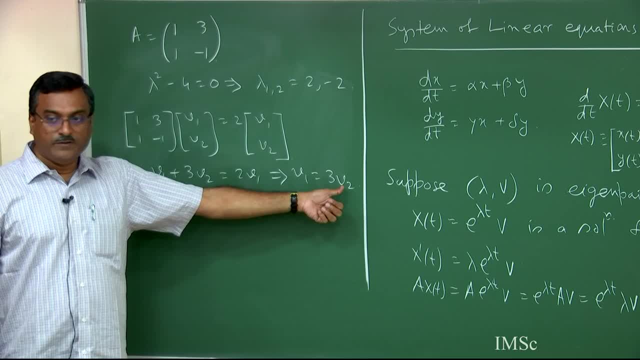 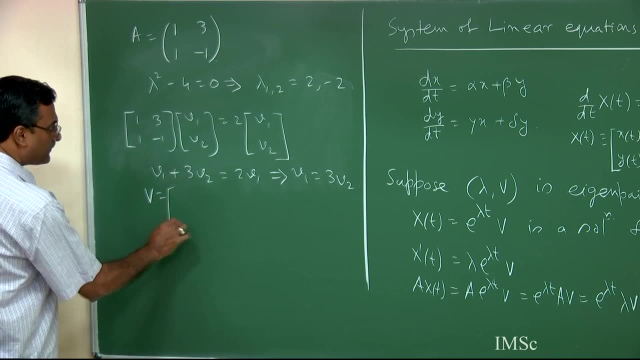 find a solution for v1- v2,. cleverly we can choose: v2 is equal to 1.. So automatically you will be having v1 equal to 3.. So then associated eigenvector v comes out to be 3,. 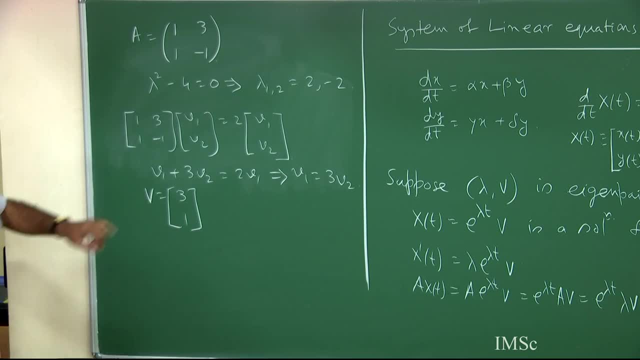 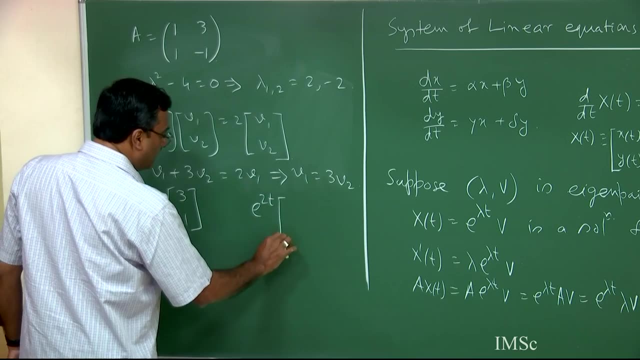 1.. So this is the eigenvector. Now, if you just add this, Hai v1 plus, this is the corresponding eigenvalue. So one solution that is given by e to the power 2t. this multiplied with 3, 1.. So this is the vector. So this: 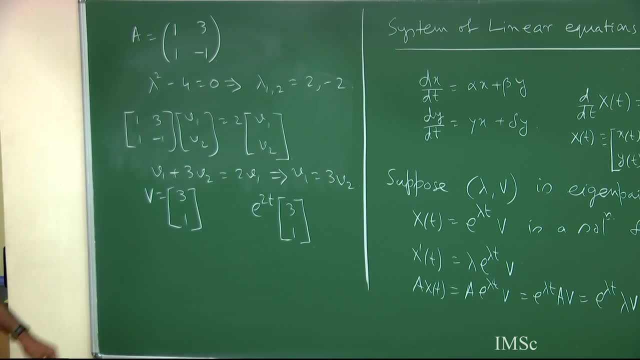 is one solution for this system. Similarly, if you calculate that eigenvector associated with the eigenvalue minus 2, then you will be having the next eigenvector as 1 comma minus 1.. You can verify. Just suppose this is your minus 2.. 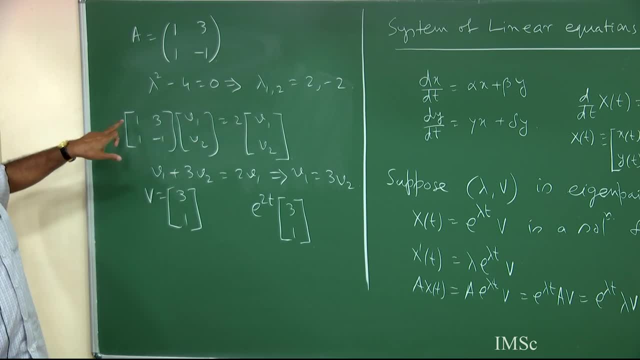 So if this is your minus guy, if I form it as 1 over the staring has given by 2, which is not going to come, So it does not help, but essentially I am is your minus 2, then you will be having 3 v 1 plus 3 v 2, equal to 0. So that means 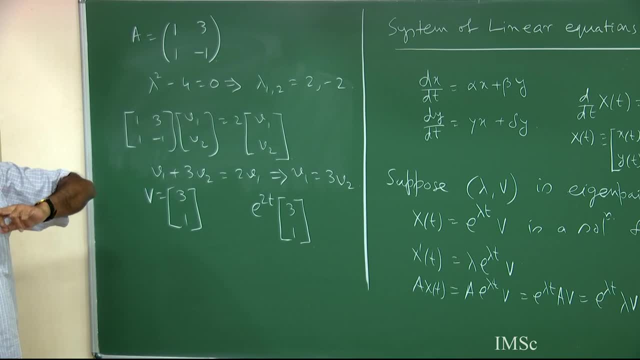 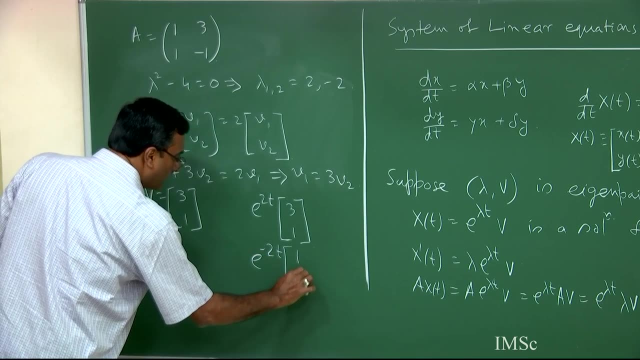 v 1 plus v 2 equal to 0. So which gives v 1 equal to 1 and v 2 equal to minus 1.. So second solution is: e to the power minus 2, t 1 minus 1.. So these are actually two solutions. 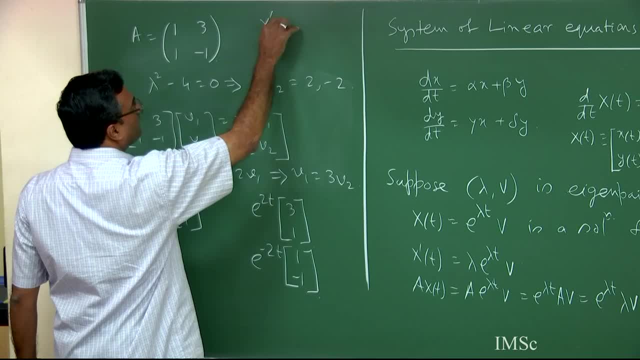 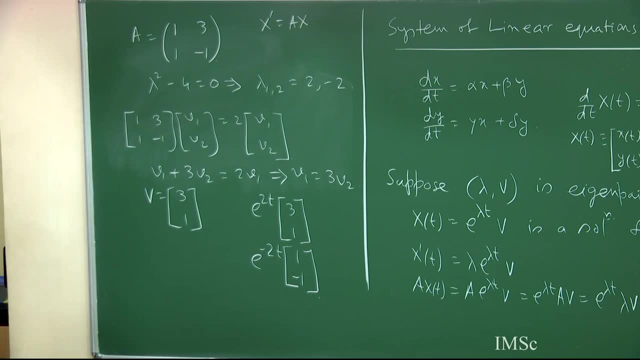 for the system of linear equations, that is, x dot is equal to A, x, where A is given by this particular matrix. Now, once you have these two solutions- I am not going into the mathematical depth, but you can prove- these two are two linearly independent solutions And, as the given system, 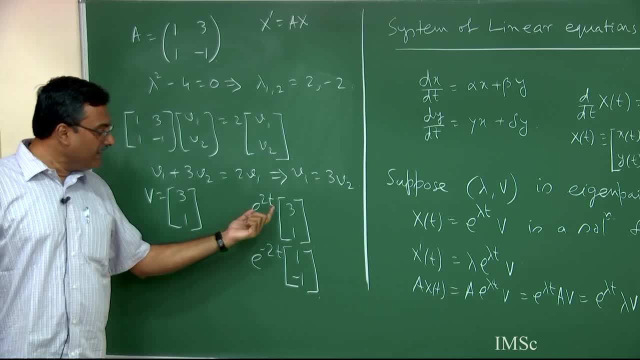 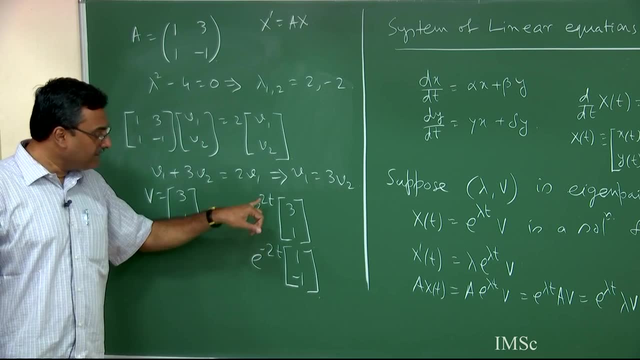 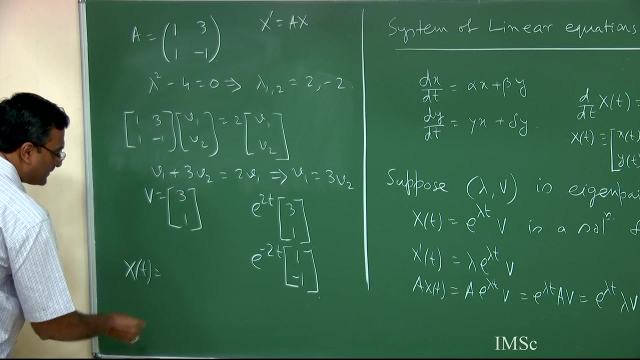 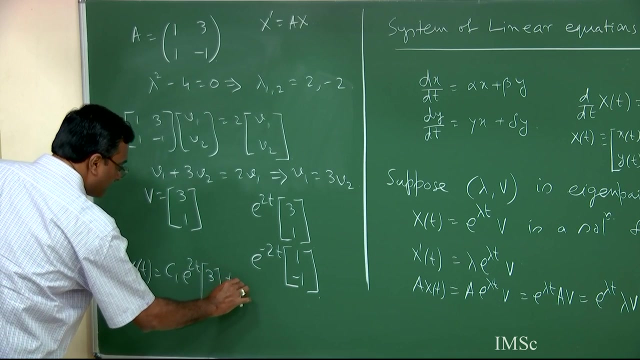 of linear equation is a linear equation, So any linear combination of these two solutions is also solution for the sorry given system, and hence we can write the general solution for the given system as: x, t equal to c, 1, e to the power 2, t, 3, 1 plus c, 2, e to the power minus. 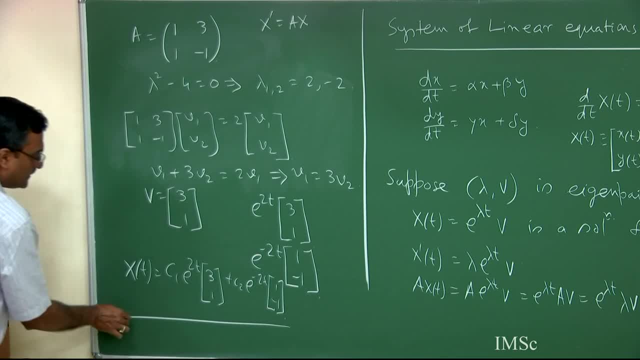 2 t, 1 minus 1.. So this is the general solution for the given system of linear equations. Now the point is that, in order to understand the phase portrait, it will be quite difficult to understand that how phase portraits are coming out if we working with a general format. 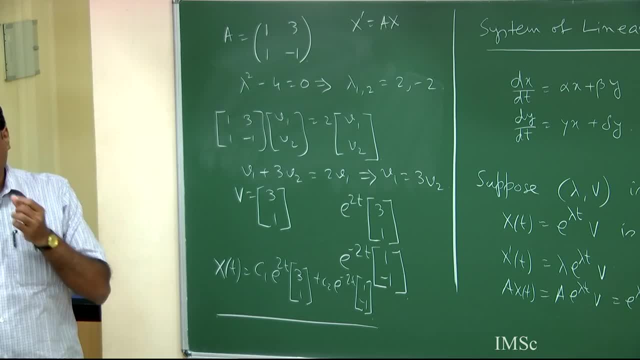 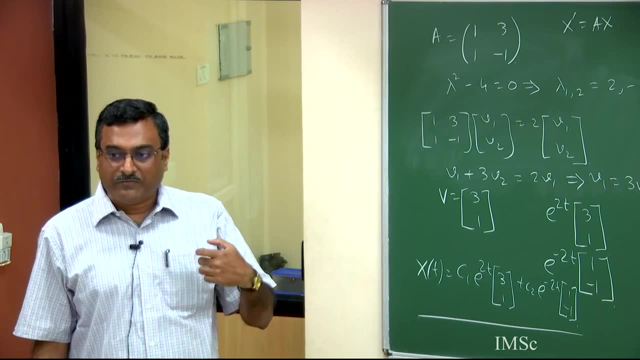 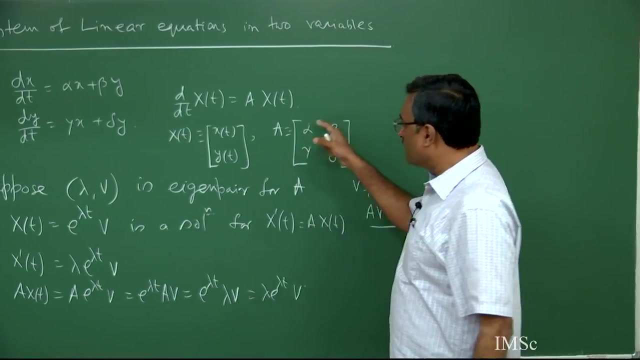 of this kind of matrix: alpha, beta, gamma, delta. Rather, we can consider three specific type of matrices, depending upon the nature of Eigen values of a 2 cross 2 matrix. For this general system, you know that your matrix is a 2 cross 2 matrix, So there will be two Eigen values. 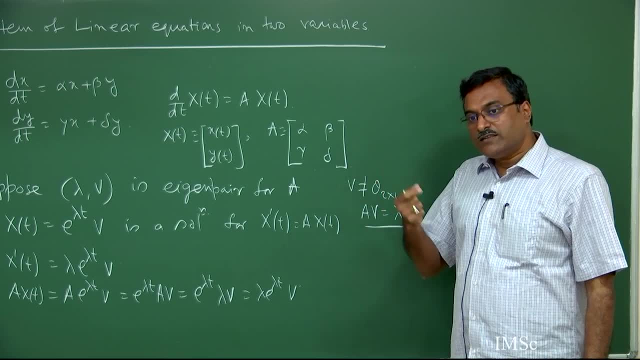 associated with this matrix, capital A. So what are the different properties of this matrix? So what are the different properties of this matrix? So what are the different properties of this matrix? So what are the different possibilities for the Eigen values associated with this matrix, capital A, The 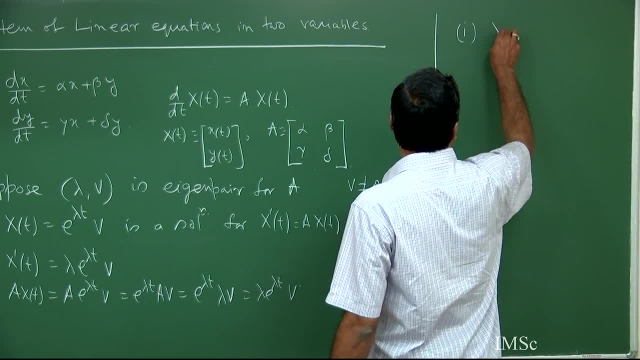 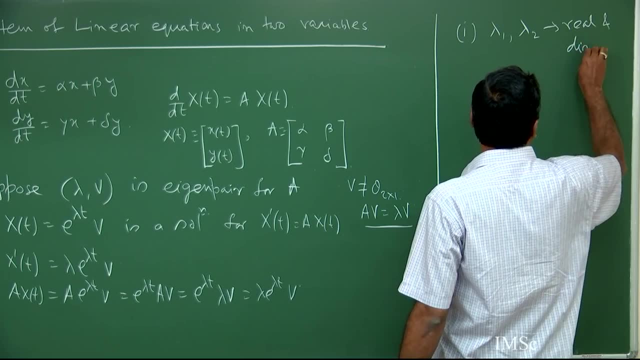 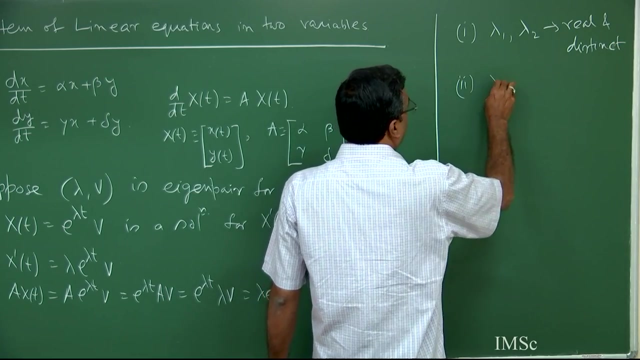 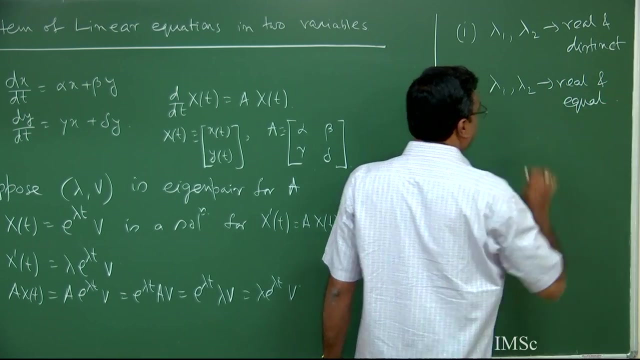 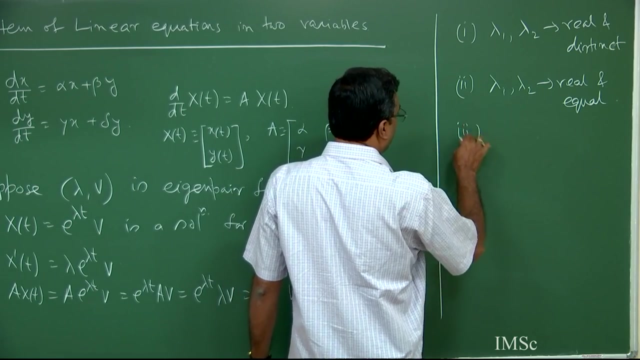 possibilities are: number 1,: both the Eigen values: lambda 1 and lambda 2, they are real and distinct right. they are real and distinct. Number 2,: lambda 1 and lambda 2, they are real and equal Right. So both the roots are real and equal. Number 3,: lambda 1 and lambda 2, they are complex. 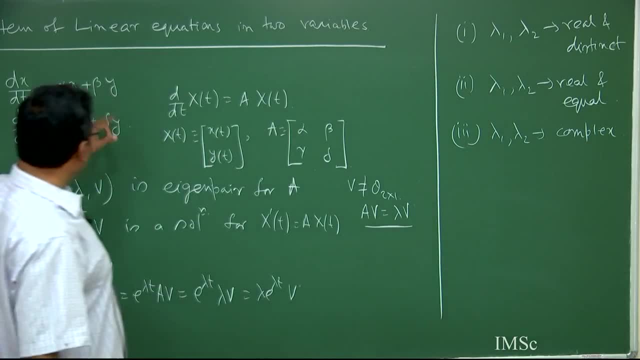 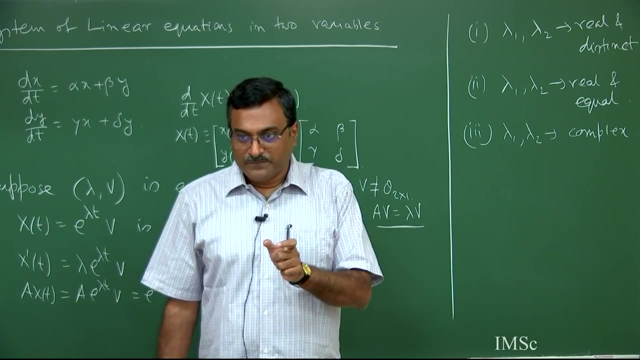 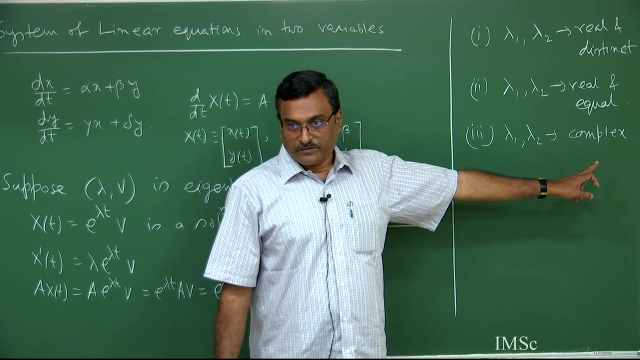 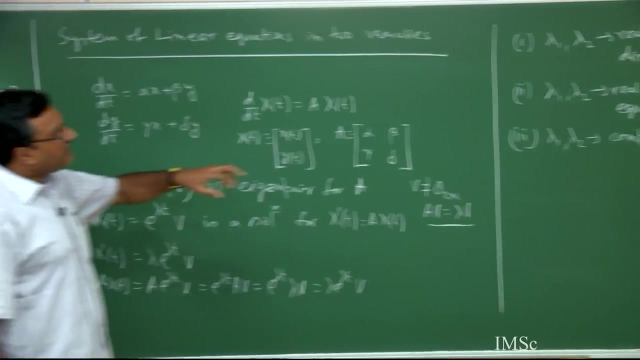 Now, as we are assuming all the coefficients- alpha beta gamma delta, they are real. So therefore, coefficients of the quadratic equation are real quantities. So therefore these two complex Eigen values should be complex conjugate Eigen values. right Now, if you have a matrix alpha beta gamma delta, of the form alpha beta gamma delta and 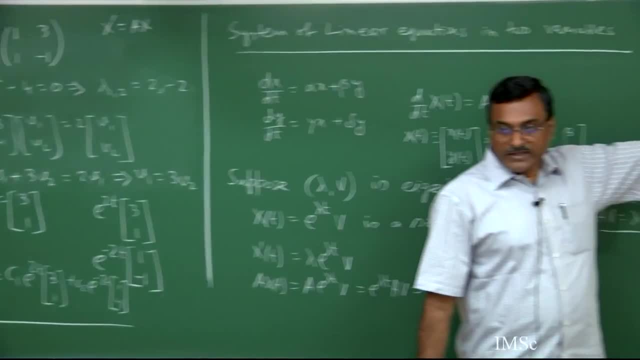 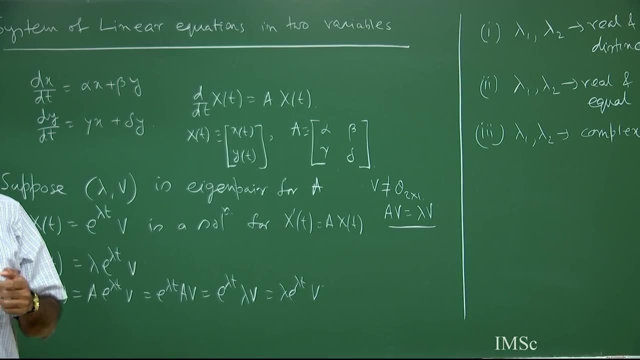 two real, distinct Eigen values, lambda 1 and lambda 2, it can be converted to its corresponding Jordan canonical form, that is, lambda 1, 0, 0, lambda 2.. Afterwards I will be showing you a particular example how you can derive the Jordan canonical form. 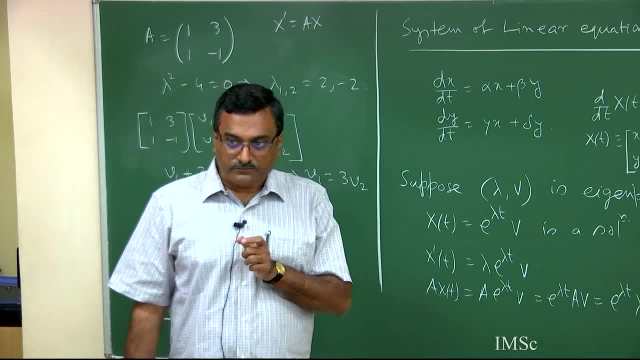 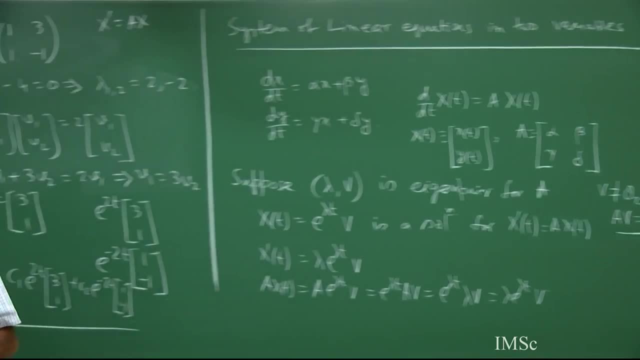 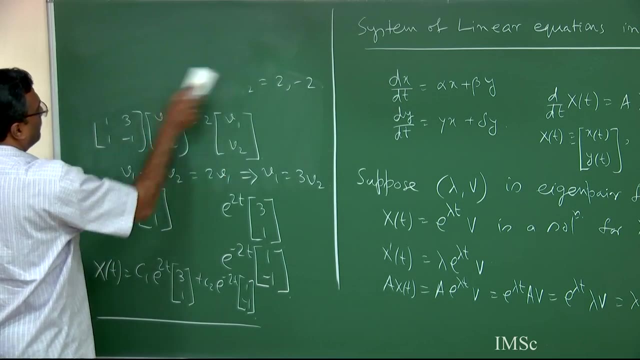 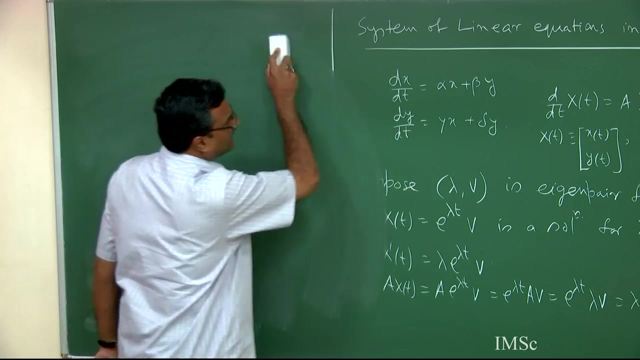 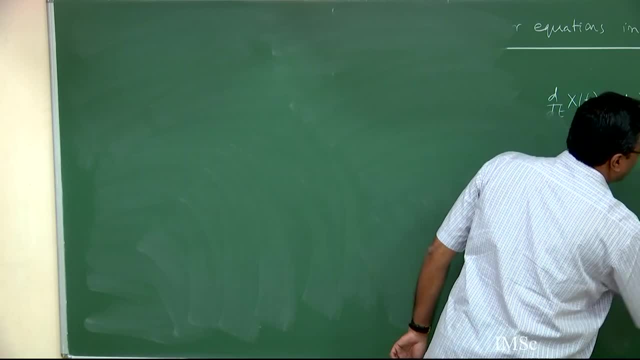 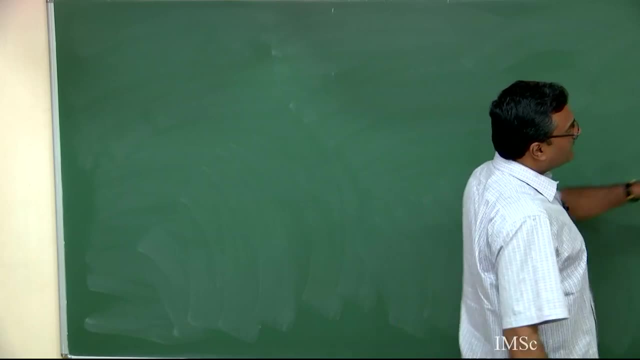 Malaysia'sěs. another slide is singедин: how can you create 360.5, That is also 1 by 2 lambda over mega zeta of x and THAT? of course, in this case we can consider both the cases, that is, Eigen values are real and 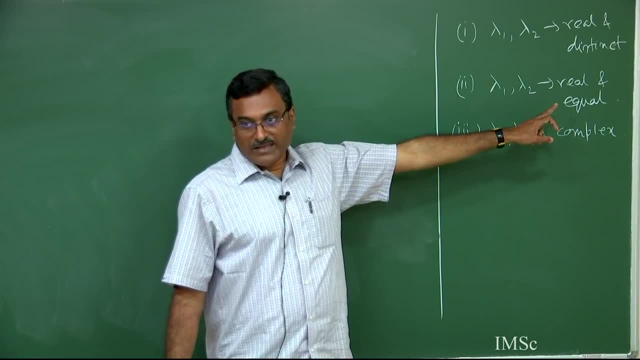 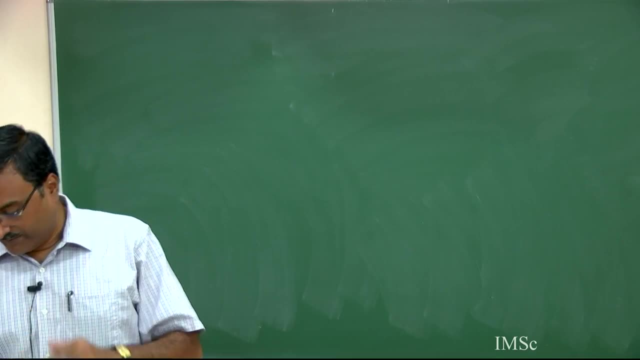 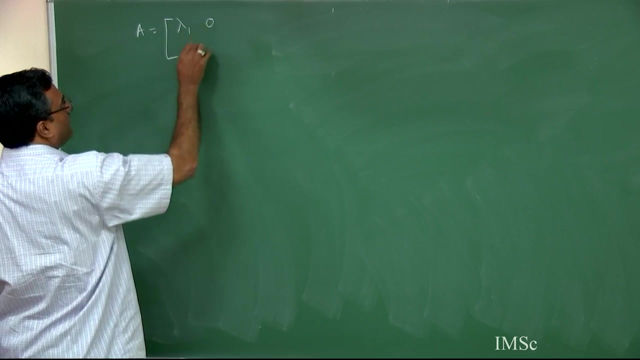 distinct as well as they might be equal. But in case of two equal Eigen values, they are two different Jordan canonical forms. I will come to that point later. So for first case we consider A equal to, in a general format, lambda 1, 0, 0, lambda 2.. So 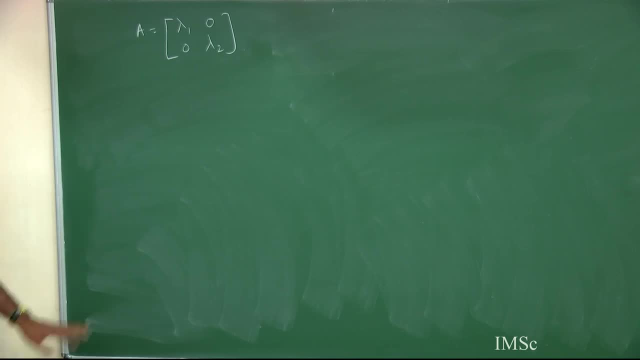 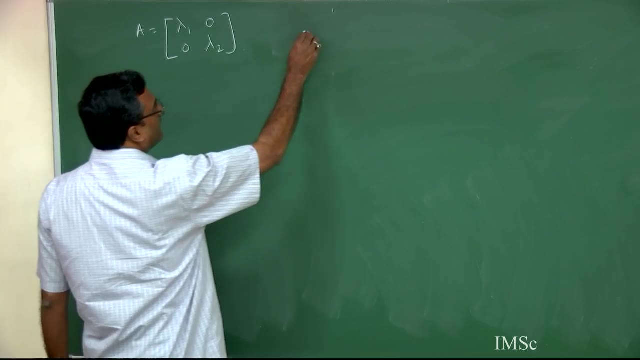 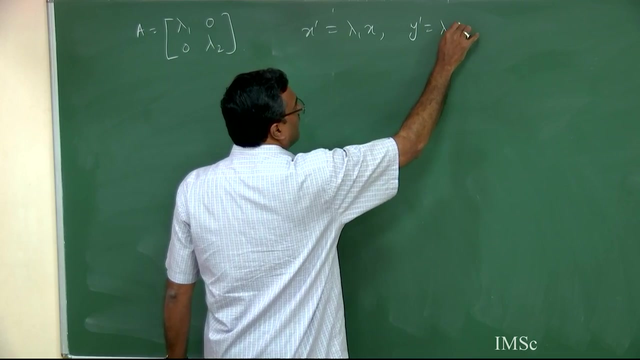 this is the matrix, capital A, So of course its corresponding equations are decoupled equations, right? because if you write the corresponding equations, then your equations is going to be: x dot is equal to lambda 1, x, and y dot that is equal to lambda 2, y. you can solve. 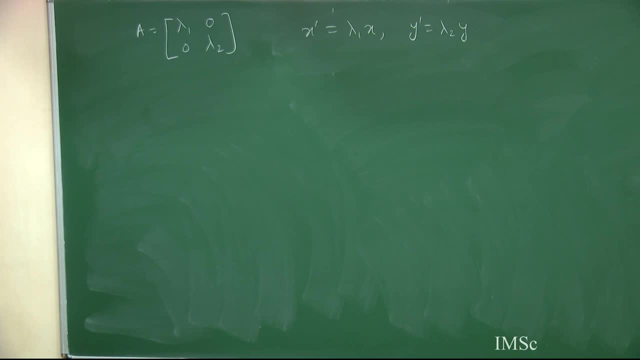 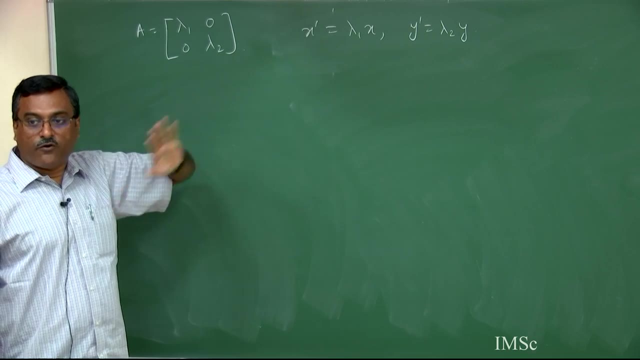 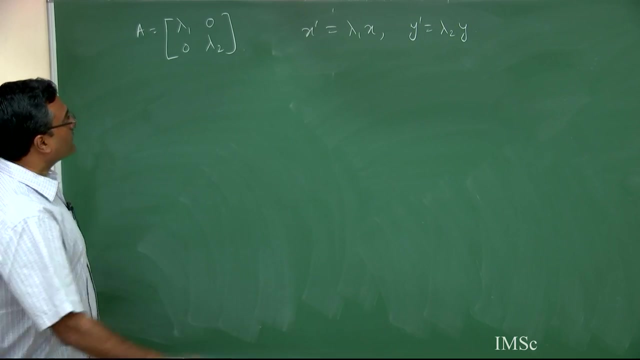 it independently, But as we are considering this as a system of linear equation in terms of matrix notation, So we follow this, So we follow this, So we follow the same approach. that means finding out the Eigen values, Eigen vectors, and then write down the general solutions. 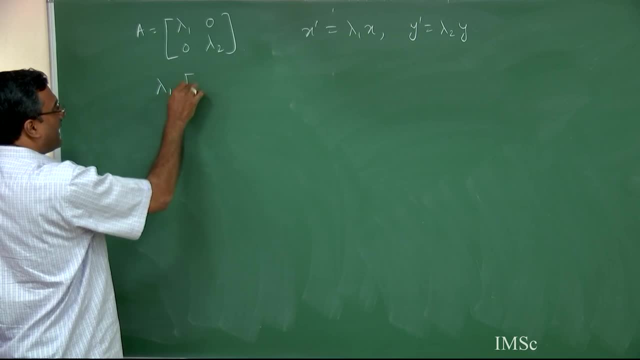 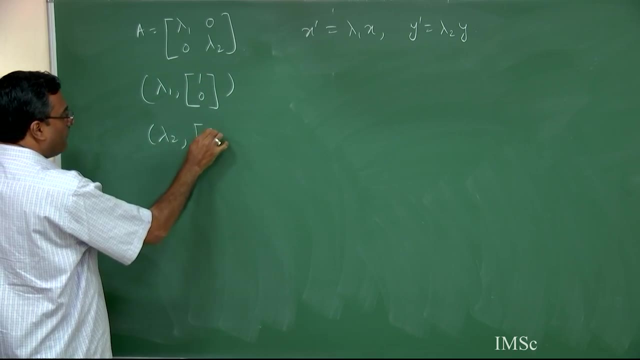 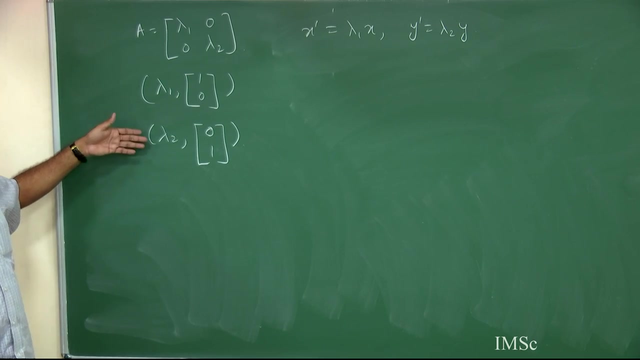 So what we are having here, lambda 1 is an Eigen value with associated Eigen vector 1 comma 0, and lambda 2 is an Eigen value with associated Eigen vector 0 comma 1, right? So once you have these two Eigen pair, automatically you can write down the solution for the given. 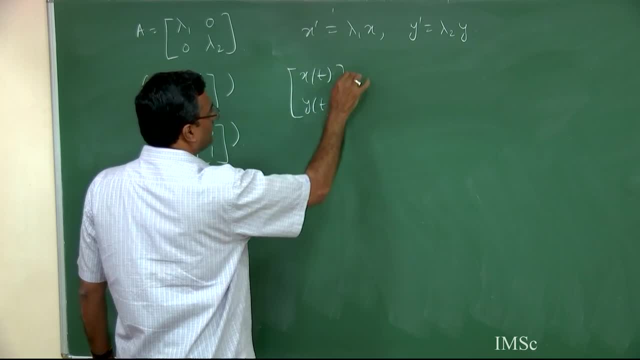 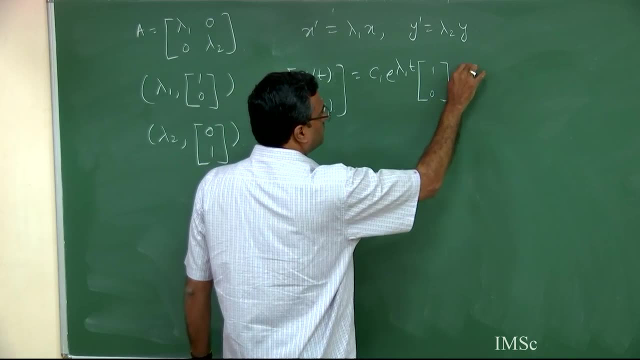 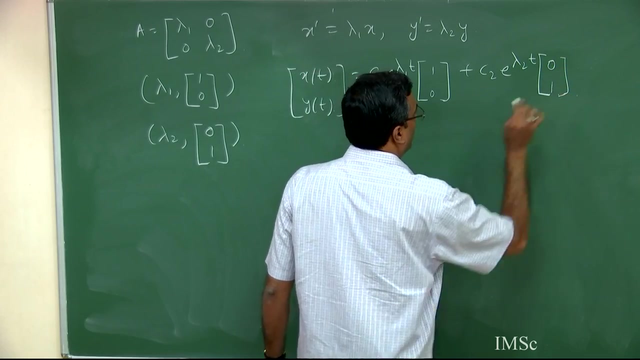 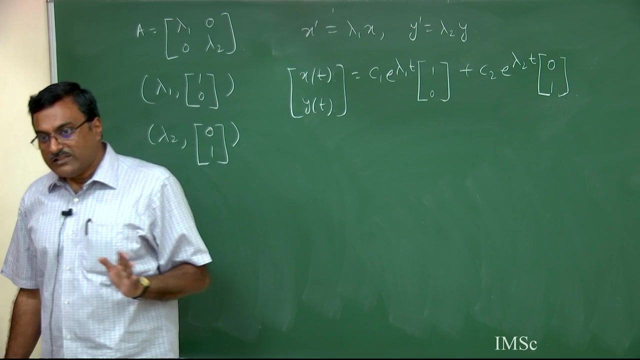 system That is x, t, y, t. that is equal to c 1 e to the power lambda 1 t 1, 0, plus c 2 e to the power lambda 2 t 0, 1. right Now, once you have this structure, that is the general solution. from here and onwards we. 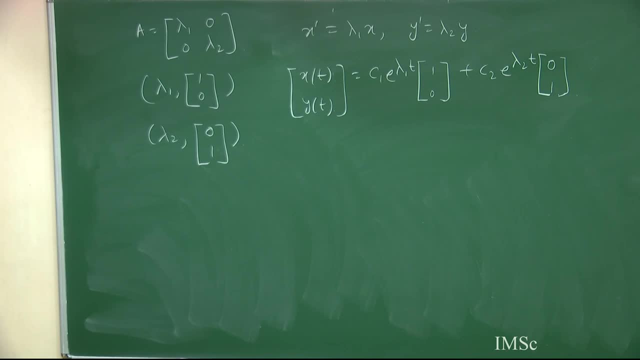 can try to understand how the phase portraits will look like. So we can try to understand how the phase portraits will look like. So, once you have this structure- that is the general solution from here and onwards- we can try to understand how the phase portraits will look like. 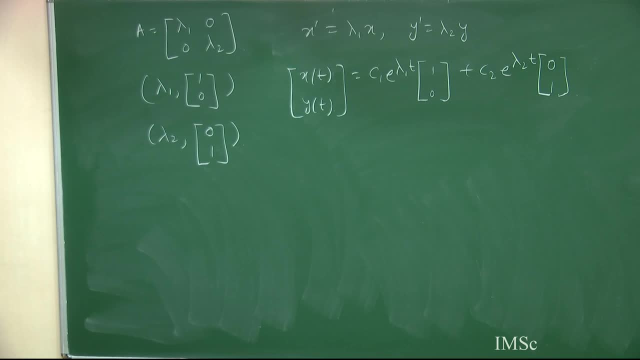 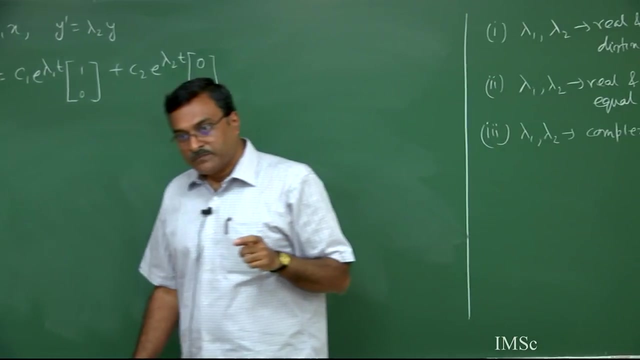 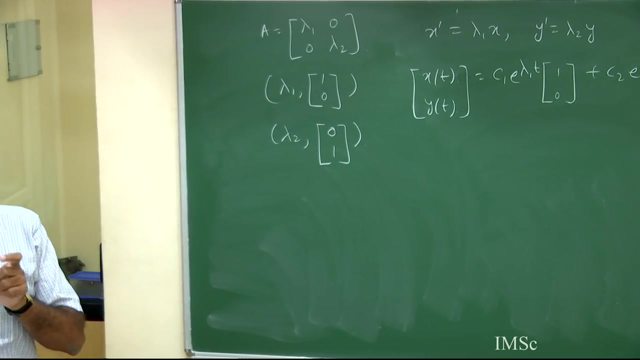 So that means in x, y plane how the solution trajectory behaves, or they can evolve with the advancement of time t. Now here I will be considering two specific example, because once you have two real, distinct Eigen values, there are three different cases. Three different cases means both the Eigen values are real and negative, both the Eigen 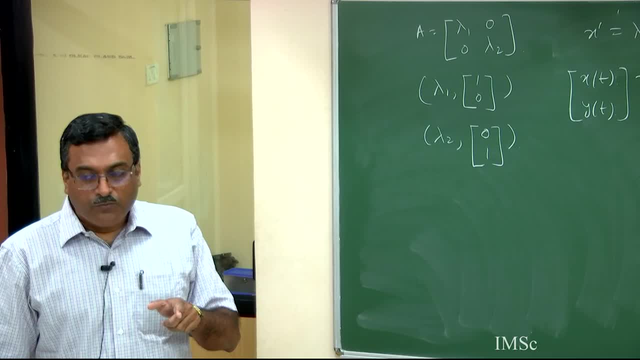 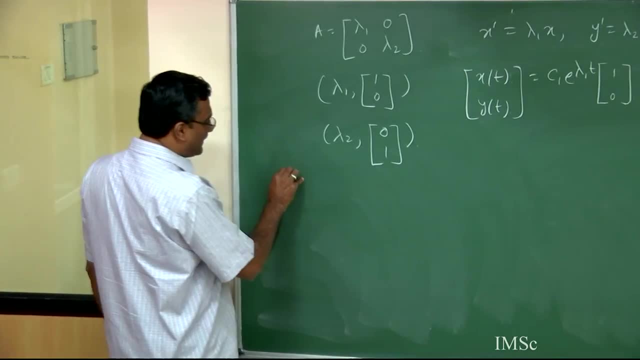 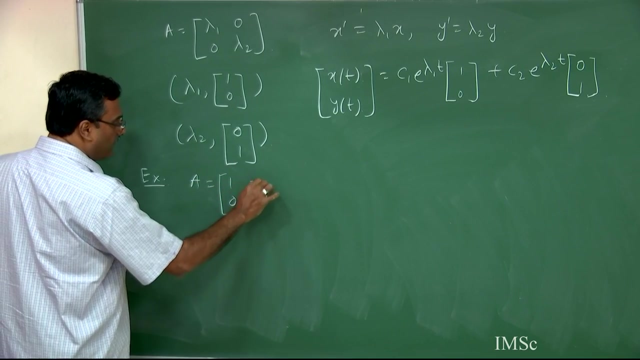 values are real and positive and, third possibility, That both the Eigen values are real and of opposite sign. So first of all, we consider a specific example, very simple example, that is, capital A. this is a matrix of the form 1, 0, 0 minus 1 right. 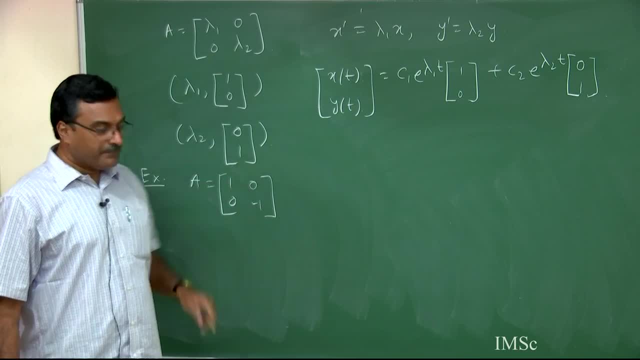 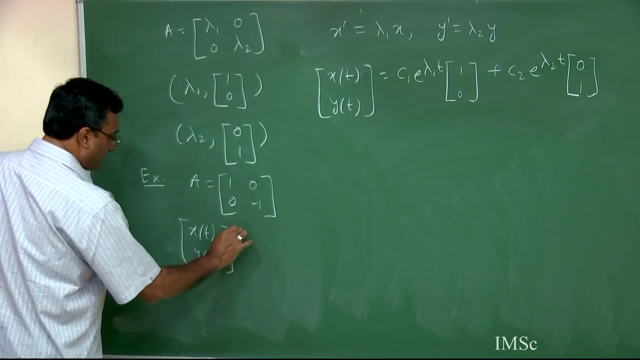 So if you follow this approach so immediately, you can write down the corresponding solution: x, t, y, t. this is equal to c 1 e to the power lambda 1 t 1 plus c 2 e to the power lambda 1 t 1 plus c 2 e to the power lambda 1 t 1 minus c 2 e to the power lambda 1 t 1 minus. 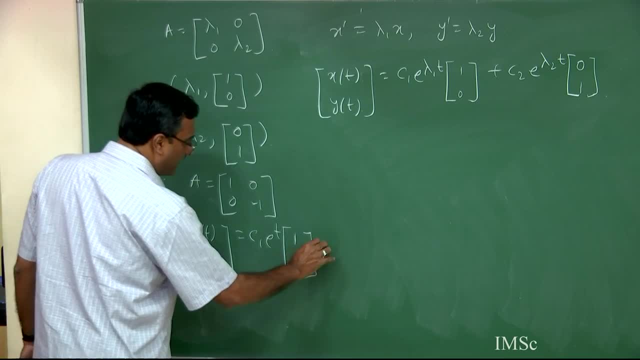 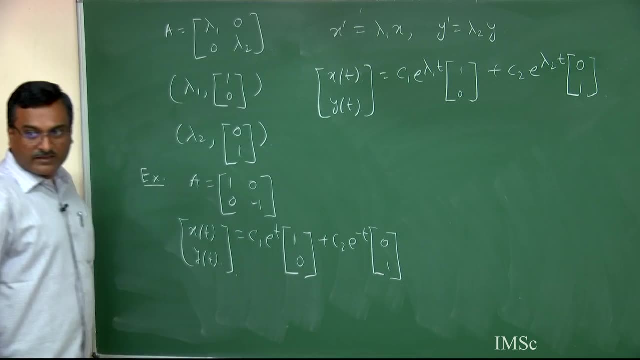 c 2. e to the power lambda 1 t 1 minus c 2. e to the power lambda 1 t2. e to the power lambda 1 T T 0, 1, E to the power t 1, 0 plus c 2. e to the power masking 0, 1 correct. 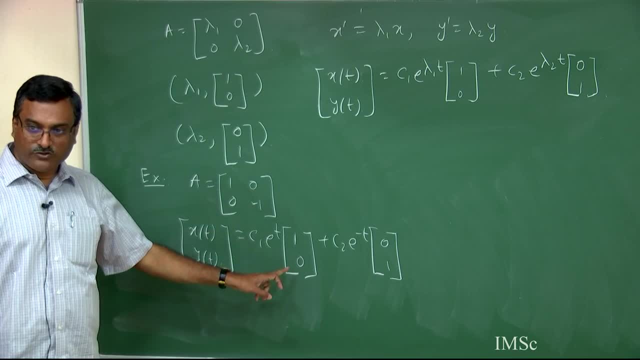 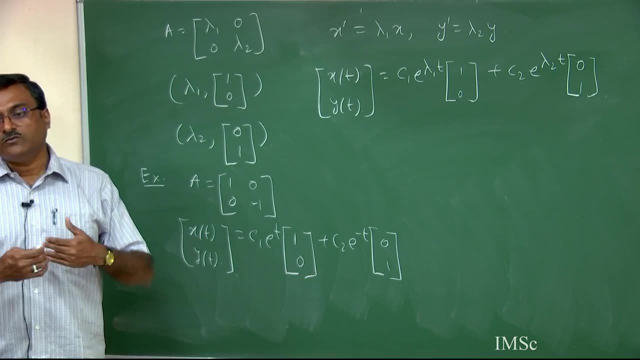 Because 1 is one Eigen value with Eigen vector one. zero minus 1 is another Eigen value with Eigen vector zero one. So this is the general solutions. Now the question is that how the solution trajectory will look like. So first of all, you try to understand. 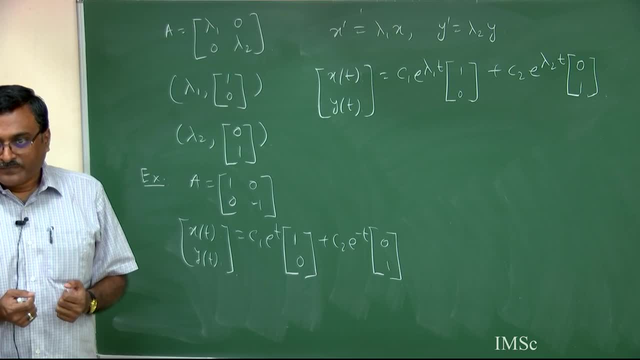 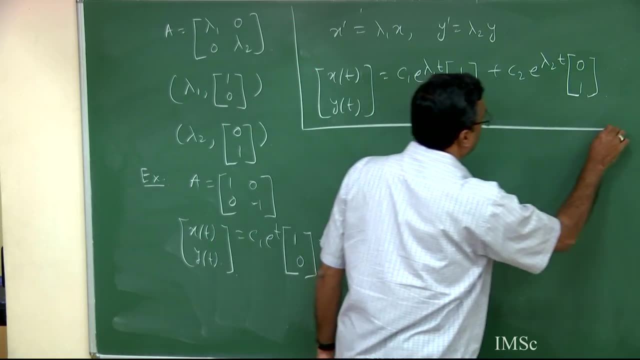 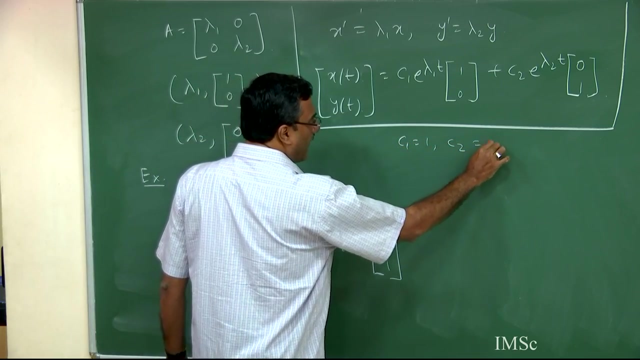 There exist two straight lines. in sampler We suppne the β, Spain, as long as x, i lambda f, x, delta of i lambda n with. so these frames line solutions. There exist two straight line solutions How we can assure that. So, first of all, from this solution we can choose C 1 equal to 1 and C 2 equal to 0.. If you consider: 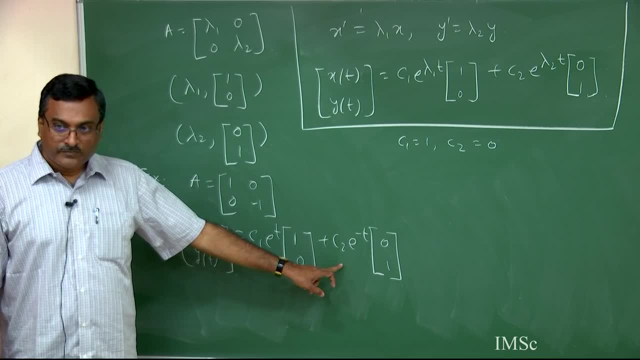 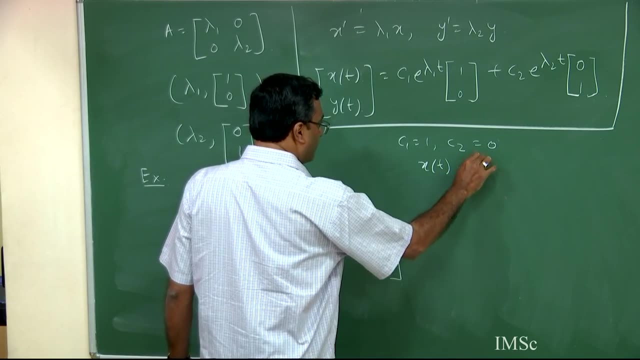 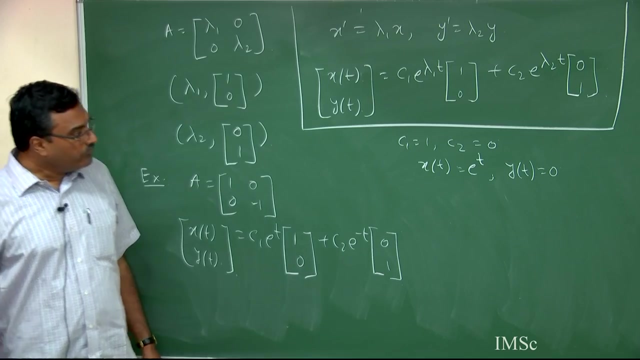 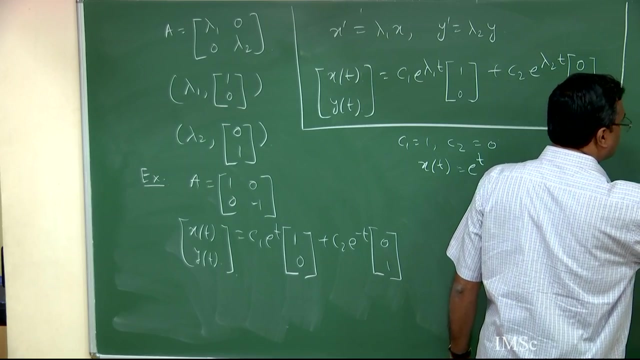 this specific values of C 1 and C 2, then what will be your solution? Your solution will be X- t- this is equal to e, to the power t, and Y t, this is equal to 0.. So the solution trajectory in x- y plane. so, if we consider, this is x axis, this is y axis, so this is: 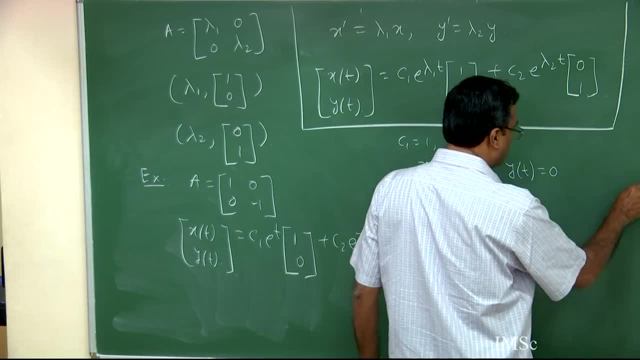 one straight line solution given by Y equal to 0.. Now, if you consider this combination C 1 and C 2 equal to 1, then what will be your solution? If you consider this combination C 1 equal to 1 and C 2 equal to 0,, then what will be your solution? If you consider this combination? 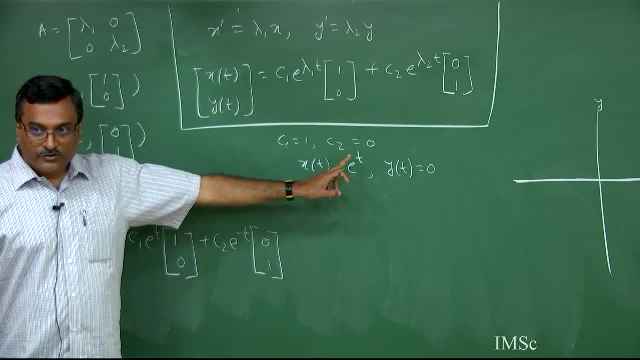 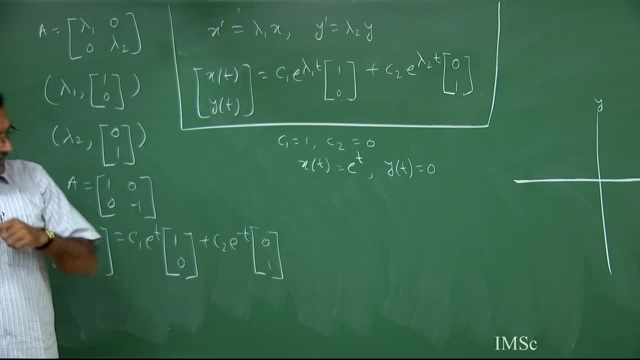 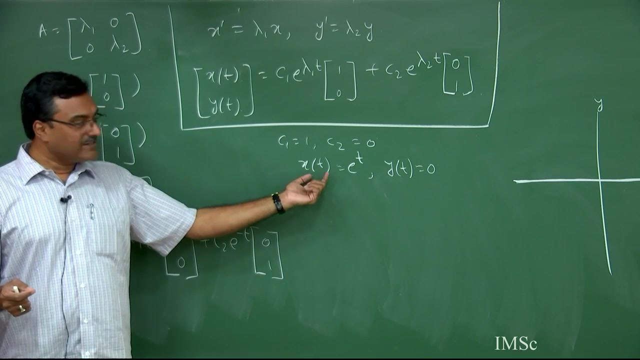 C 1 equal to 1 and C 2 equal to 0, so, along this line, what will be the movement of the trajectory with the advancement of time? You can see, the associated coefficient is e to the power t. So the advancement of time, this point X, t will be moving towards plus infinity. 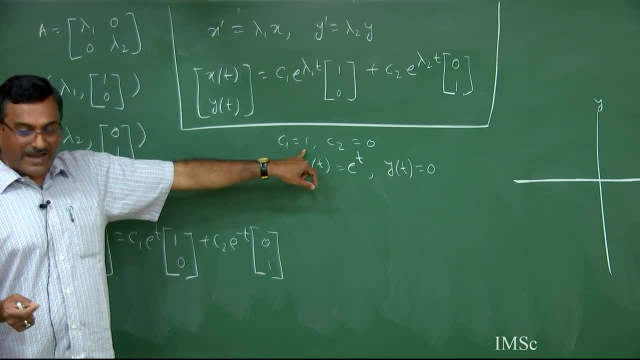 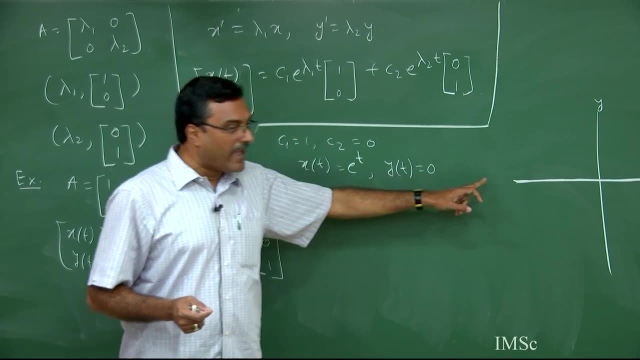 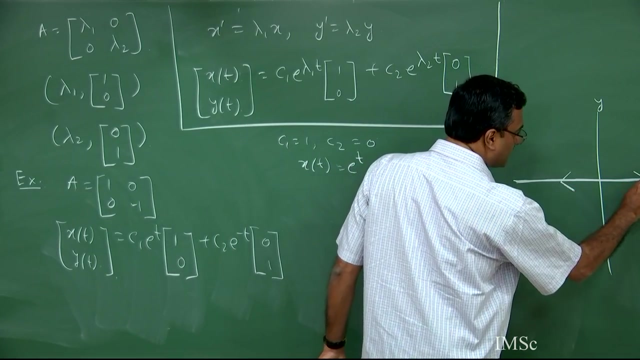 if you start with the positive initial condition and instead of 1: 0, if you choose just, for example, minus 1, 0. Then it will be starting from here and will be approaching in this direction, as t tends to infinity. So therefore, on this line, the direction of solution trajectories is this: 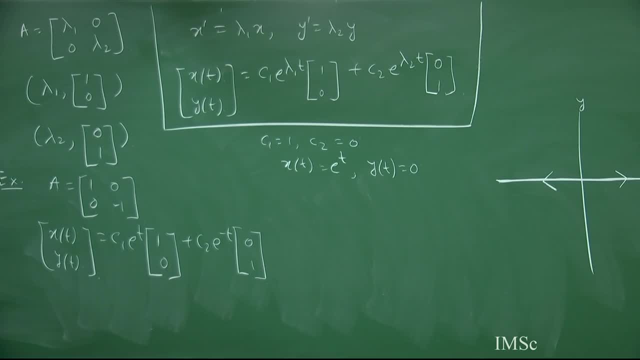 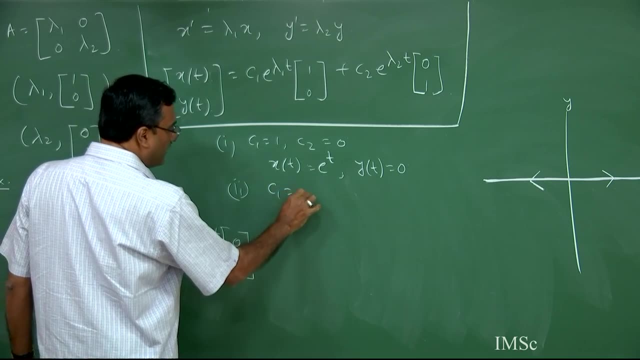 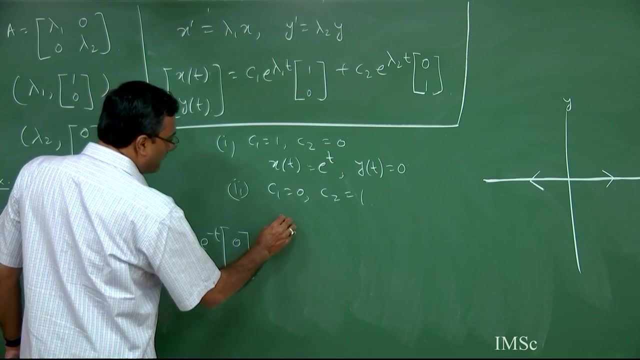 one. so that means away from the origin. Similarly, if you consider the next choice, number 2, C 1 equal to 0 and C 2 equal to 1. If you have this choice, then you can find your X t. 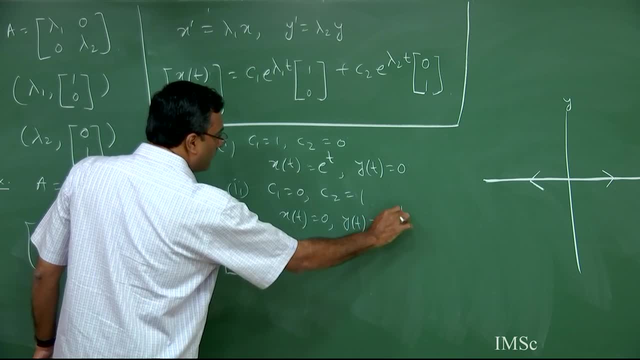 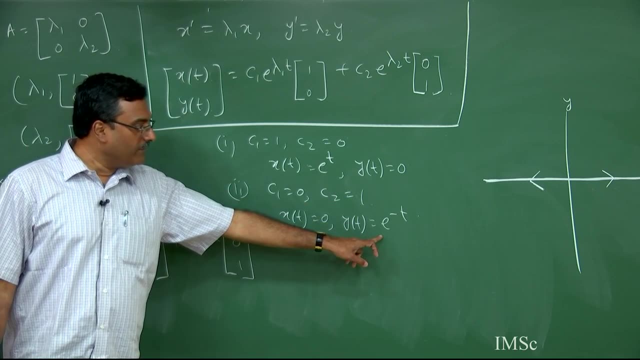 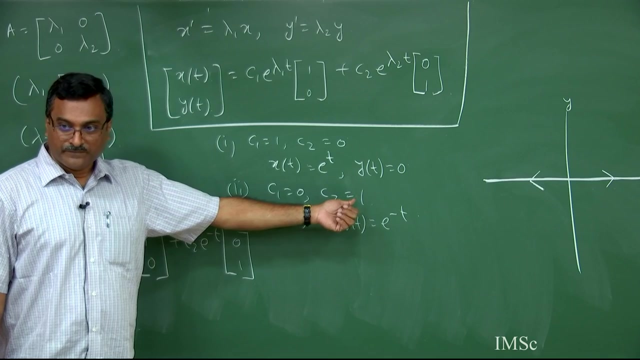 this is equal to 0, Y t equal to e to the power minus t. So again, instead of 1, if you choose minus 1, then it will be minus e to the power minus t. So, whatever may be the positive or negative choice you are having for C solution trajectory, always remain on. 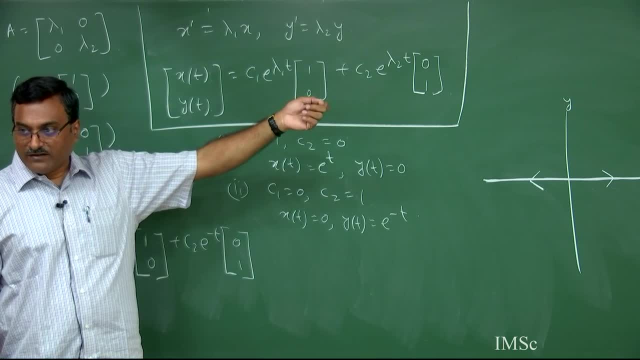 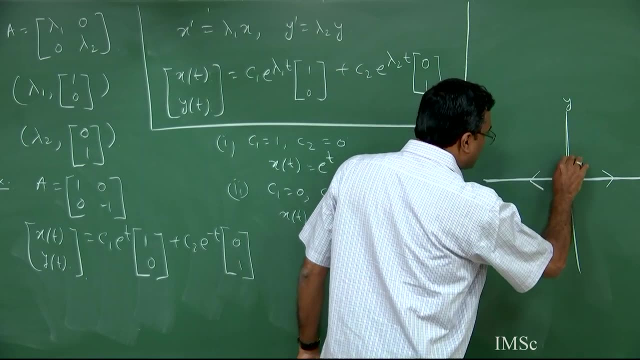 the Y axis and from wherever you start, it will be approaching towards the point 0: 0 along the vertical line. So therefore, if you consider this combination, you can see this is another straight line solution along the vertical Y axis and in this way, the trajectory. 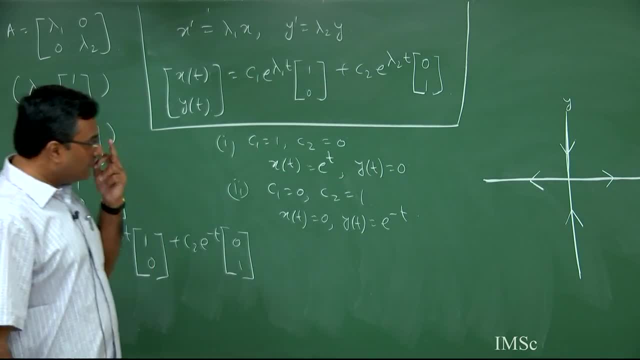 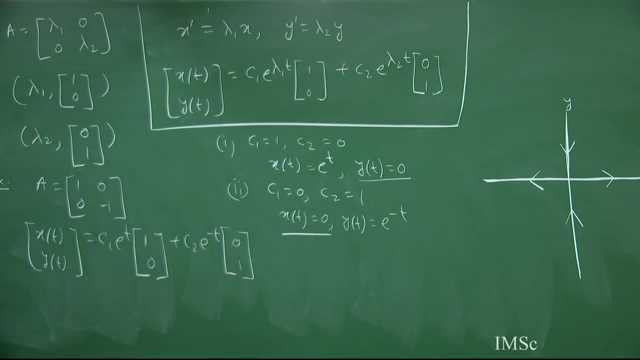 will be moving towards this direction. So these are actually two straight line solutions. one is given by Y equal to 0, another one is given by X equal to 0. Now what will be the structure of the solution trajectories for rest of the initial conditions? So in 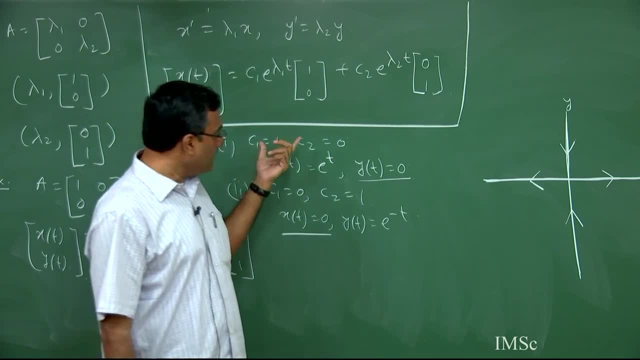 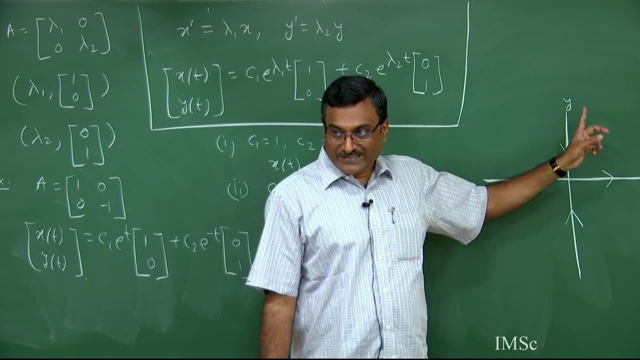 this case what you are considering here. You are choosing the positive or negative point, either on X axis or on Y axis. But if we choose any arbitrary initial condition except on the coordinate axis, then how the solution trajectories looks like I can tell. 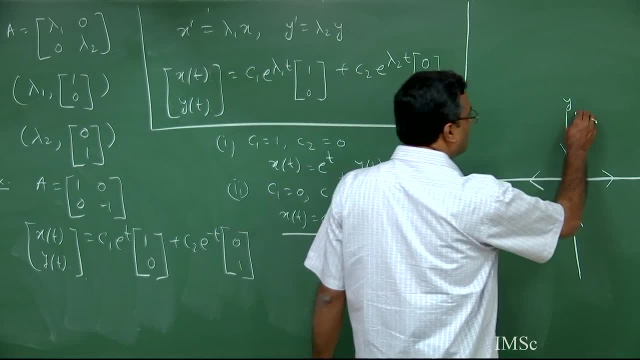 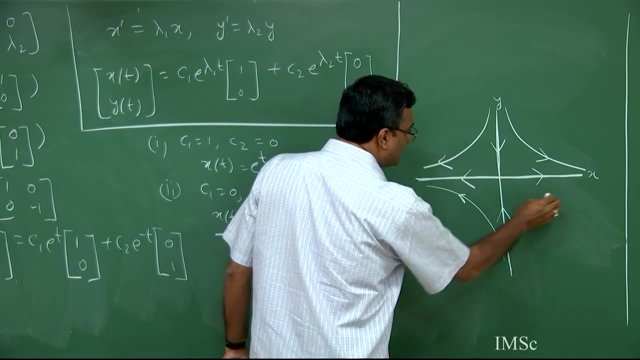 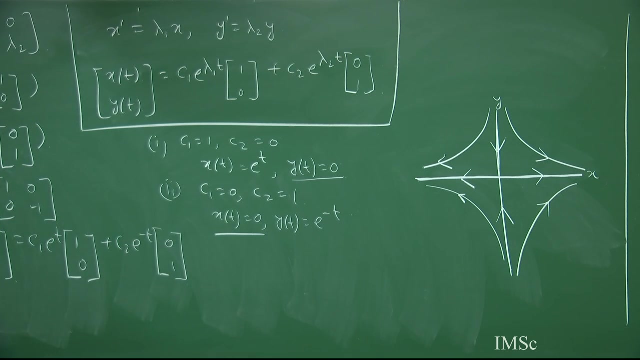 you at this point that all other solution trajectories will looks like this one, this one and this one. But the question is that: can we convince our self that, yes, this would be the possible structure? So what is the possible structure of the solution trajectories? Answer is yes, it is easily understandable. 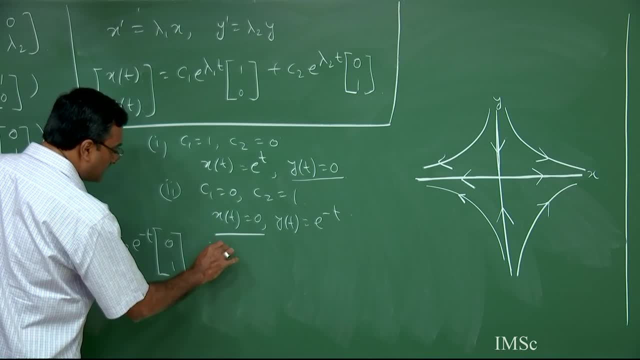 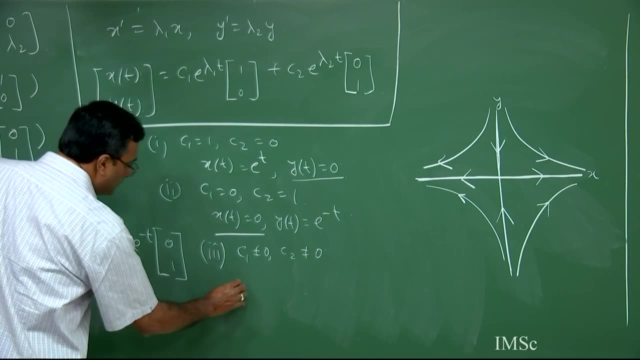 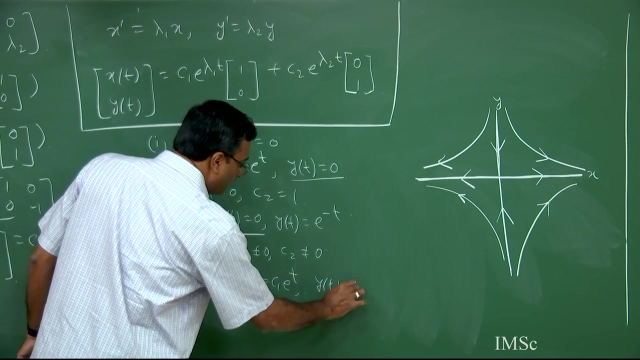 because for non-zero initial condition. so that means you are assuming your C 1 not equal to 0, C 2 not equal to 0.. So solutions are X t equal to C 1 e to the power t and Y t equal to C 2 e to the power minus t. So if you take this product, X t equal to C 1 e. 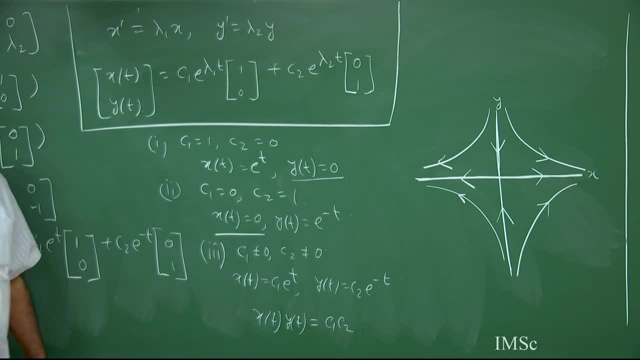 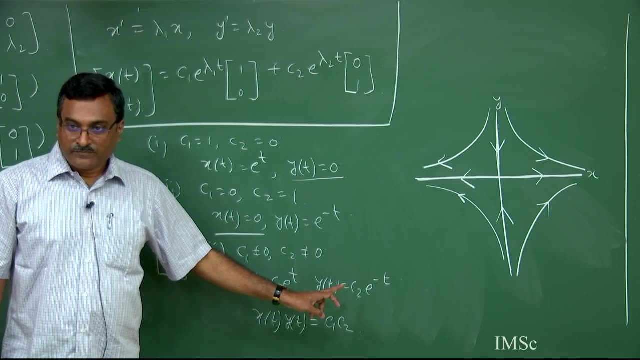 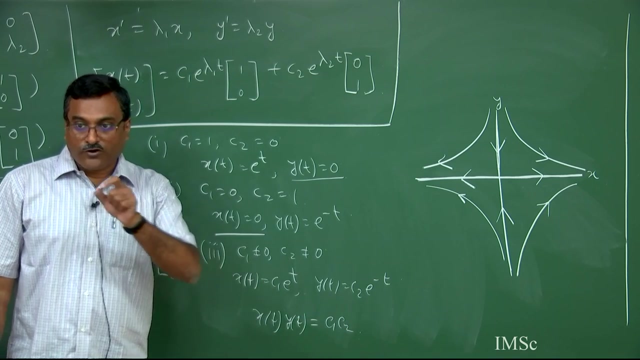 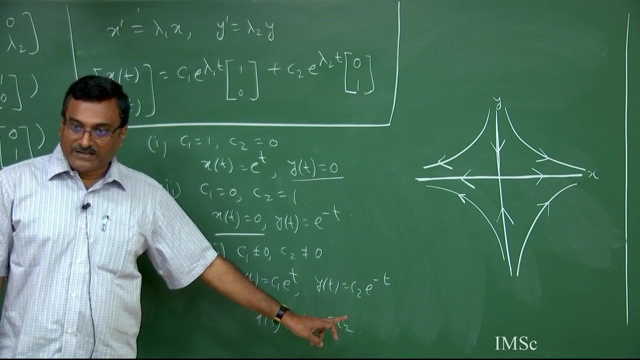 to the power t and Y, t. so this becomes C 1, C 2.. Now your C 1, C 2 are two arbitrary constants, So this product might be positive, might be negative. So for non-zero initial conditions, solution trajectories are given by X, Y equal to constant. So that means rectangular. 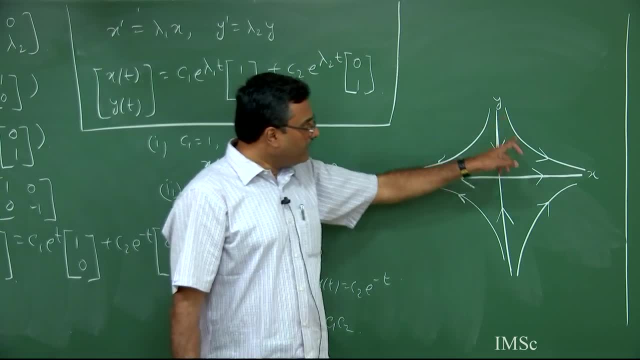 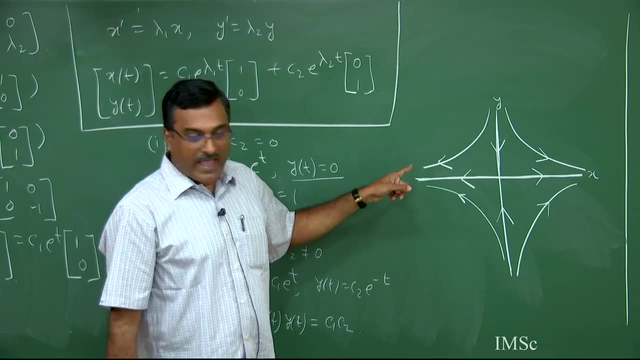 hyperbola. If this constant is positive, so therefore you will be having this constant, this branch, and if your product is negative, then you will be having this branch And these arrows can be understood just looking at either this direction or you can apply. 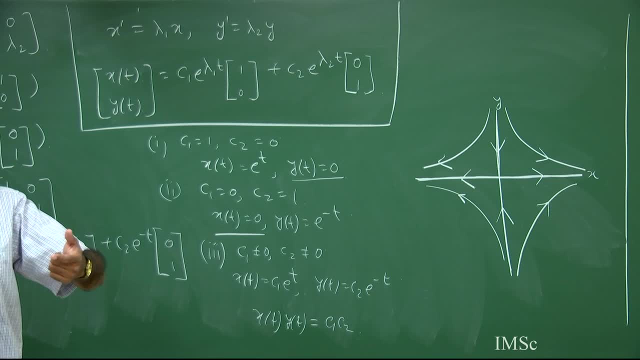 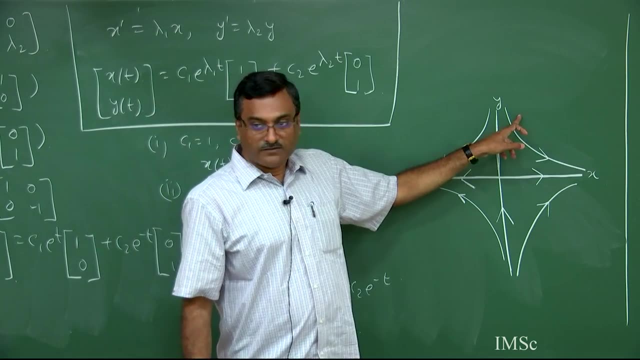 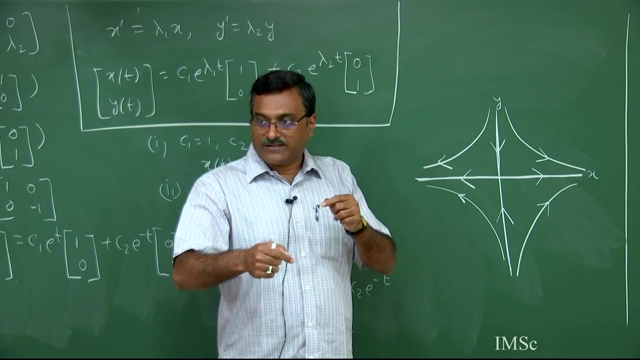 some other technique that I will be explaining in my third lecture, when I will be considering the three dimensional system, But the simplest idea is that here you can choose one point: look at the given equation, find out the direction of x and y and then look at the resulting direction. 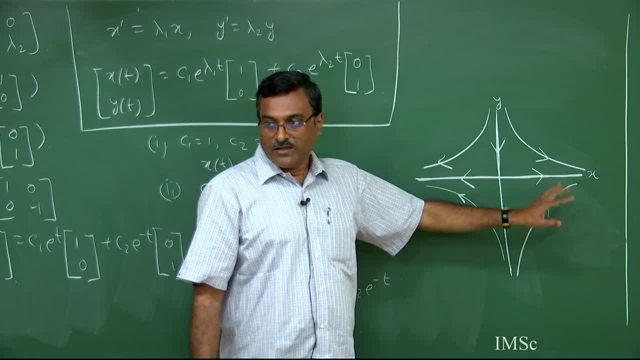 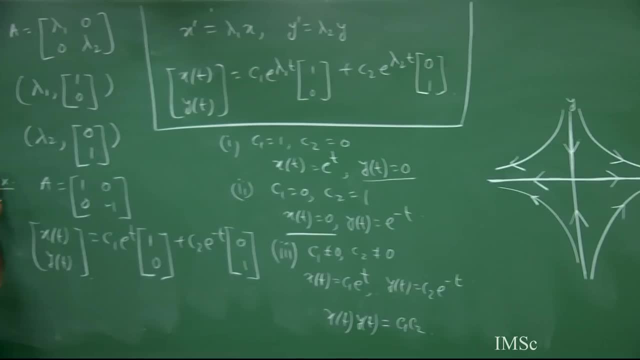 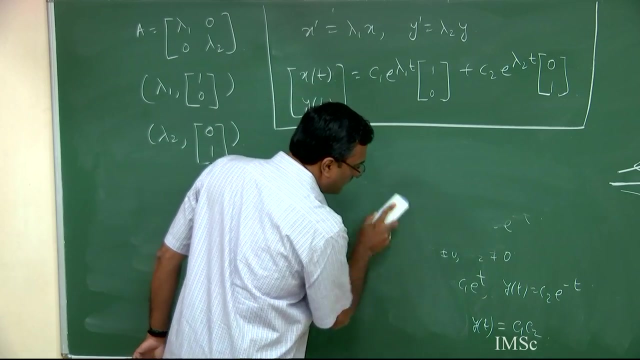 So this will give you the direction, like this one and this one. So that is called phase flow, right? So this is the example where both the eigenvalues are real, but they are of opposite sign. So next, quickly, we can consider one more example. 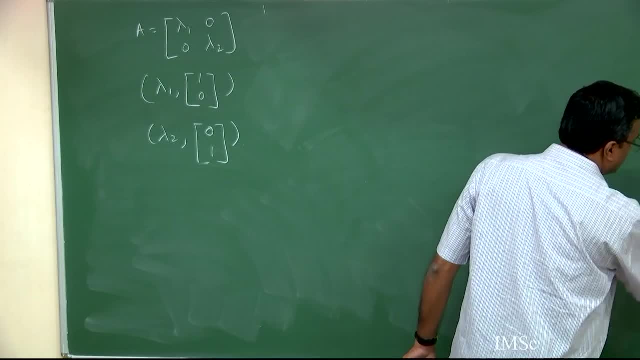 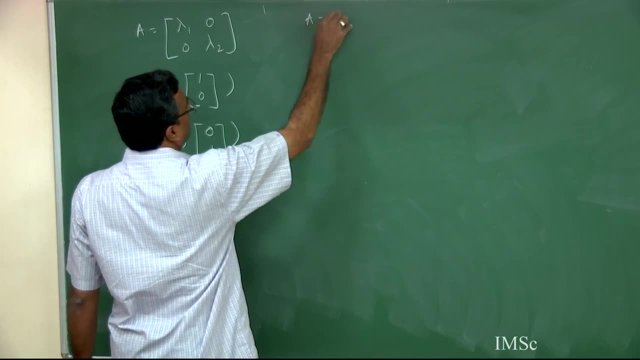 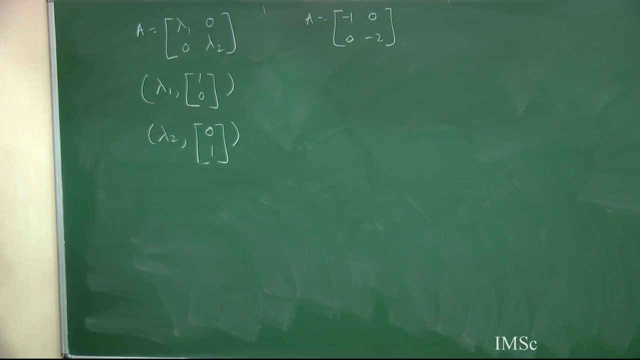 With the same, With the same format, that is, two eigenvalues are real and distinct, But just for specific reason. we can take this example: this is minus 1, 0, 0, minus 2, right? So again, you can find out eigenvalues, eigenvectors and you can write down the general solutions. 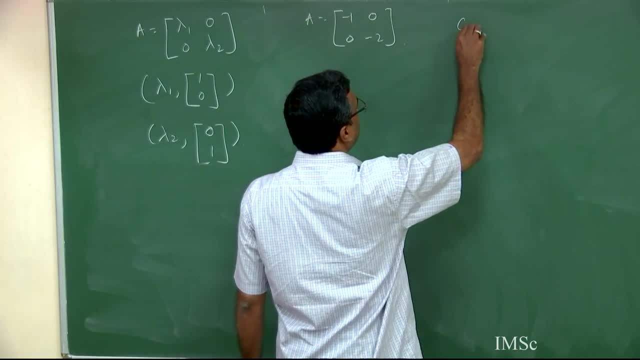 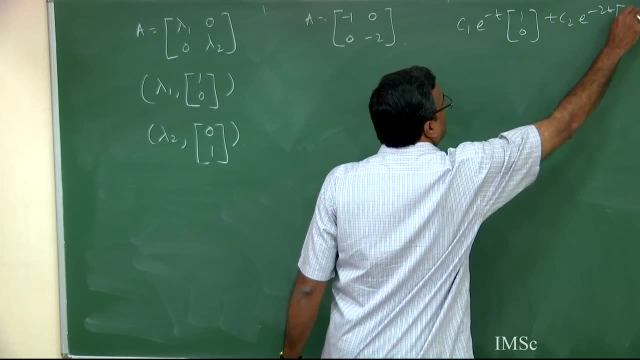 in this case. So what is the general solution? general solution will be c 1 e to the power minus t 1, 0 minus c 2 e to the power minus 2 t 0, 1, these things. So if you apply the same kind of argument, 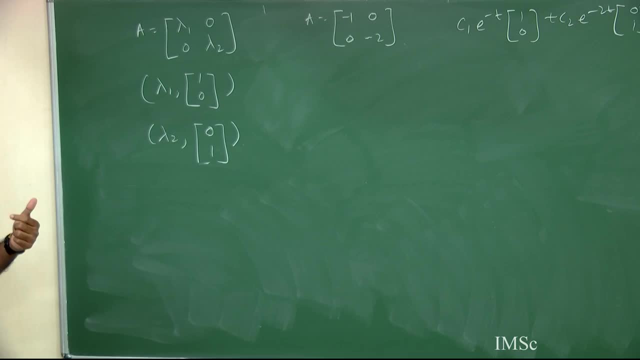 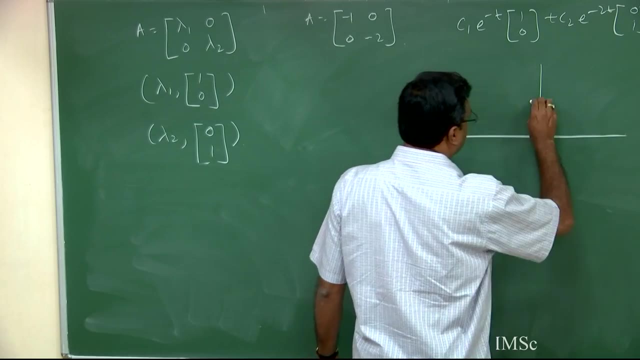 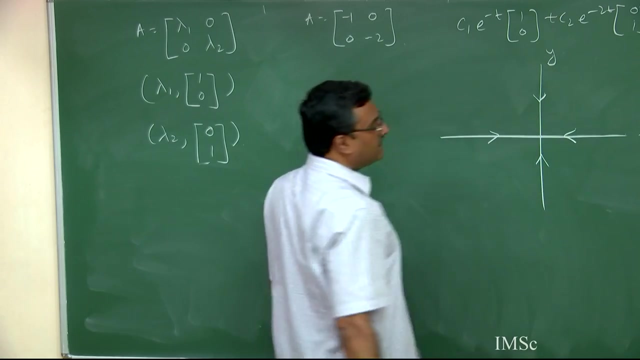 So there are two straight line solutions. one is y axis, second, one is x axis. Now, in this case, along both the axis, solutions will be approaching towards the point 0 comma 0.. This is x and this is y. right, So this is x and this is y. 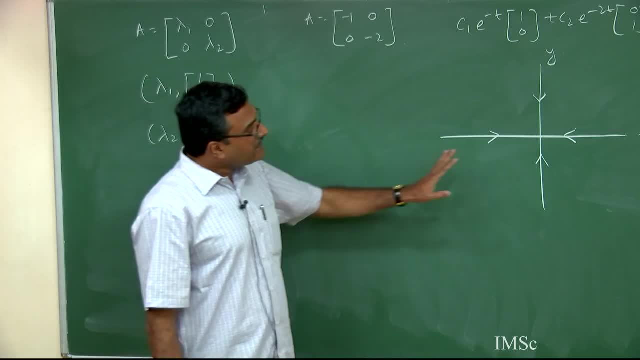 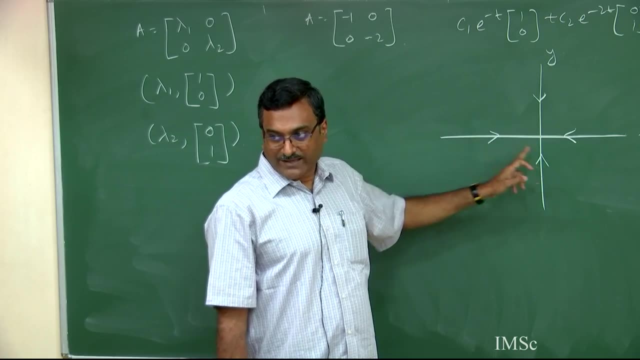 So this is x and this is y, So this is x and this is y. Now the question is that how other trajectories looks like. so that means, if we start from any point apart from the coordinate axis, So in which direction trajectories will move? 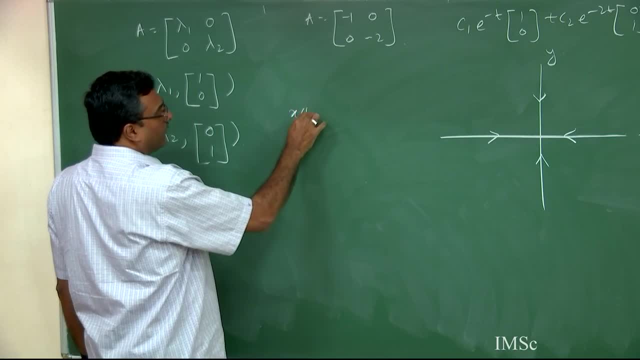 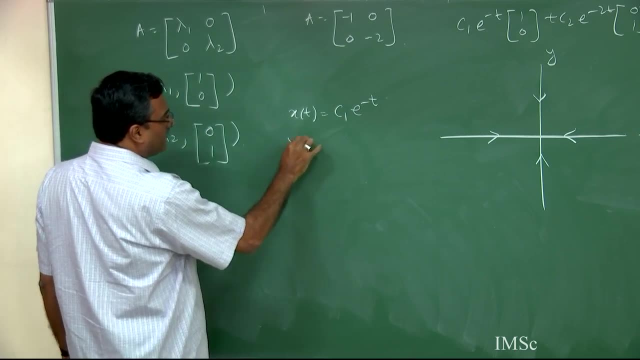 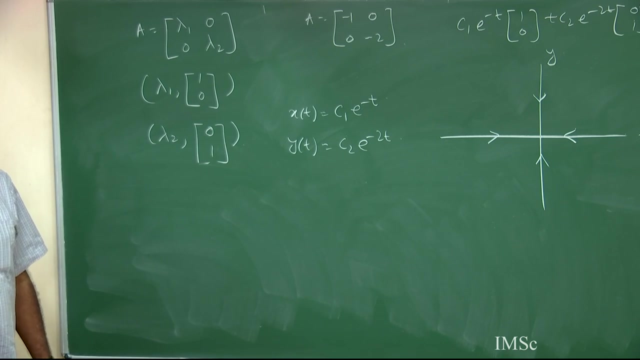 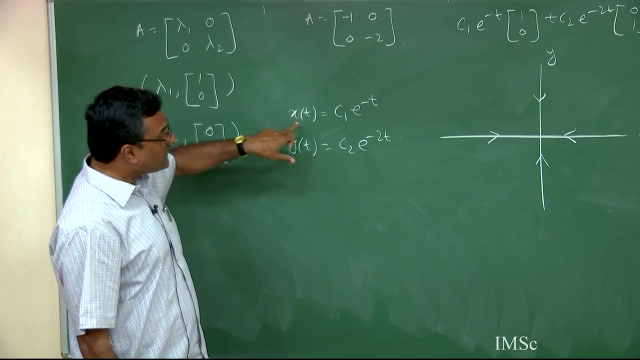 In this case, you can write down the solution as: x- t equal to c 1 e to the power minus t, and y t equal to c 2 e to the power minus 2 t. Right Now, in this case, if you square at the both side of x- t equal to c 1 e to the power minus. 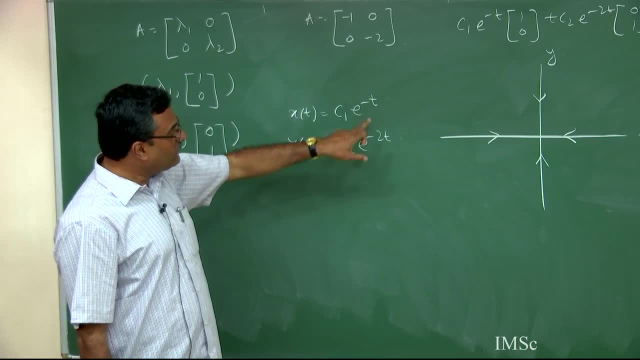 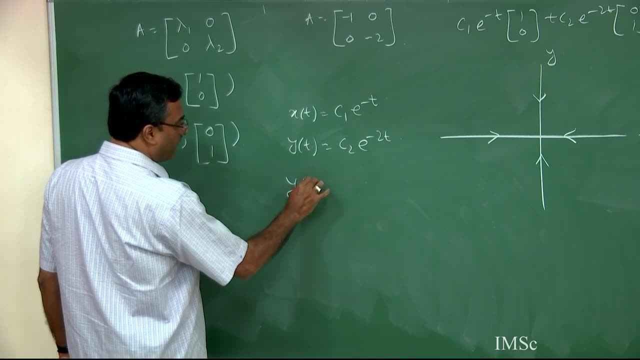 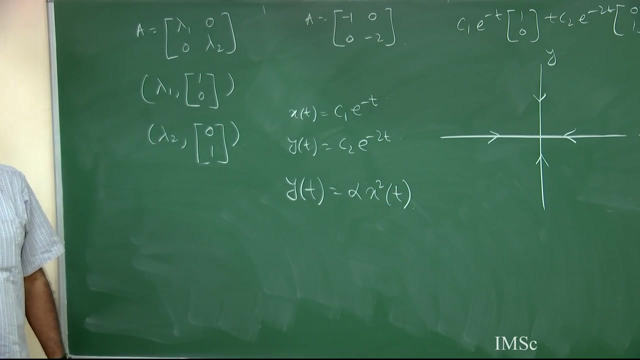 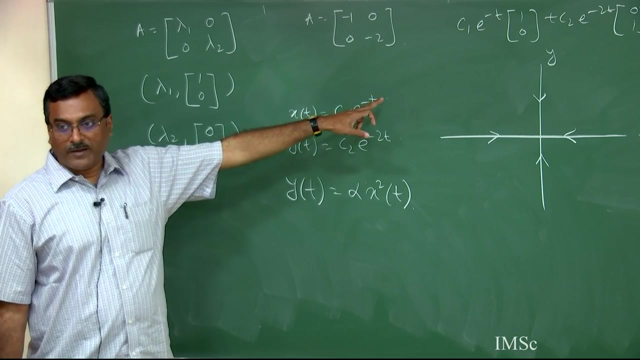 t and then eliminate e to the power minus 2 t from both the equations, Then you will be having the solutions in the form: y, t is equal to some alpha times x square t. Correct, Because x, t by c, 1 whole square equal to e to the power minus 2 t. 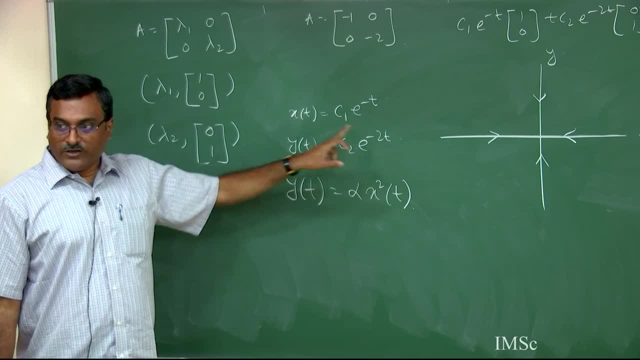 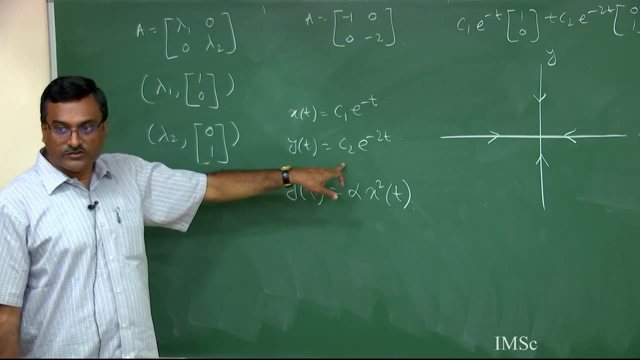 y, t by c 2, equal to e, to the power minus 2 t. So, equating, you will be having x square by y, that is equal to constant. Here we are assuming c 1 and c 2 are both non-zero, right. 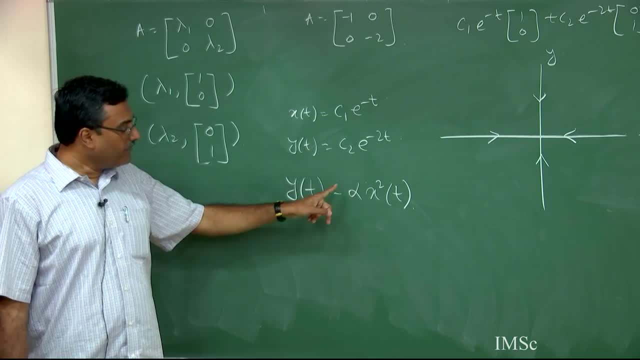 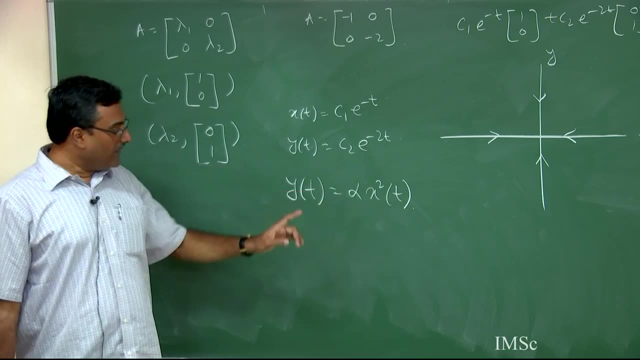 And as c 1, c 2 are arbitrary quantity, so therefore it might be positive, might be negative, depending upon whether your c 2 is positive or not, Right? So if this is the general format of the solution trajectories for the given system, 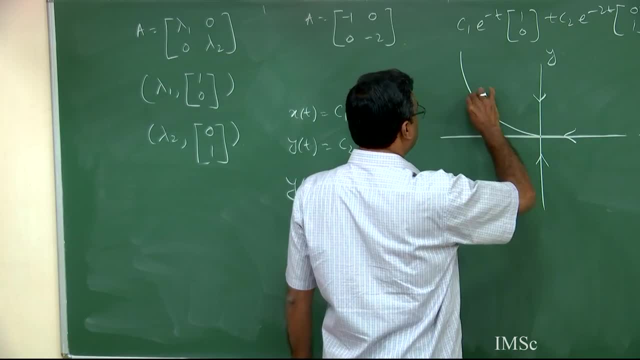 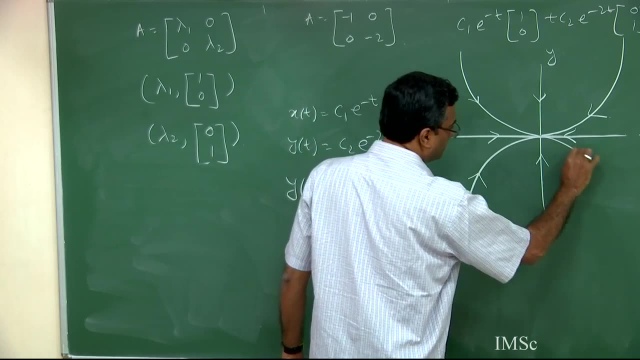 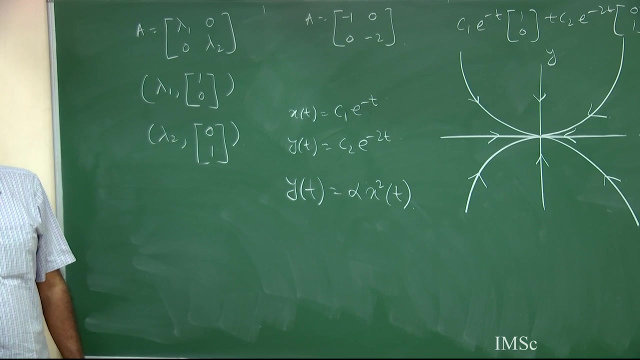 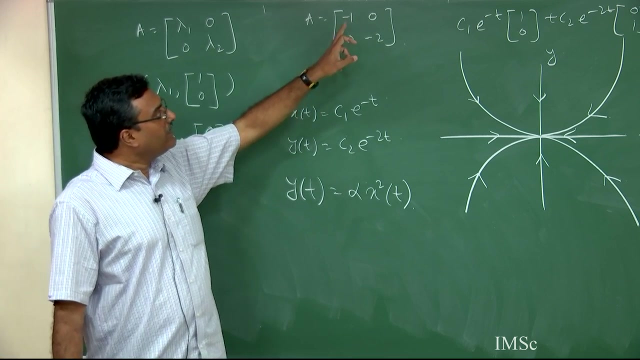 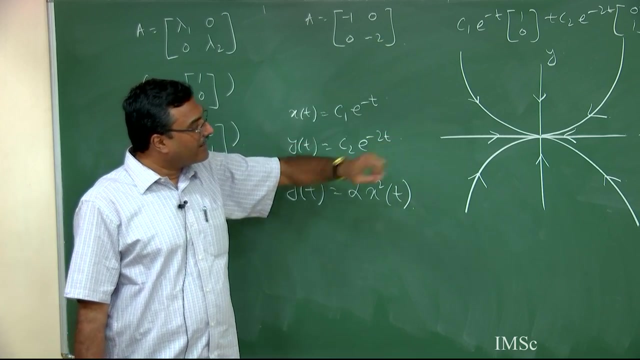 So, therefore, other solution trajectories, except the solutions on coordinate axis. they looks like this one, right? So this is the phase portrait, and you can similarly consider the other possibilities. That means this is, say, minus 3, this is minus 1.. So in that case, what will be the change in the diagram? 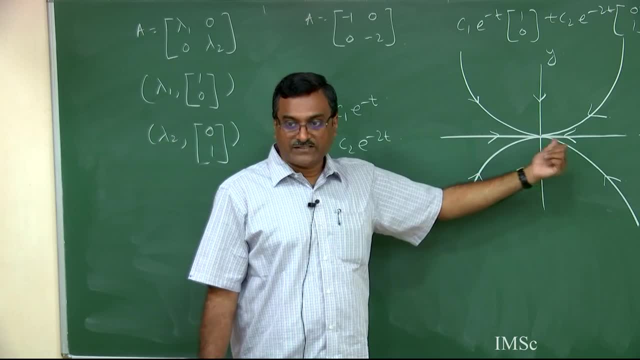 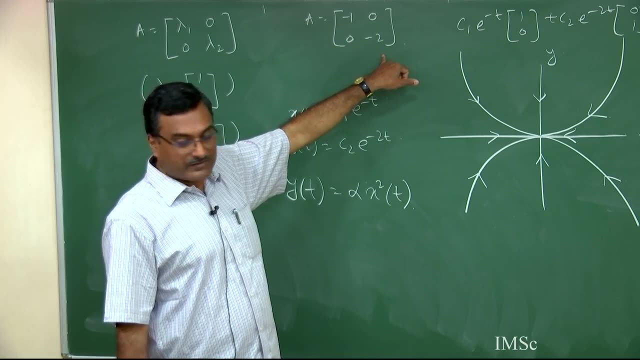 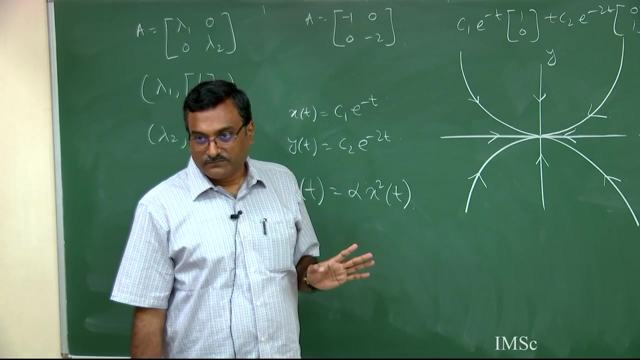 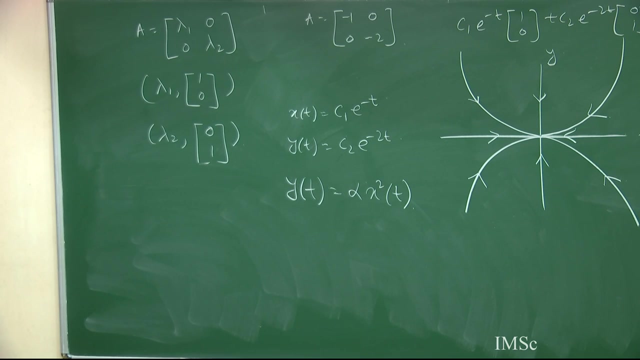 So here all the trajectories are having x axis as its tangent. But in case the magnitude of first eigen value is larger than the second one, then vertical y axis will be tangential to the all solution trajectories near origin Right. So this is the structure of solution in case of two distinct eigen values. 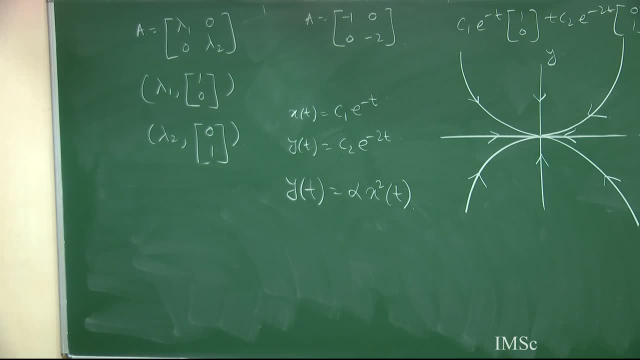 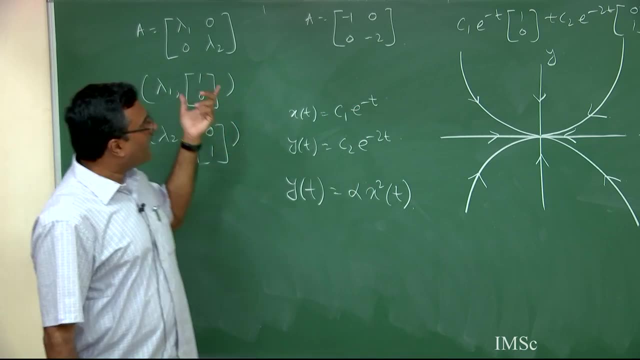 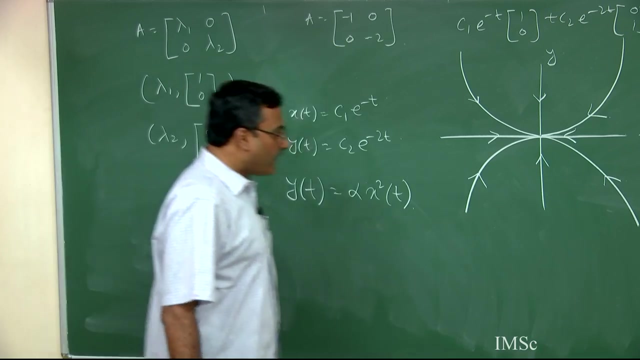 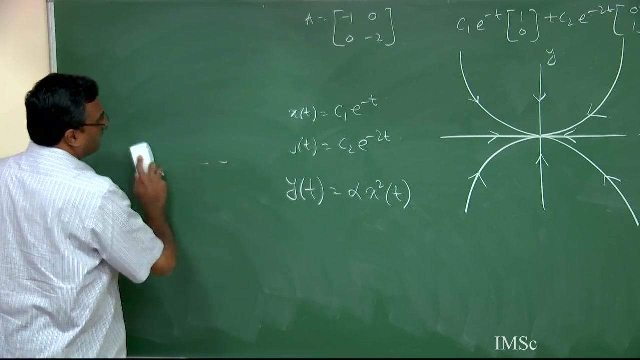 Now the point is that I have already explained that this kind of system can be derived from the given equation in case you have two real distinct eigen values. So now I can show you that how this result can be utilized. Ok, understand the nature of the solution trajectories in general system which are not in the Jordan. 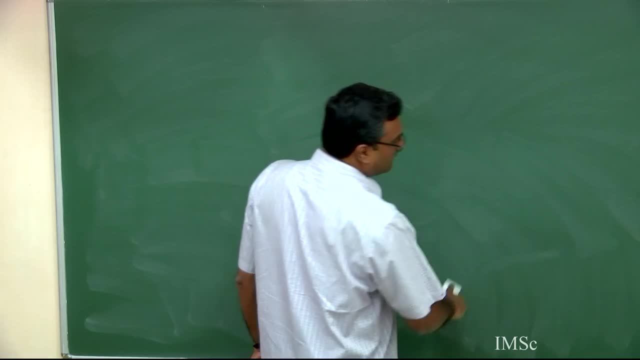 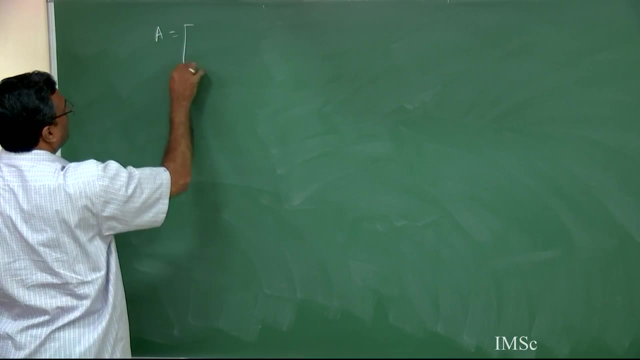 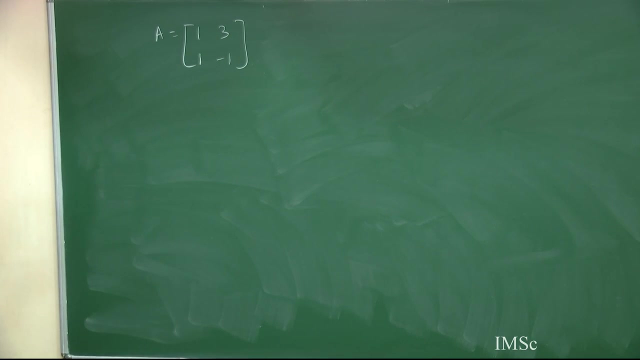 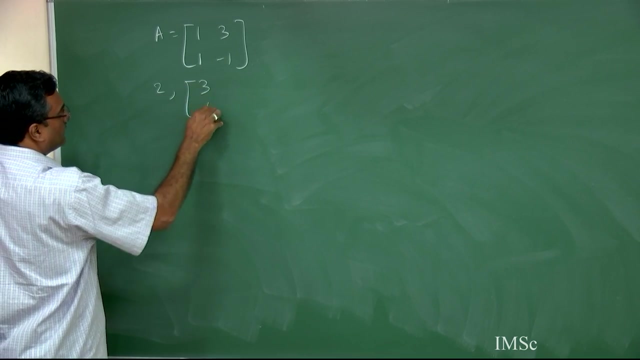 canonical form. In order to explain this result, I can go back to the first example, where we have considered A equal to 1, 3, 1 minus 1.. This was our capital A. So for this problem, we have obtained this Eigen pairs, that is, 2, with Eigen vector 3, 1.. This is Eigen value. 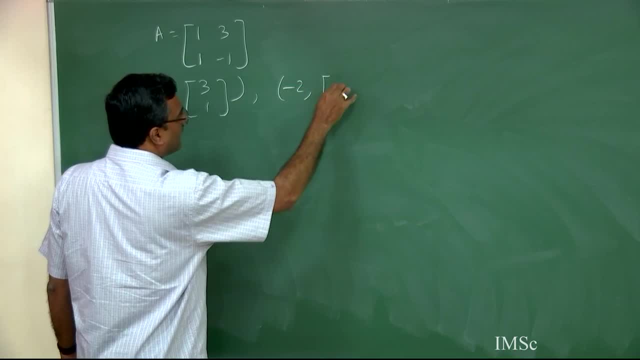 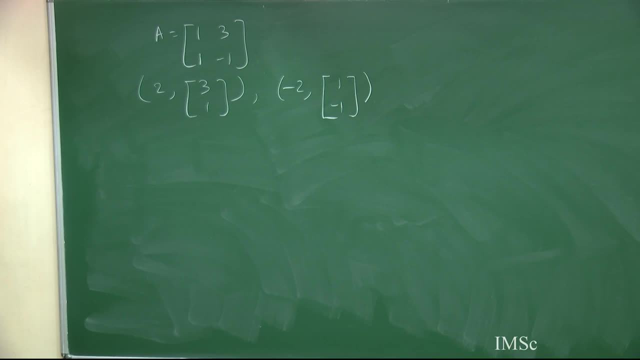 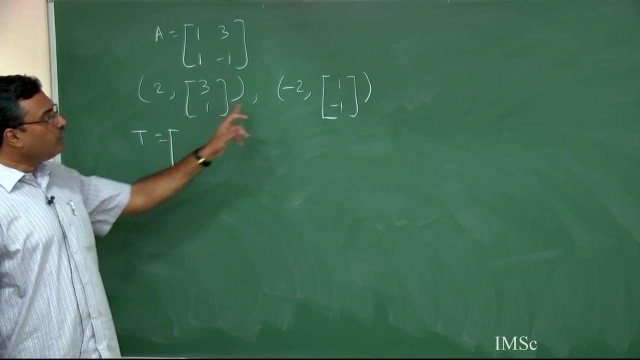 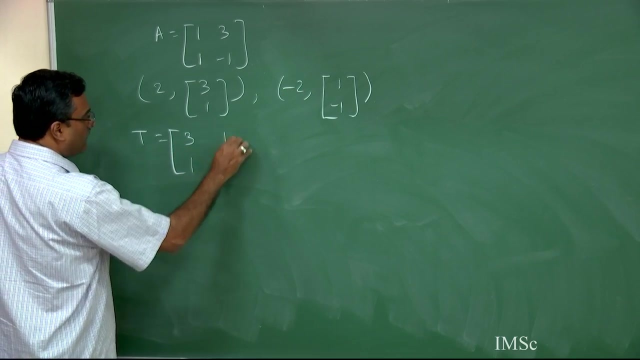 corresponding Eigen vector and another Eigen value. Eigen vectors are given by this one minus 2, 1 minus 1.. So now I can construct a matrix, capital T, consisting with these two Eigen vectors as its components. So therefore the matrix T is given by 3, 1 1 minus 1.. It is a 2 cross 2 matrix. Therefore, 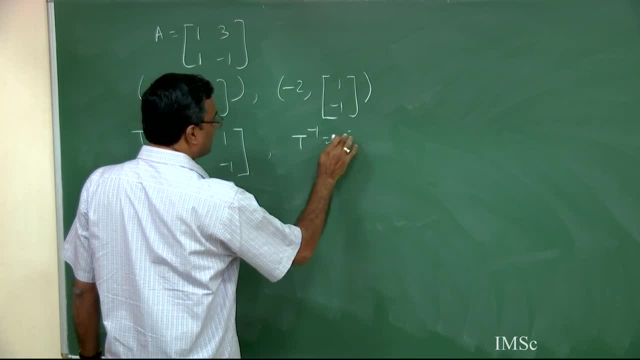 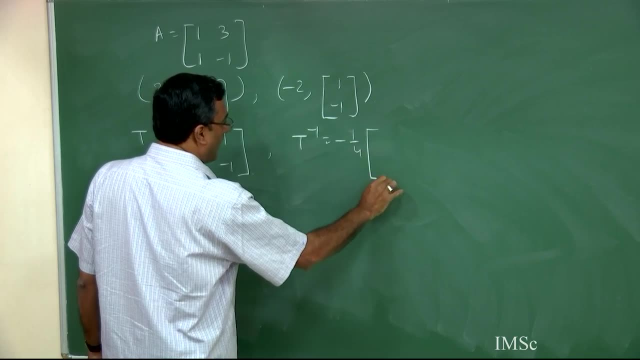 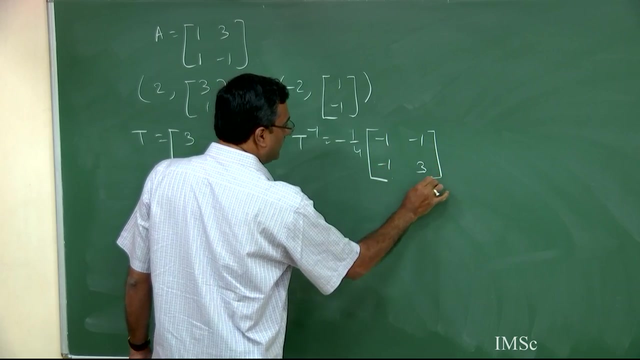 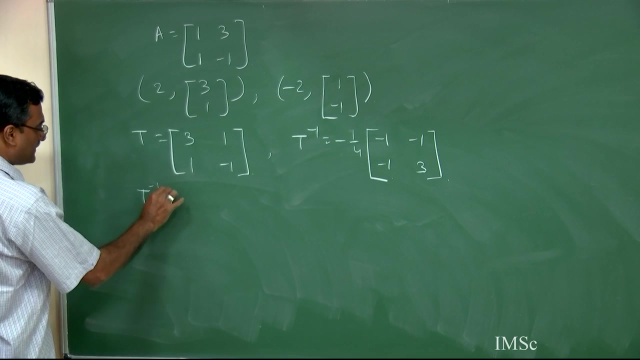 you can calculate easily: T inverse- This is going to be determinant- is minus 4.. So, therefore, minus 1 by 4, and then these two element will be interchanged and for these two element sign will be changed. Now the idea is that if we calculate T inverse, A T- this is the standard technique for deriving 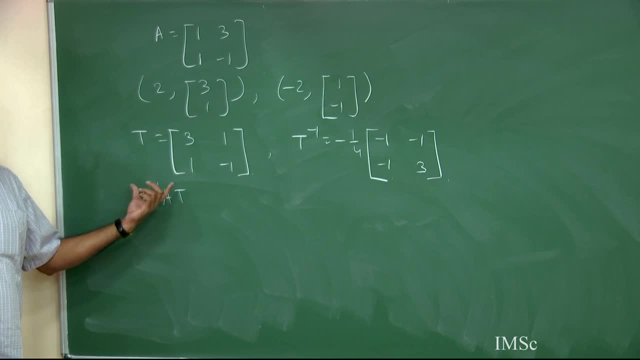 Jordan canonical form. I am just giving you the explanation through an example, not going into the details, such that you can have certain essence that how to do it Next. you can apply these things for higher dimensional system as well as for the cases with repeated Eigen. 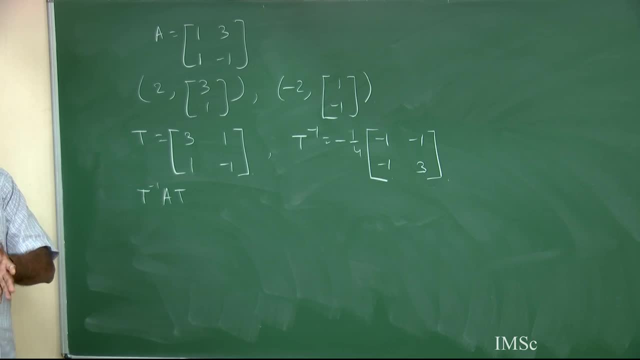 value as well as complex Eigen values, or larger matrix consisting with both real Eigen values, complex Eigen values and so on, and at the end I will be giving you a reference where you can see all these details. So now we are interested to calculate this T inverse A T. So first of all, if you calculate, 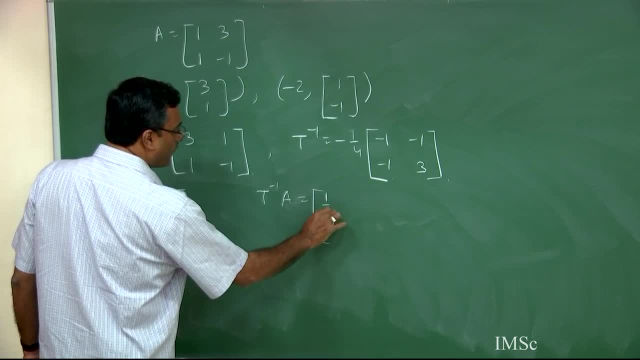 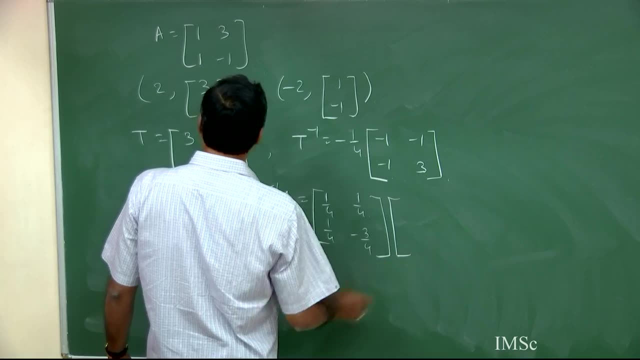 T inverse A. So this is nothing but 1 by 4, 1 by 4, 1 by 4 minus 3 by 4.. This multiplied with this matrix: 1, 3, 1 minus 1.. So this will be equal to this is 1 by 4, 1 by 4.. If we get, 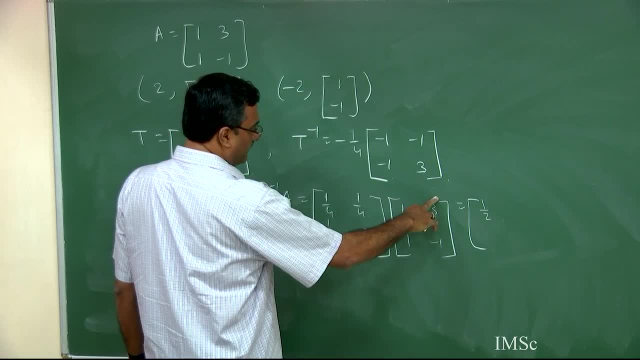 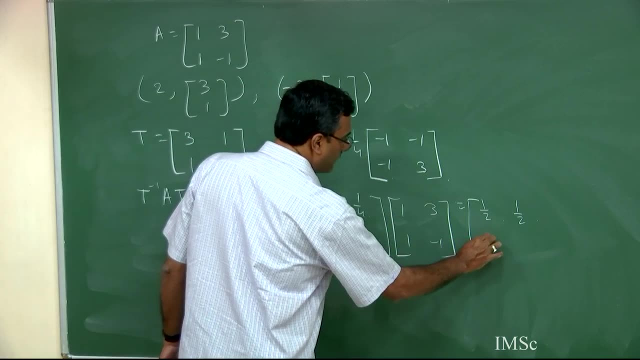 by 4.. So this is equal to half, then 3 by 4 minus 1 by 4.. So this is equal to half, then 1 by 4 minus 3 by 4.. So this is equal to minus half. and finally, 3 by 4 plus 3 by. 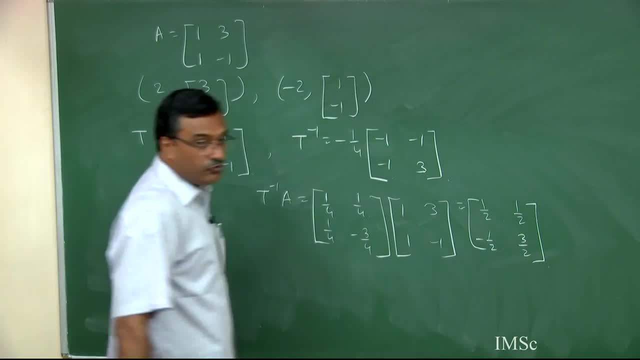 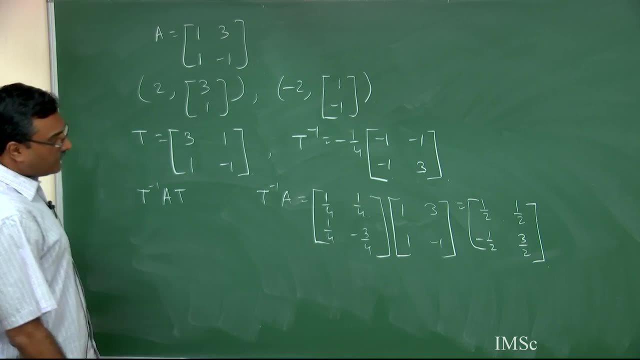 4.. So this is equal to 3 by 2, right? this is T inverse A. Now, if you calculate, now if you calculate T inverse A T, So this is equal to half half minus half 3 by 2, this multiplied with this, multiplied with 3: 1, this matrix: T: 3, 1, 1 minus. 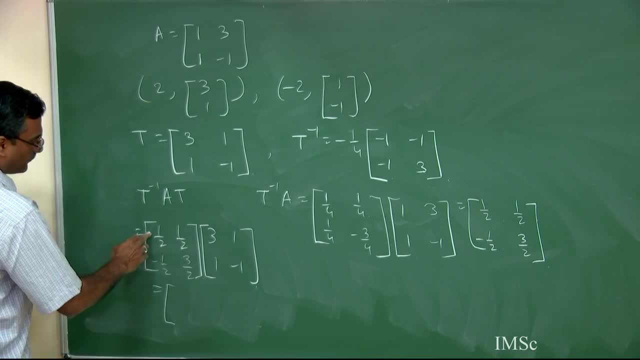 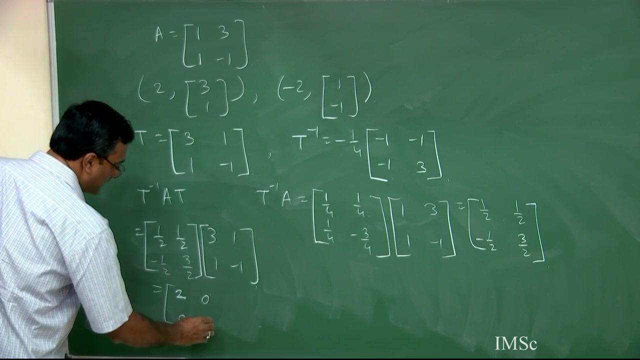 1. So, therefore, this will be equal to 3 by 2 plus half. So this is 2, this is half minus half, 0, this is minus 3 by 2 plus 3 by 2: 0, this one, and this is going to be minus half, minus 3 by. 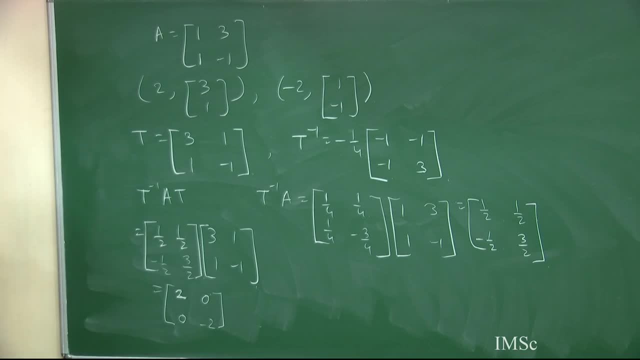 2. So this is equal to minus 2 right Now, the next question is that I have this: given matrix A associated system, is x dot equal to A x, So how this matrix can be utilized in order to understand the solution of the original system. The idea is that your given. 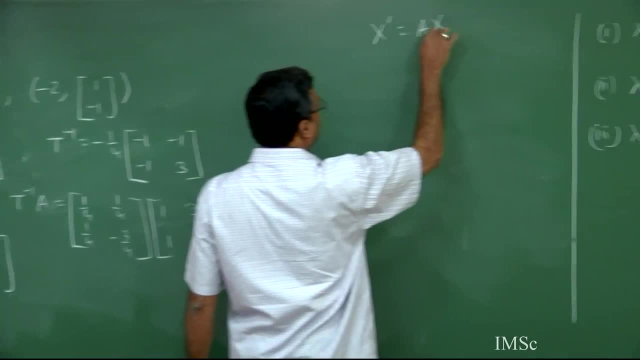 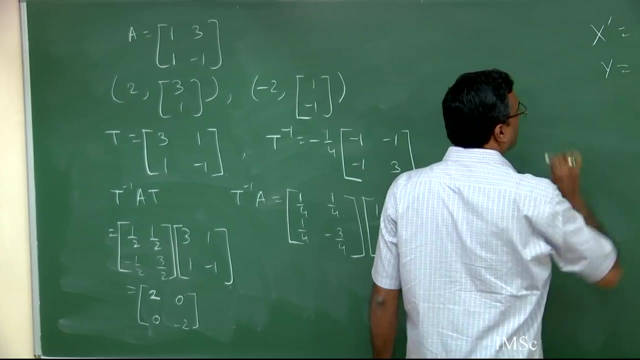 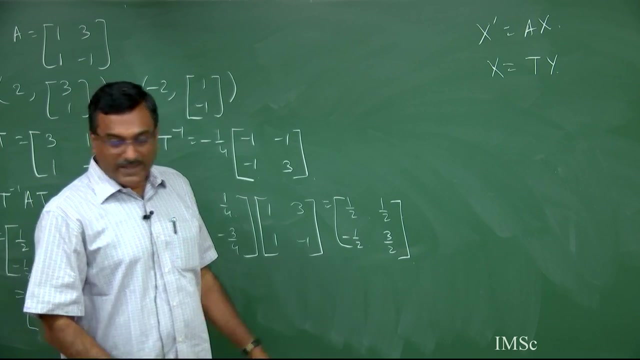 system is x, dot is equal to A, x. You have defined the matrix T here, So you can use a transformation x equal to T, y. you use this matrix transformation, So X is X, T, Y, T, so you can consider capital Y as. 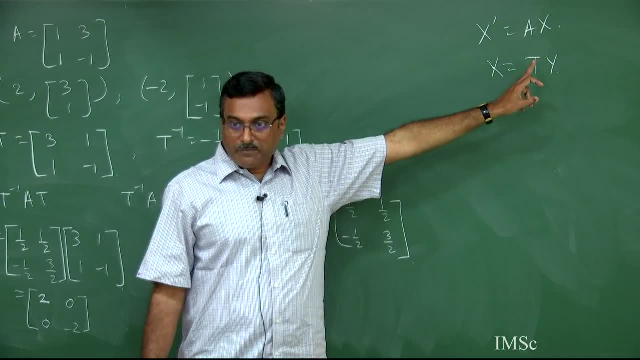 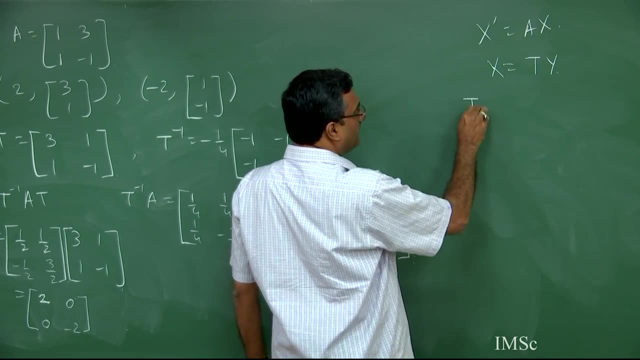 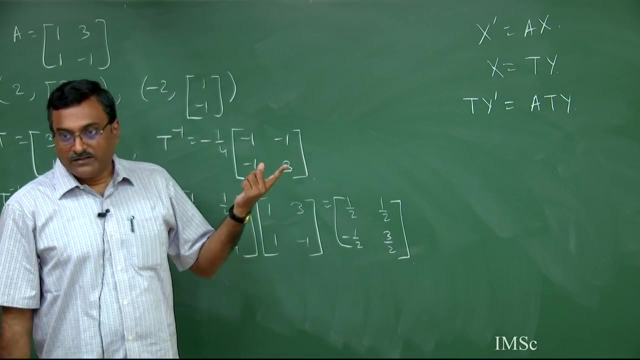 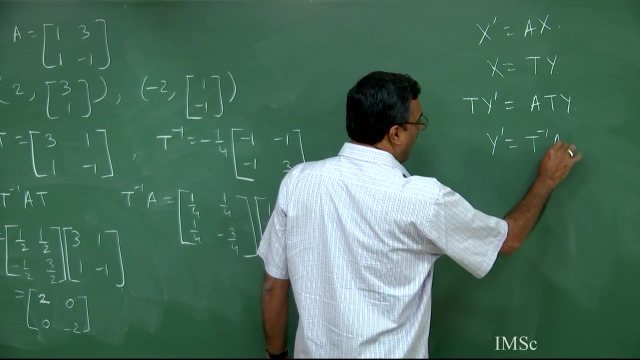 say Y 1, T, Y 2, T, but in terms of matrix notation, if we substitute this X equal to T Y in this equation. so therefore you will be having T Y dot that is equal to A T Y. so X is replaced by T Y right. So therefore, in terms of transformed variable, you will be having this matrix T. 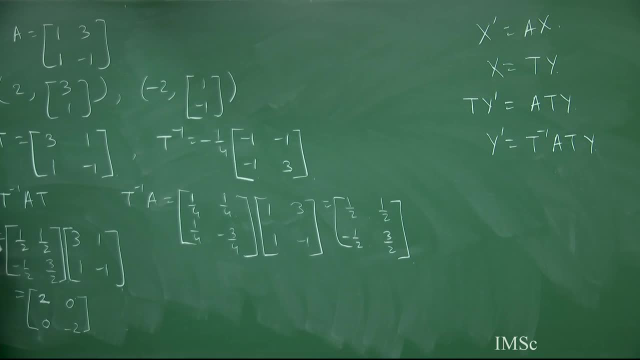 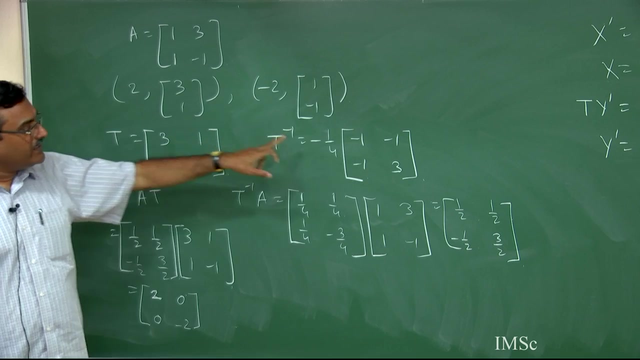 inverse A, T, Y. Now I forgot to mention one thing: that in case of A having two real, distinct Eigen values, so therefore Eigen vectors are linearly independent to each other. So in this way, if you construct the matrix T, so this matrix T is always invertible, right? So once you have this invertible matrix, 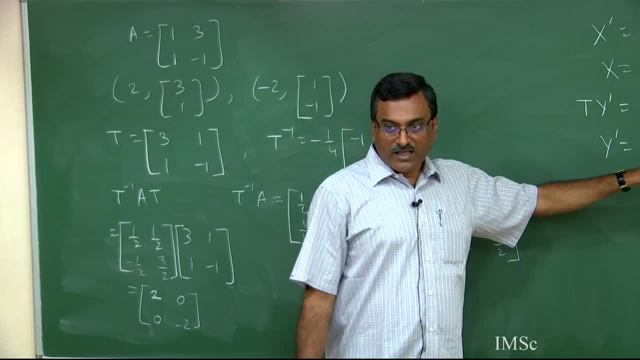 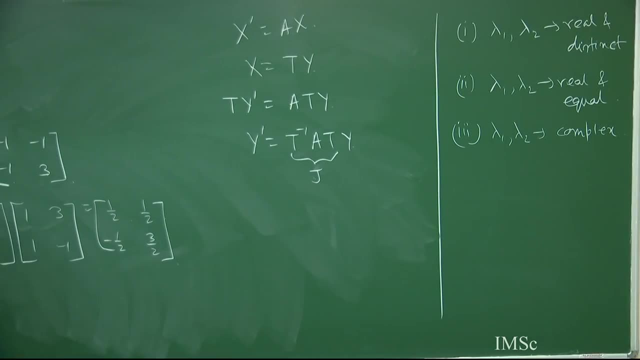 so you can have this particular structure and then you can call this matrix as say, J, which is the corresponding Jordan Canonical form. So once you have the solution trajectory for this transform system, that is, Y dot equal to J, Y, which is very much clear, and then, if you use the inverse transformation, that 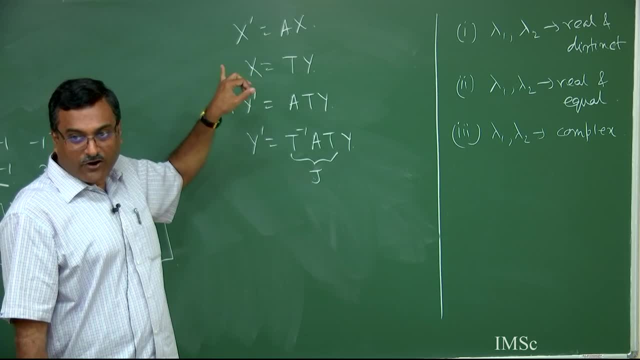 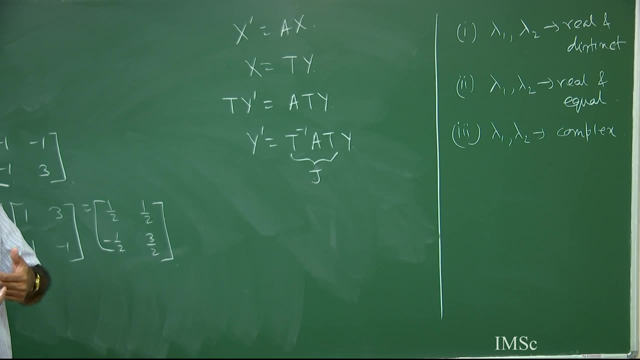 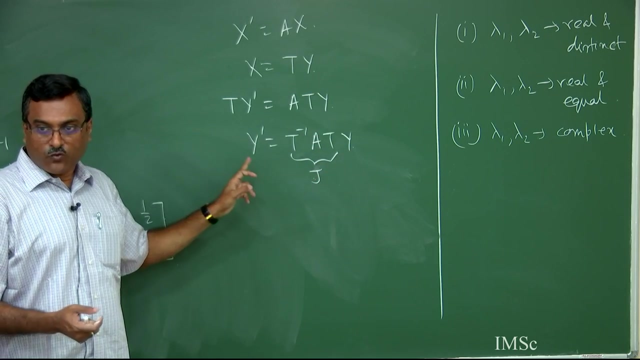 is Y equal to T inverse X. so accordingly, you will be having solution for the original system as well as you can understand how the phase portraits will looks like. Now you know that structure of the phase portrait for this system: y dot equal to j. y. now under. 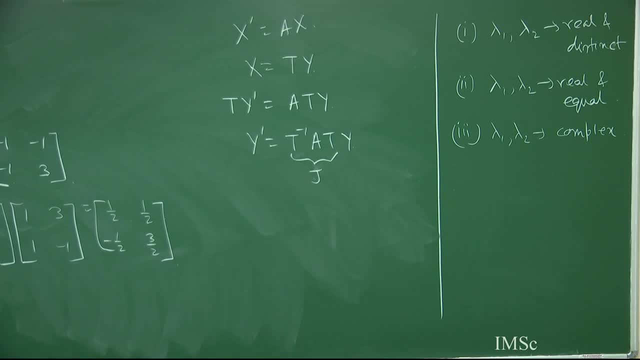 transformation how the phase portraits will looks like for the original system. So then you can recall that for original system these are the Eigen pairs. So therefore general solution is given by X, t. this is equal to C 1, e to the power 2. 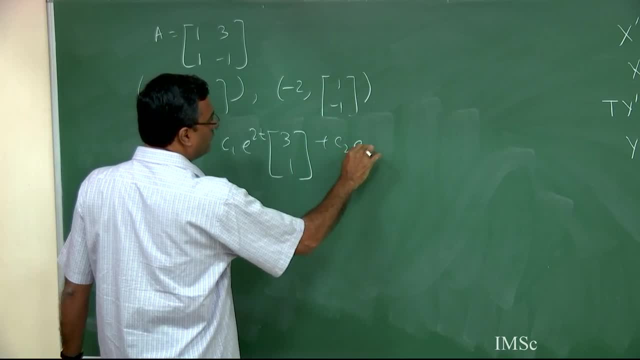 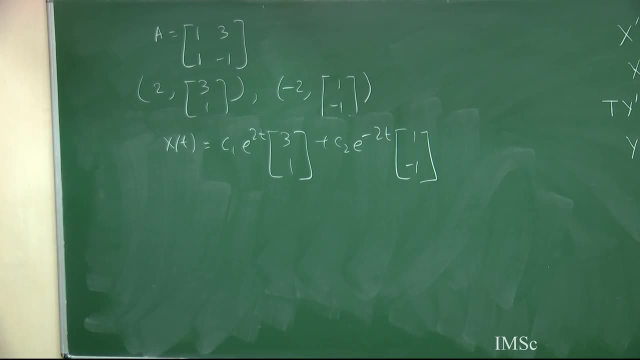 t 3, 1 plus C, 2 e, to the power minus 2 t 1 minus 1.. So what we have done earlier, in this case also, first of all, we can try to find out two straight line solutions. So how can you find out straight line solution? 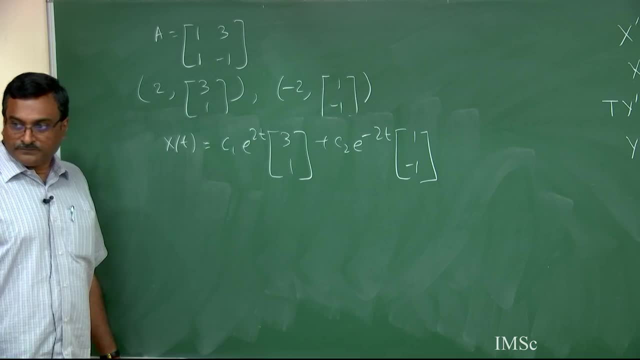 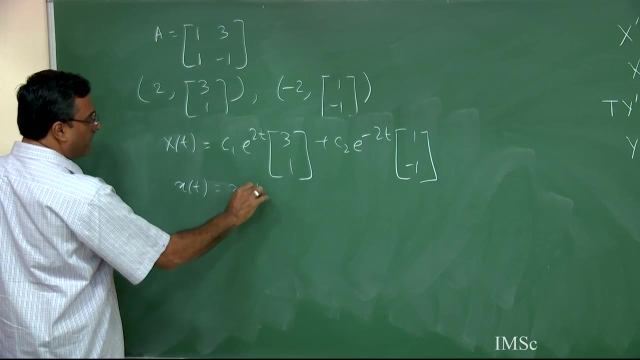 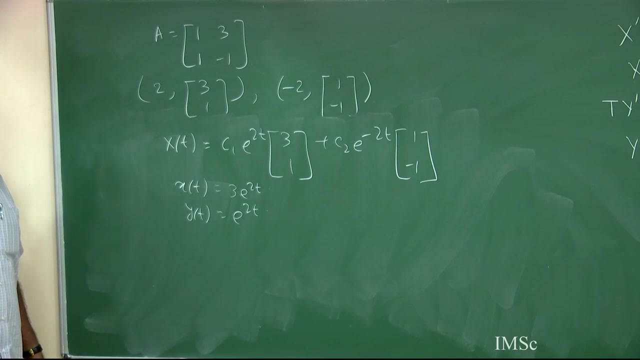 You substitute C 1 equal to 1.. And C 2 equal to 0. if you choose C 1 equal to 1 and C 2 equal to 0, then you will be having X- t is equal to 3, e to the power 2 t and y t. this is equal to e to the power 2 t, right. 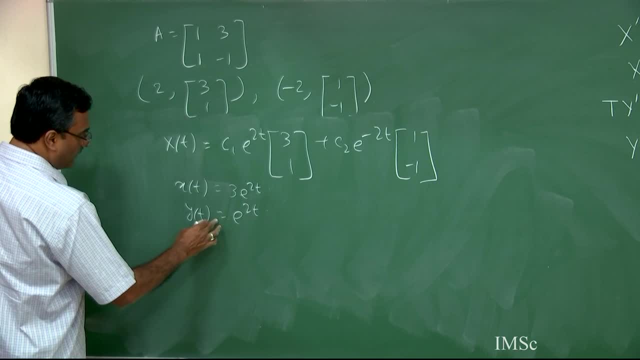 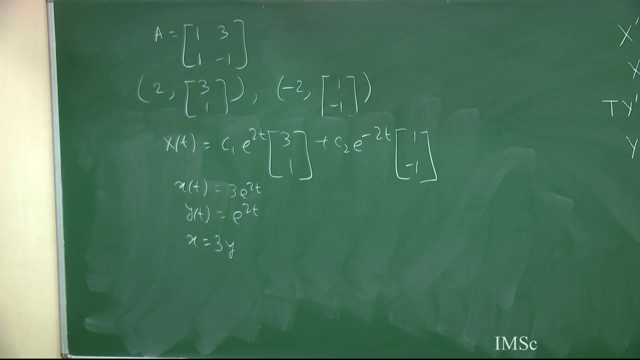 So therefore, X equal to this is 3, this is 1.. So, therefore, if you multiply this by 3, so therefore this is equal to 3, this one. So you will be having X equal to 3, y. this is one solution. 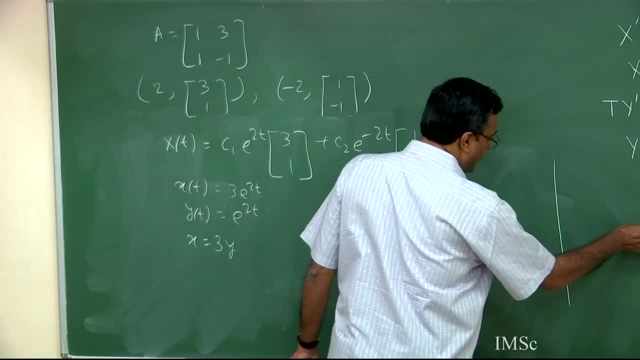 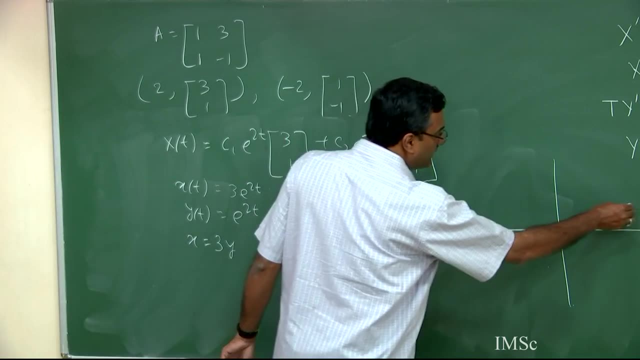 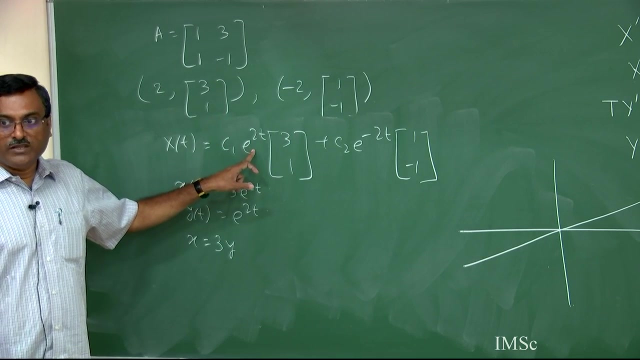 So in the phase portrait, this is your vertical y axis, this is x axis. So y equal to one-third x. y equal to one-third x means you will be having roughly a straight line like this. Now, along this line, the coefficient is e to the power 2 t. this is positive. 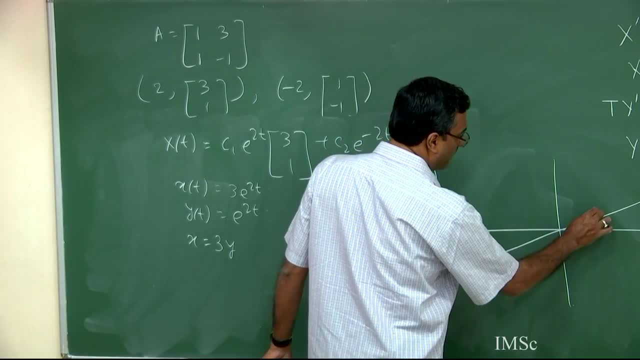 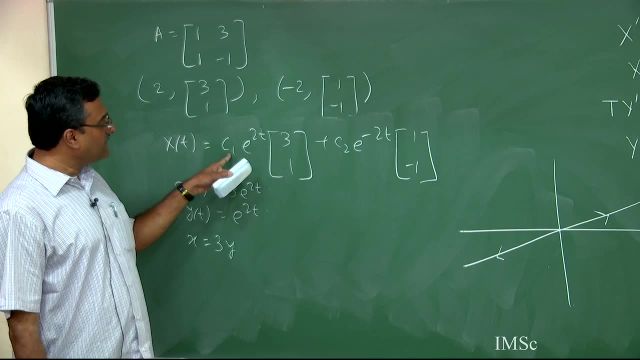 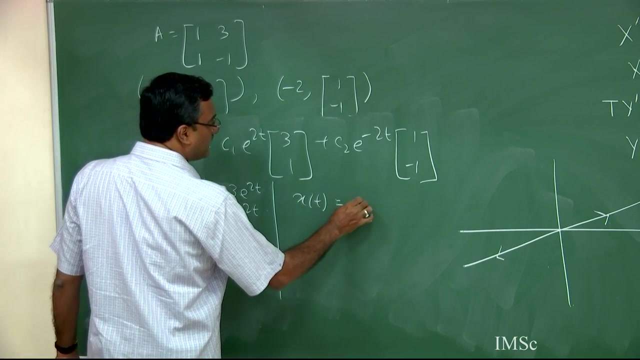 So solution will be approaching away from the origin. Thank you. Similarly, if you consider C 1 equal to 0 and C 2 equal to 1, so then you will be having X t, that is equal to e to the power, minus 2 t, and y t- this is equal to minus e to the. 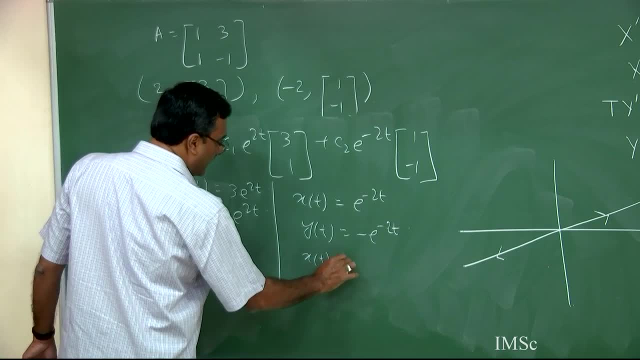 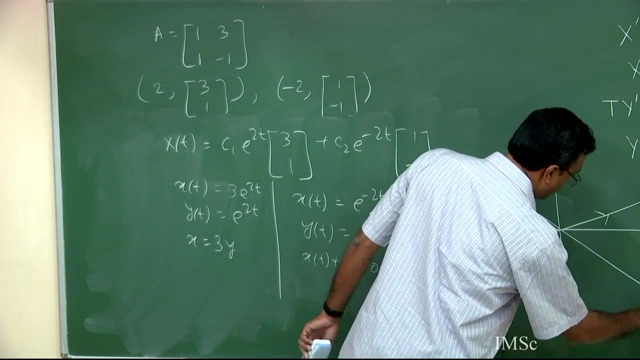 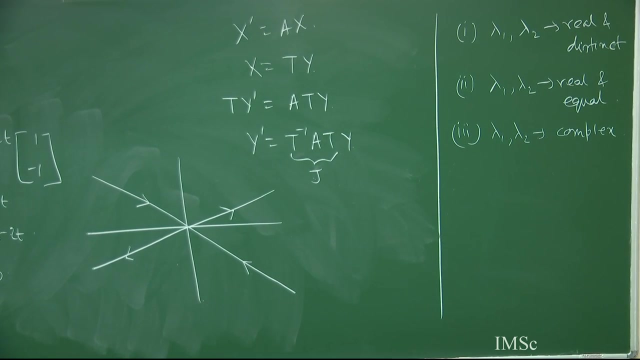 power minus 2 t. So therefore solution is X t plus y t. this is equal to 0, so that means this is a straight line along which Trajectories will be approaching towards this one right Now, if you just apply your common sense, that now this axis are rotated little bit. 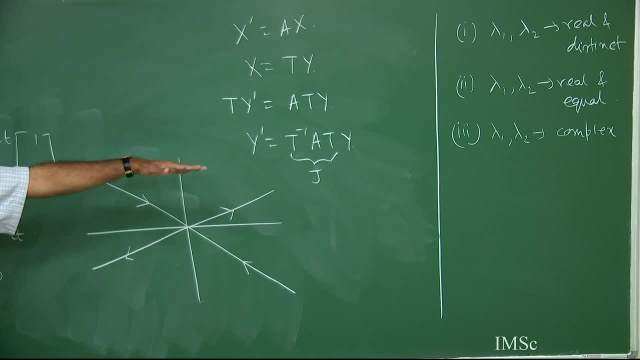 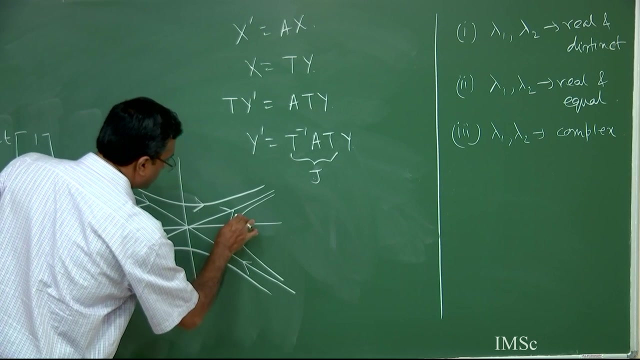 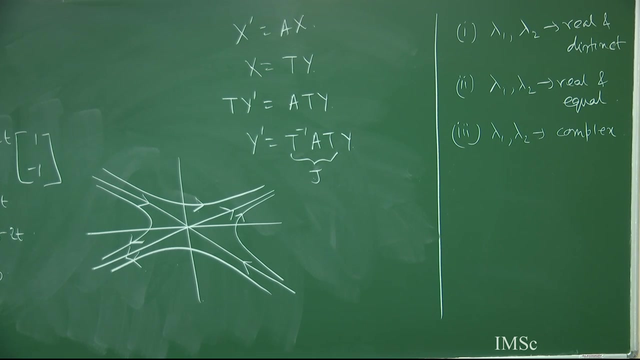 So the rest of the trajectories will be stretched accordingly. So, therefore, the final phase portrait will looks like this one: This is this one And, finally, this is this one, right. So this will be the solution structure for the, this kind of two variable system with 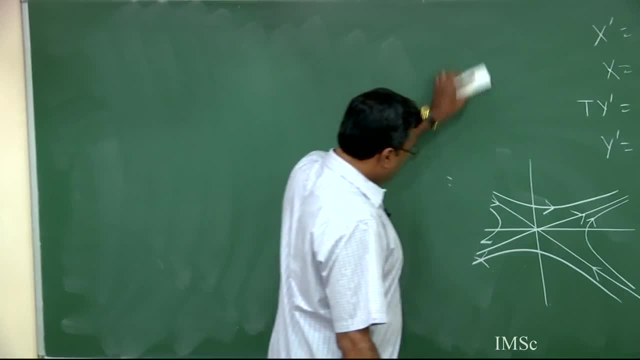 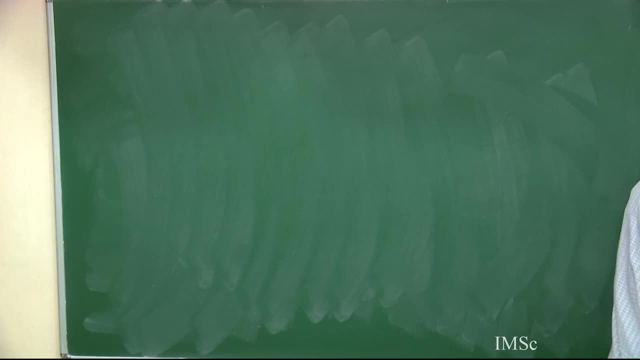 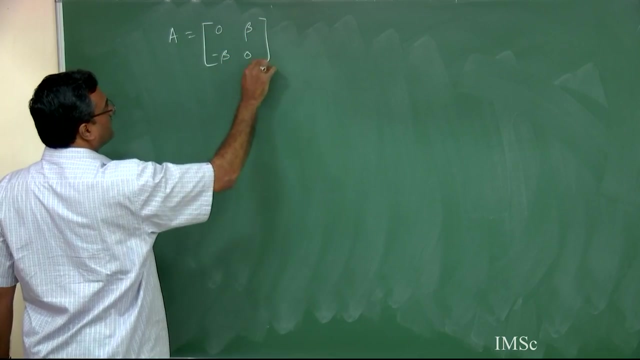 real eigenvalues. Now, in case of complex eigenvalues, the question is that given system of equations are real. then how to find it? Then how to find out two real solutions out of this, whether we can apply the same theory or not. For that purpose, you choose this matrix: A equal to 0, beta minus beta 0. this is the matrix. 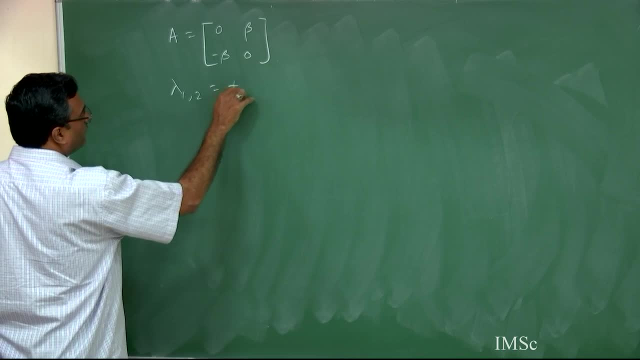 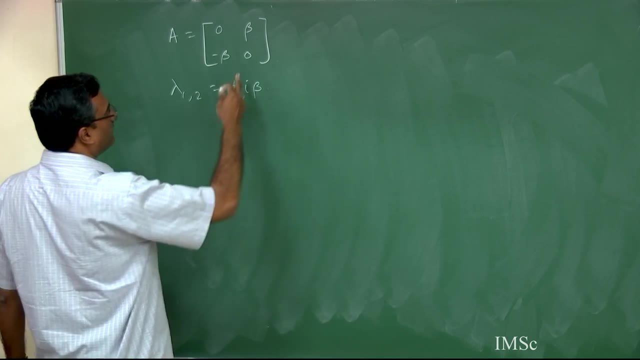 So immediately you will be having the eigenvalues lambda 1 comma 2, that is plus minus. i beta. these are the eigenvalues. If you interested to find out, we need to find out the eigenvectors. So therefore, 0 beta minus beta 0.. 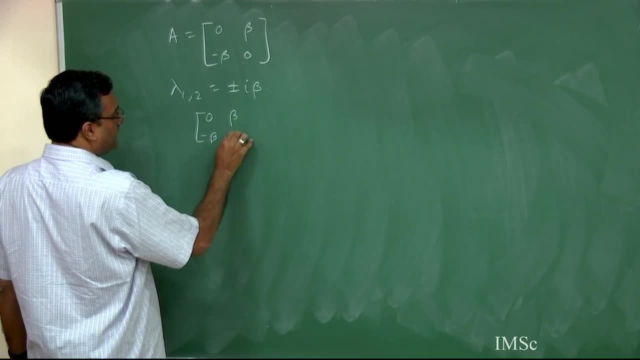 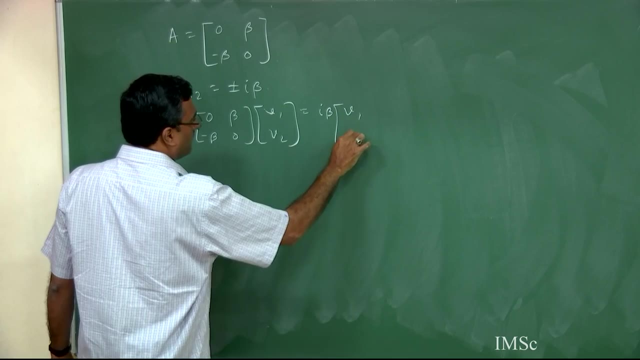 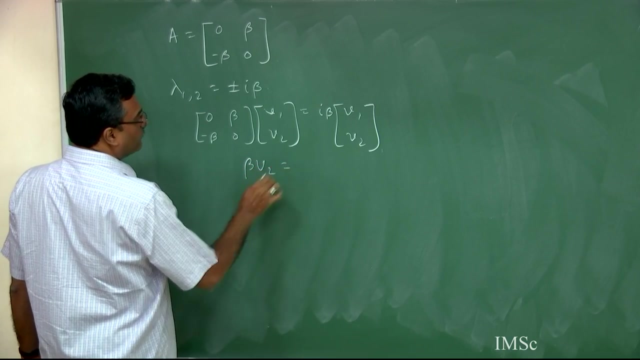 Okay, So 0 beta minus beta 0. this multiplied with v 1 v 2.. So this is equal to i beta times v 1 v 2.. So from the first equation you will be having beta v 2. that is equal to i beta v 1.. 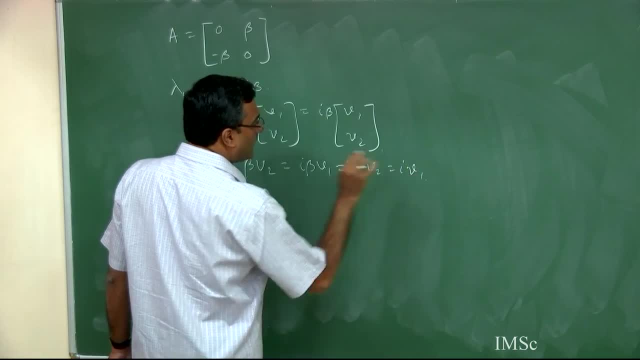 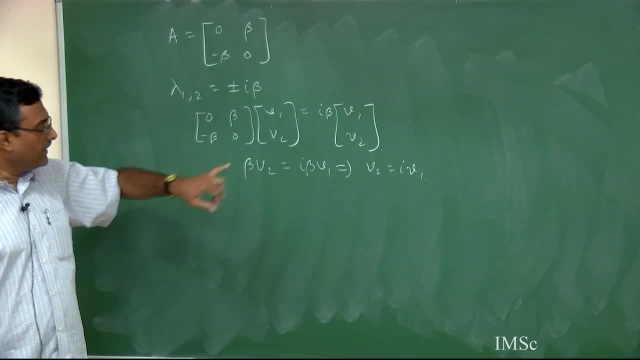 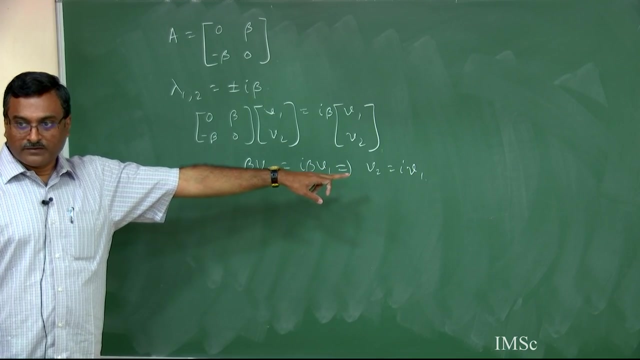 So implies v 2 equal to i v 1. right Now, if you solve the second equation, Solve for the second component, that is, minus beta v 1 is equal to i beta v 2. then you will be having the same equation, right. 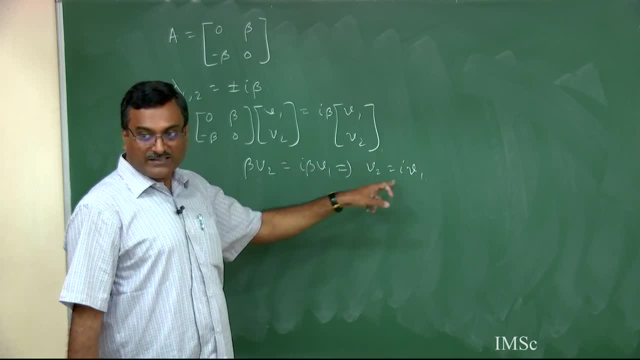 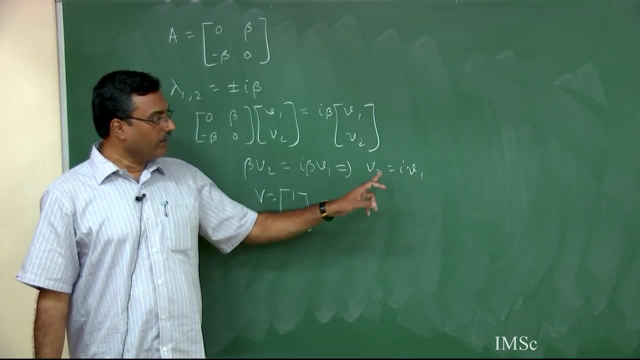 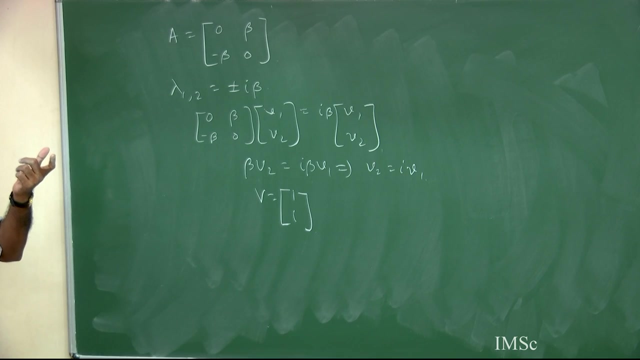 So therefore from here we can find out the eigenvector as v equal to 1, i. So if you choose v 1 equal to 1, so v 2 is coming out to be i. right Now you apply the same result, that means e, to the power lambda t into v is going to be: 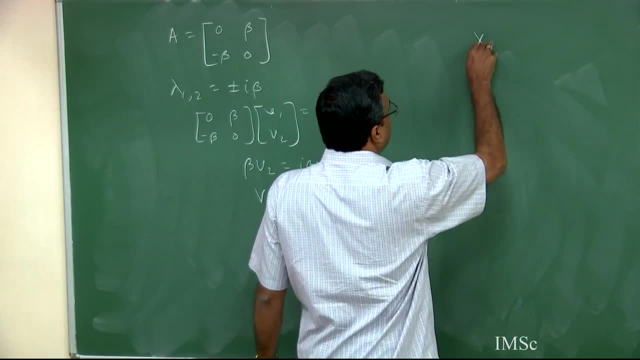 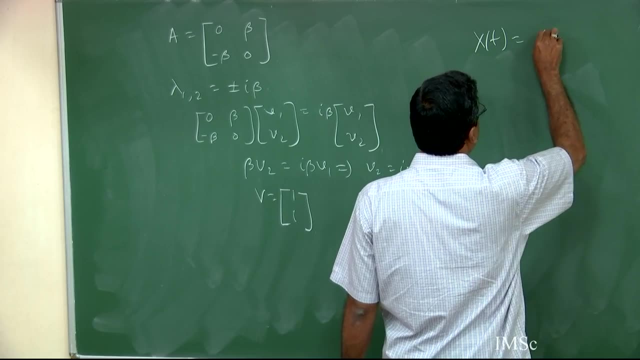 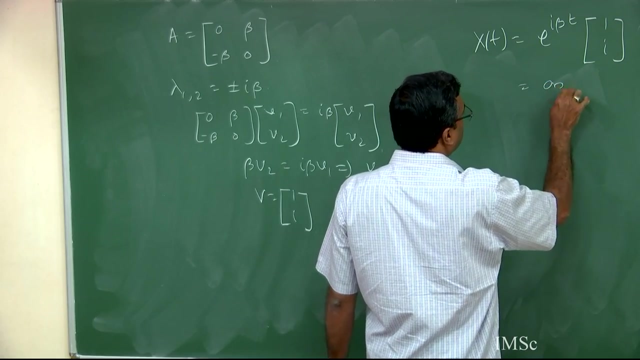 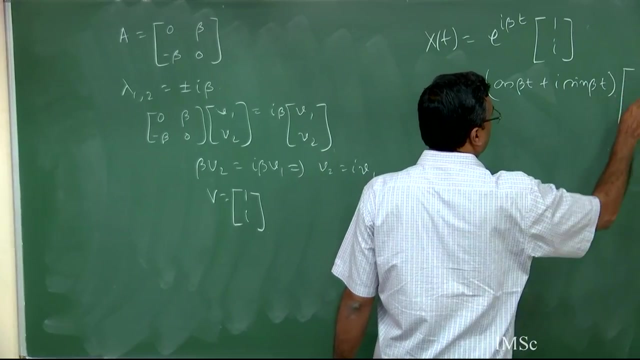 a solution for the given system. Interestingly, in this case you will be having two real solutions from this single expression: e to the power lambda t into v, So e to the power i beta t. this multiplied with 1 i. So that means cos beta t plus i sin beta t, this multiplied with 1 i. and now from here: 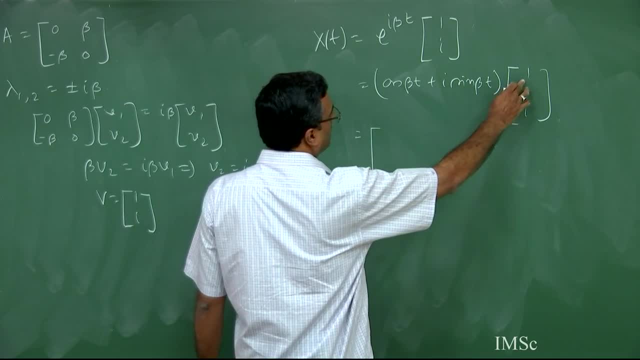 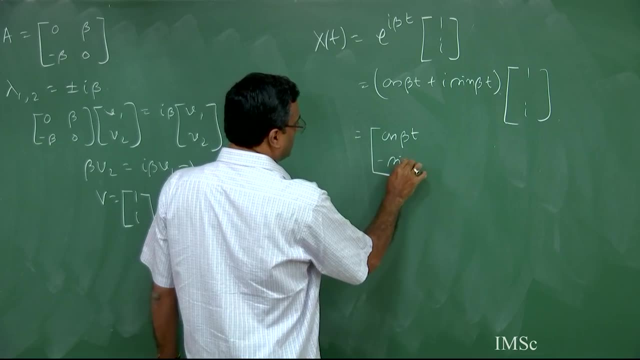 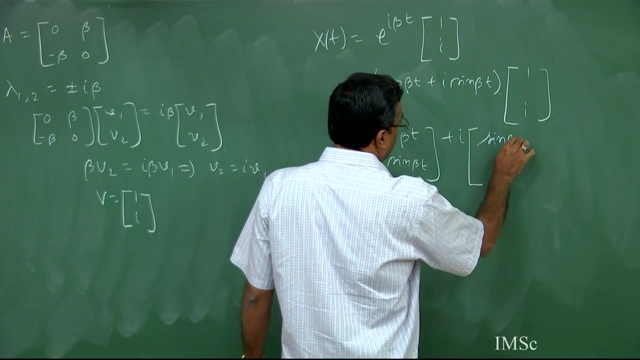 if you separate the real and the real, Okay, So if you separate the real and imaginary part, so from the first equation you will be having cos beta t, this multiplied with this one, so that is minus sin beta t. this is the real part, plus i times sin beta t and then cos beta t. 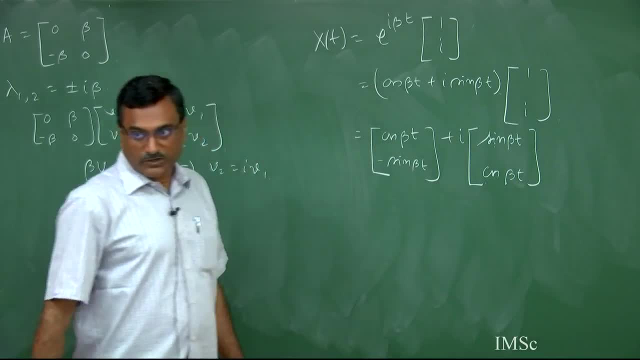 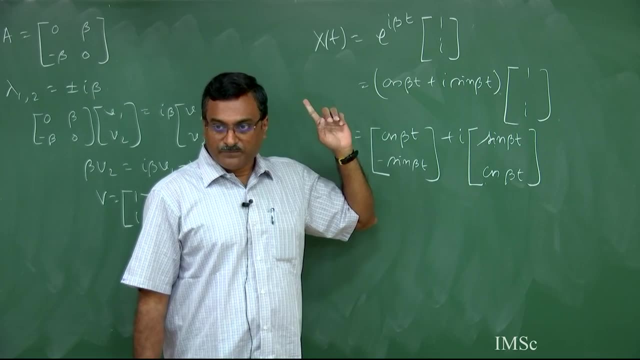 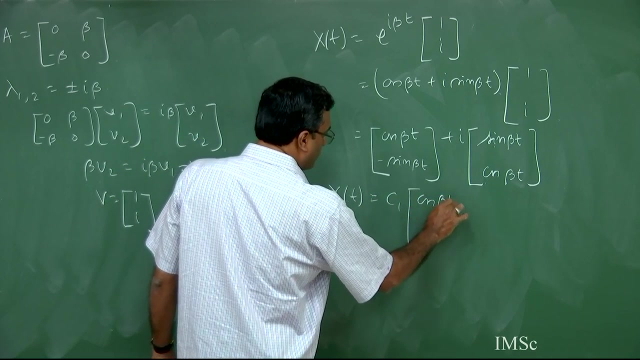 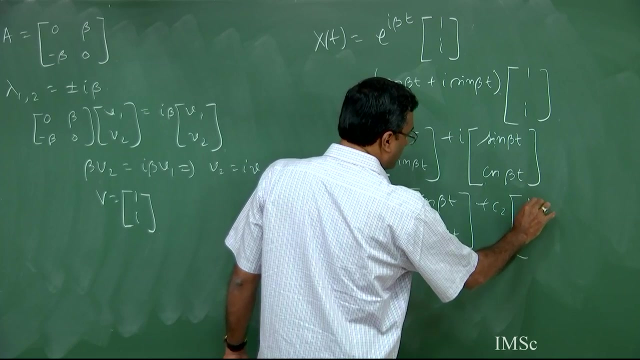 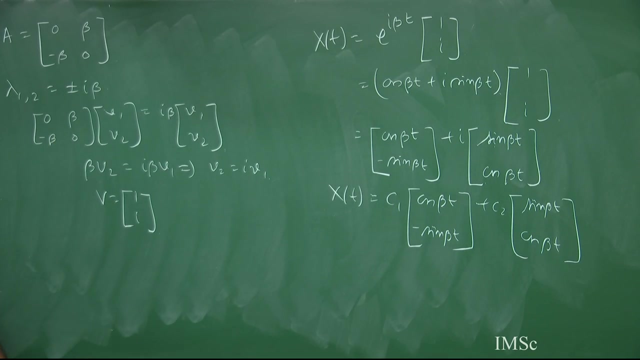 So this is the real component and imaginary component and you can verify that these are two linearly independent solution For the given system. so therefore, general solution: x, t. this is given by c 1 cosine beta t minus sin beta t plus c 2 sin beta t, and this is cosine beta t, right. 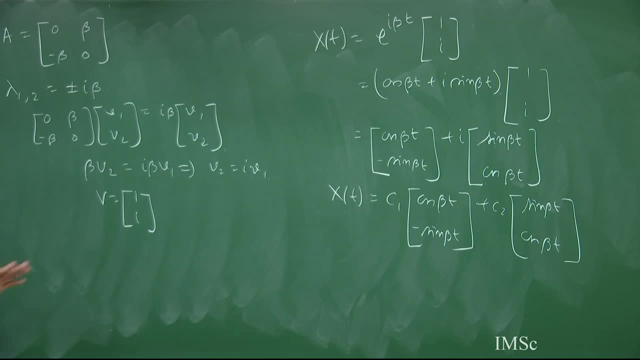 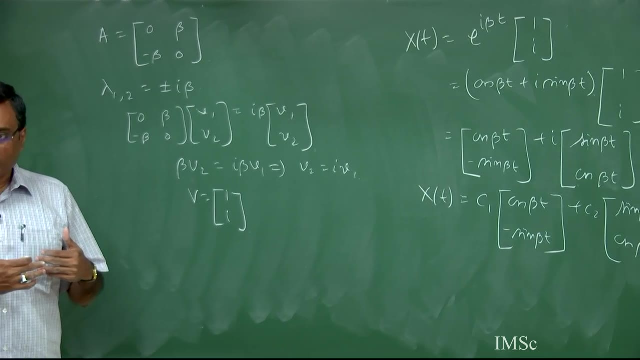 Now, in this case, there is no straight line solutions, correct? You cannot find a straight line solution. You cannot find a straight line solution, Okay, You cannot find out any straight line solution by a specific choice of c 1 and c 2.. 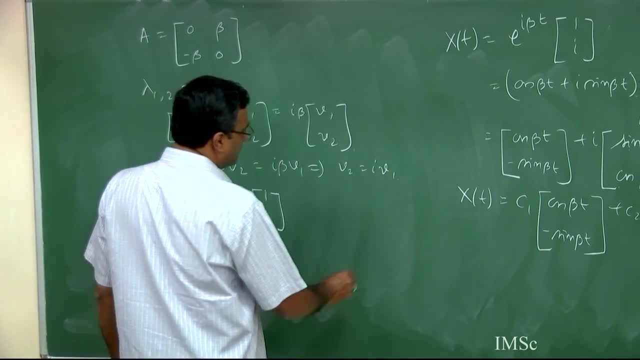 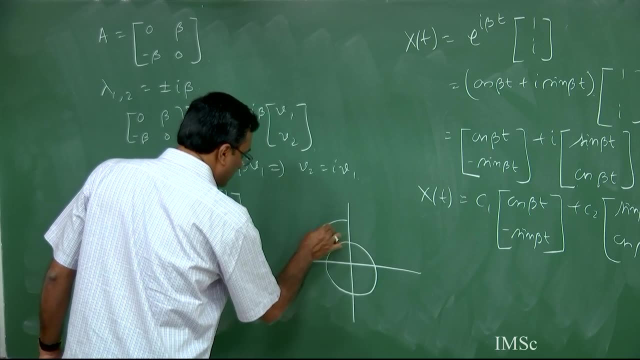 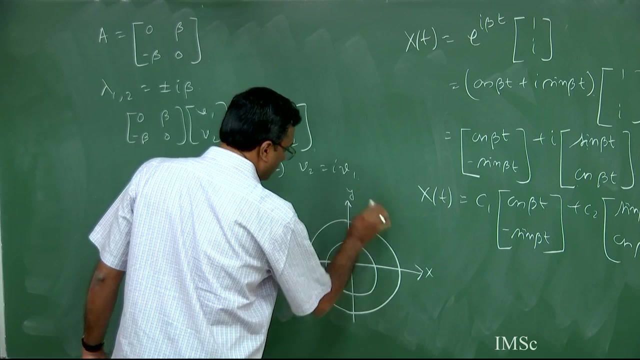 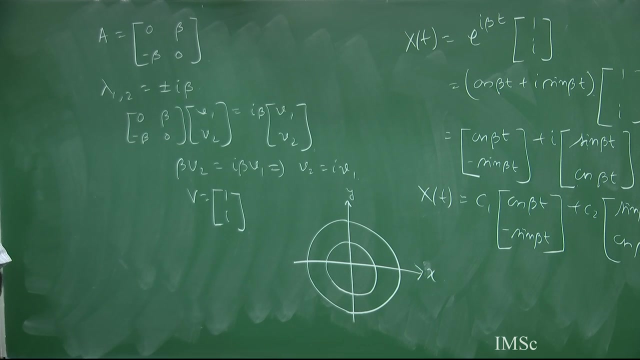 So how the solution trajectories are looks like. Solution trajectories will be, in this case, all concentric circles. These are all concentric circles, but after getting this concentric circles, we need to understand what will be the direction of the solution trajectories. These are going to be clockwise or anticlockwise. 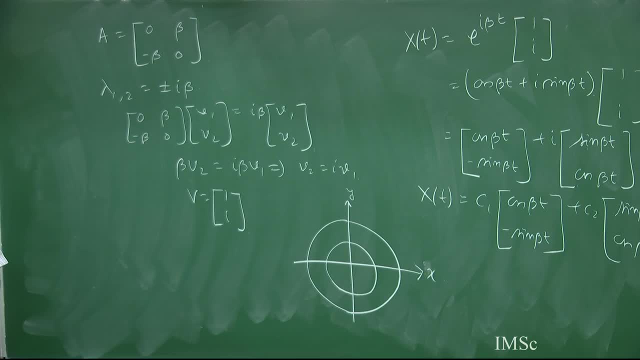 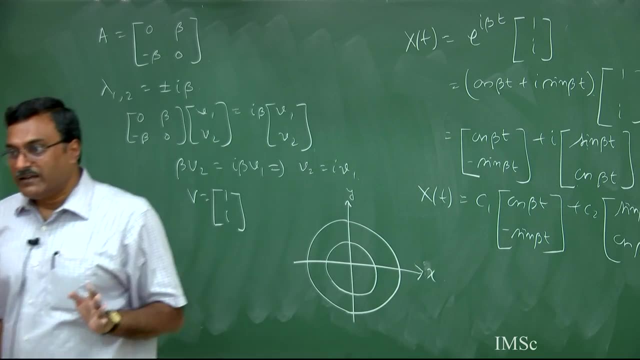 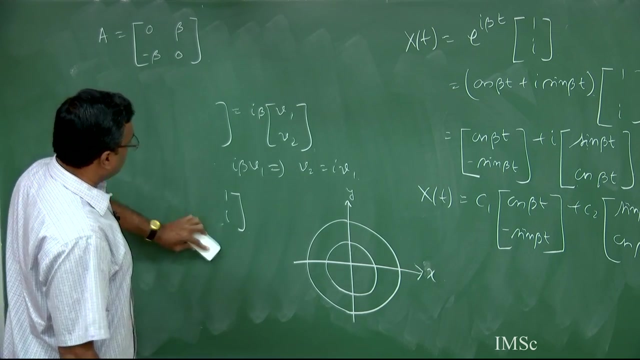 Okay, So this rotation- whether it is clockwise or anticlockwise, that should be determined by the value of beta, correct? Now the question is that how we can ensure that? what is the appropriate direction of the solution trajectories? Now, in order to understand that particular direction of the solution trajectories, you 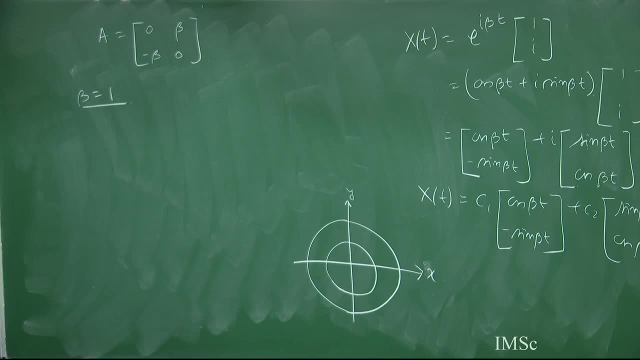 take a specific example: beta equal to 1, right, Okay? Okay, So you can have a clever choice for c 1 and c 2 in order to understand in which direction solution trajectories will rotate. So what is the clever choice? c 1 equal to 1, c 2 equal to 0. then your solution is x. t is. 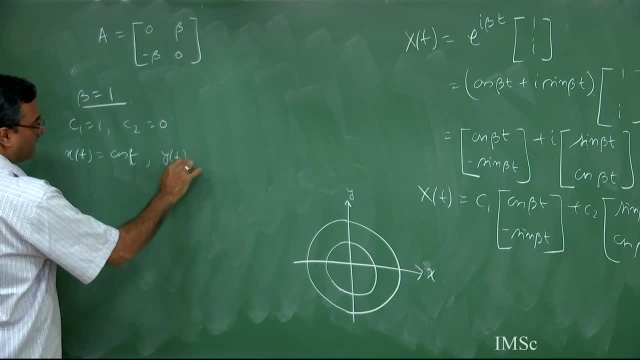 equal to cosine t and y t. this is equal to minus sine t. Now, if you choose two particular time point, that is t equal to 0.. So this corresponds to a point 1 comma 0 on x axis. Next, if you choose another point: t equal to pi by 2.. 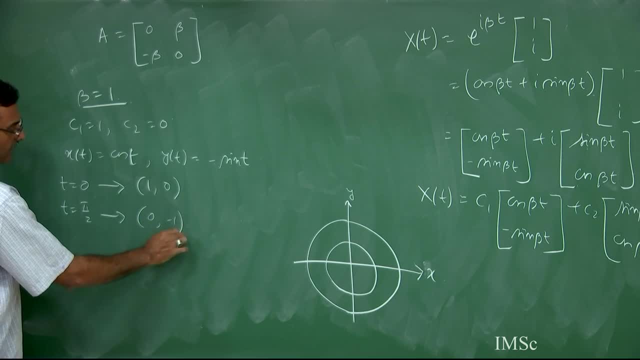 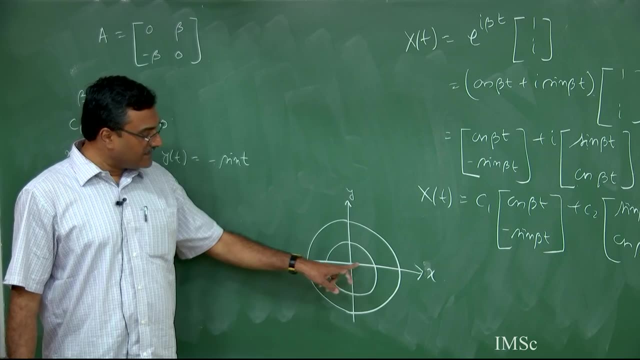 So then this will be giving you a point on the negative y axis, correct, So without a loss of generative. you can, if you assume that this distance is 1, 0. So therefore this will be 0 comma minus 1.. So at t equal to 0 if you start from here. 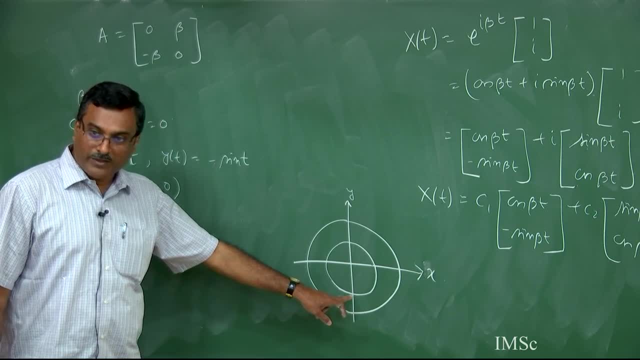 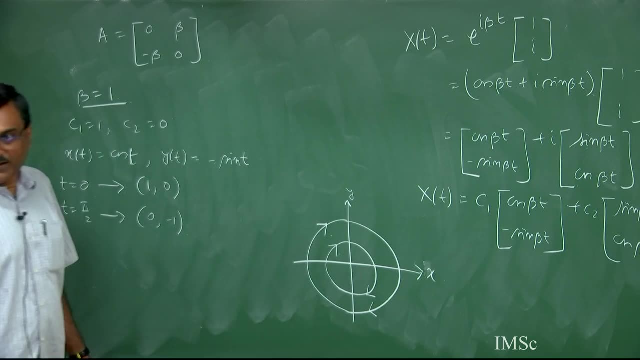 So trajectory will be reaching, at this point, At t equal to 0.. At t equal to pi by 2.. So, therefore, rotation is going to be in this direction, right? So once you have a specific values of beta, you substitute the value of beta and then 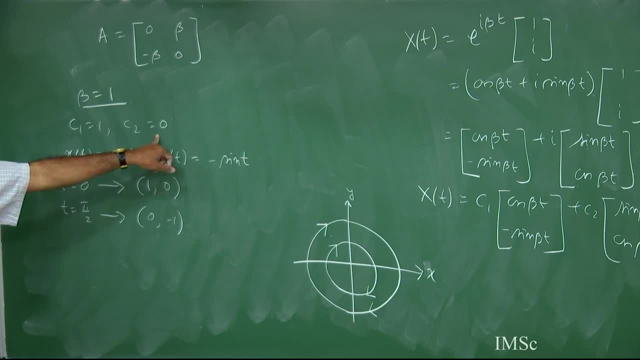 choose c 1 equal to 1 and c 2 equal to 0, or c 2, c 1 equal to 0, c 2 equal to 1, and then you can find out two points like this. So immediately you will be having in which direction solution trajectories will move. 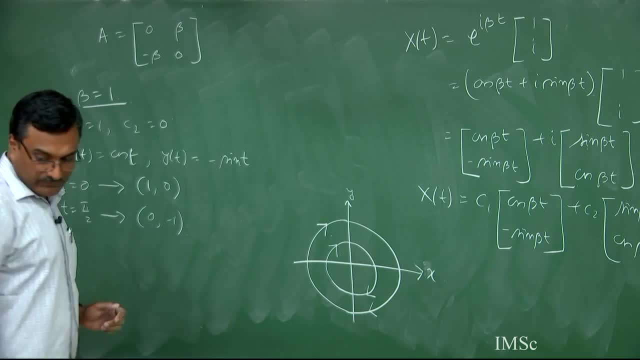 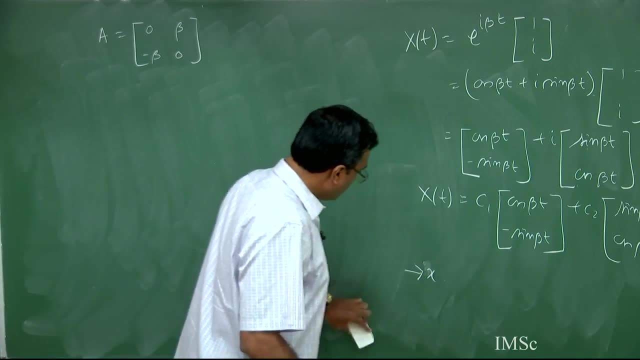 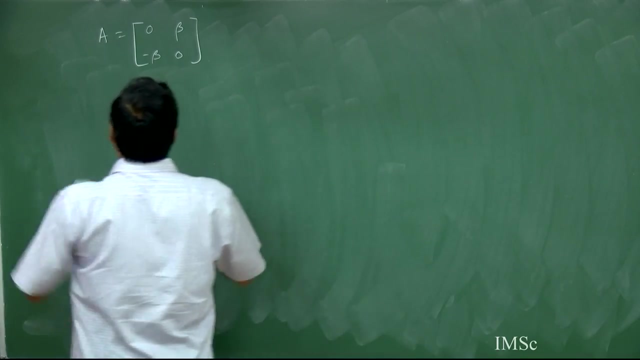 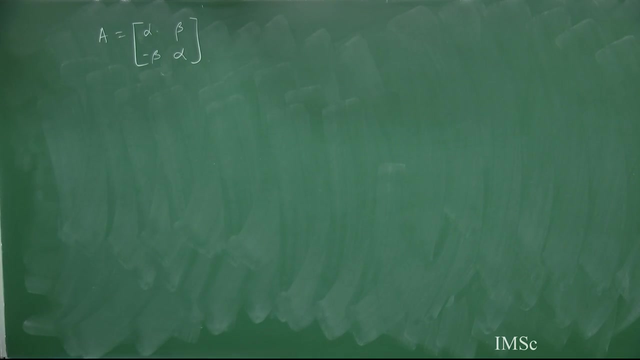 Correct. Now another case where you will be having complex conjugate eigen values. I am not going into the details, but I am sure you will be able to work out this kind of problem. that is, a equal to matrix, alpha, beta minus beta, alpha, right. In this case, what will be the 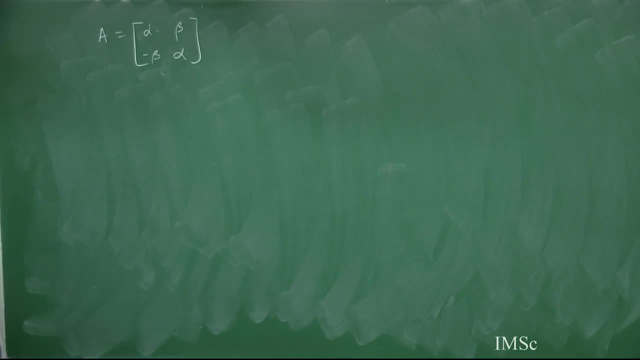 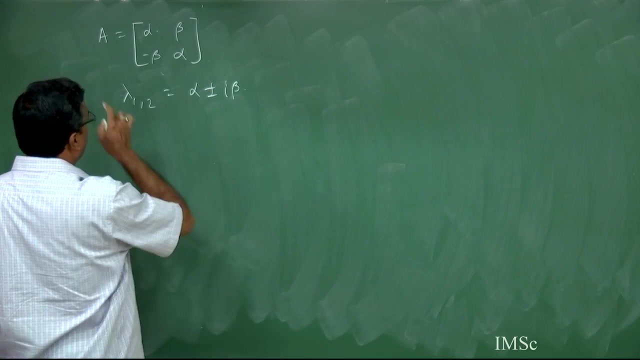 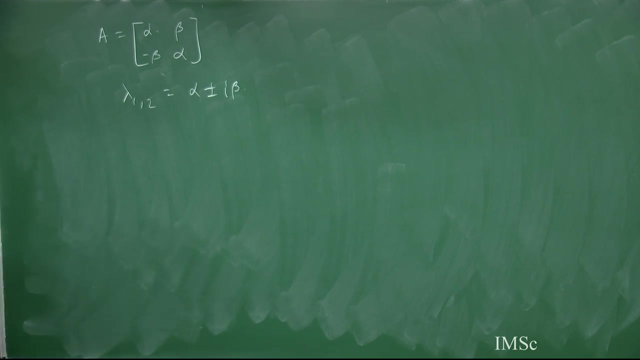 Okay, Now change in the system. change in the system will be: Eigen values are lambda, 1 comma 2, that is alpha plus minus i, beta, and you can verify that v 1 will be the same Eigen vector, 1 comma i. and if you proceed in a similar manner, So in this case you will be having 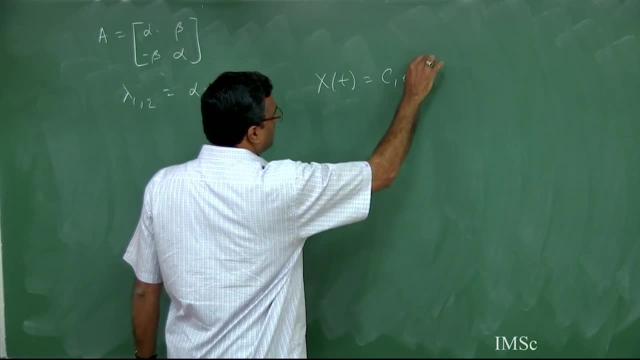 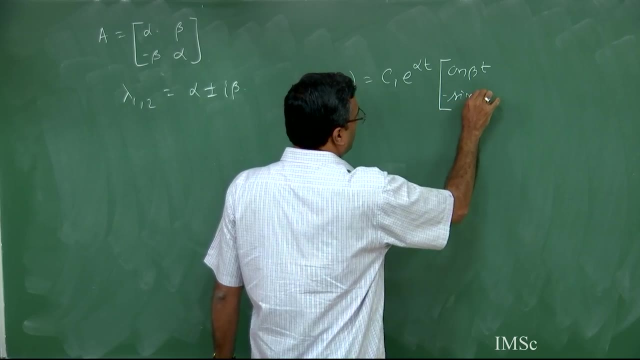 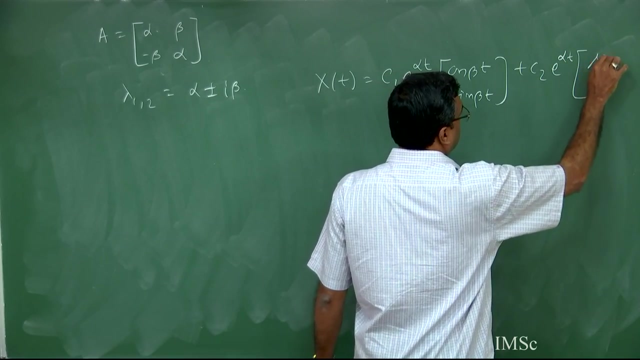 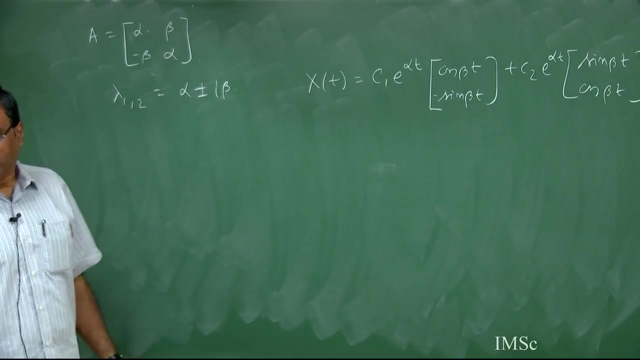 the general solution: x t equal to c 1 e to the power alpha t. this multiplied with cosine beta t minus sine beta t plus c 2 e to the power alpha t, this is sine beta t and this is cosine beta t, this one. So accordingly in this case also you can. 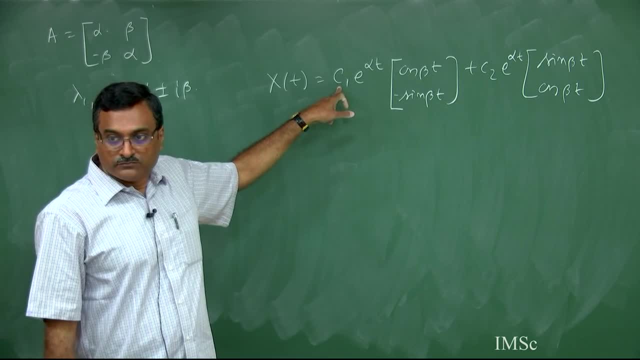 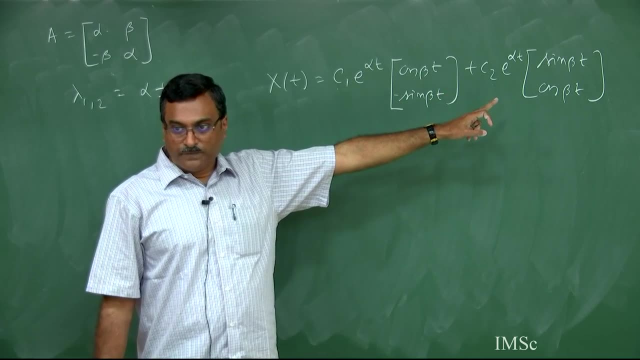 choose c 1 equal to 1, c 2 equal to 0. So if your alpha greater than 0, then you can choose c 1 equal to 1, c 2 equal to 0, then trajectories will move away from the origin. 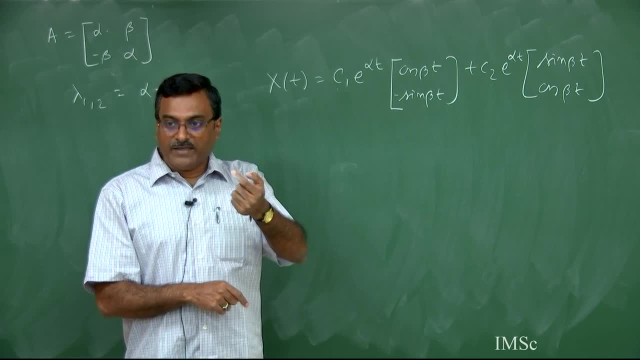 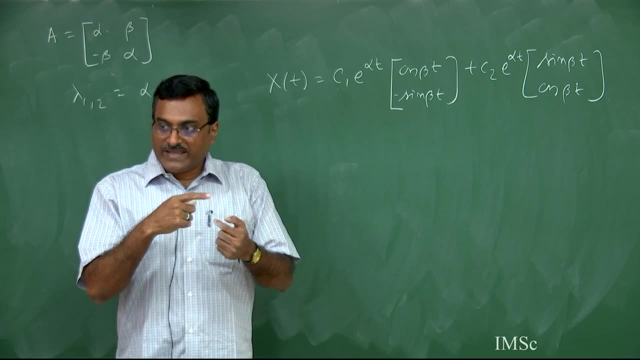 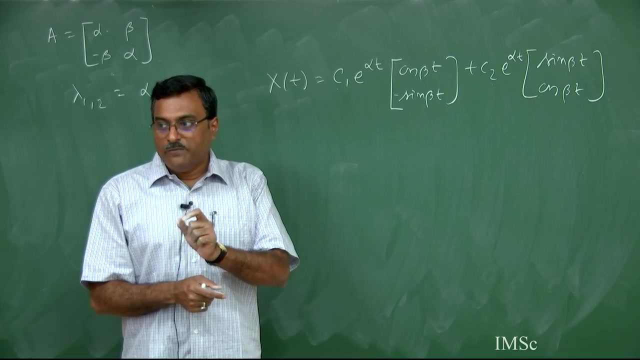 If your alpha less than 0, solution will be coming inside. that means towards origin, and trajectories are spiral, either with decaying magnitude or increasing magnitude. So, depending upon the values of alpha and beta, you will be having four different kind of phase portraits. 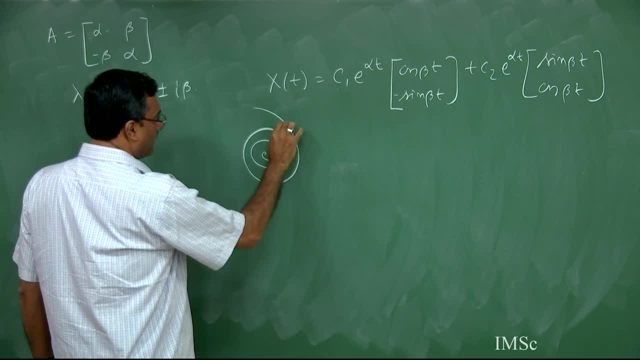 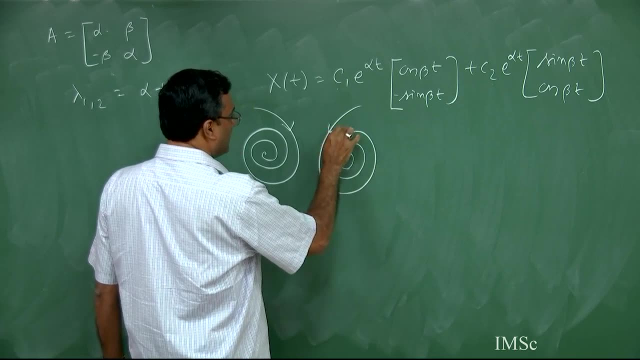 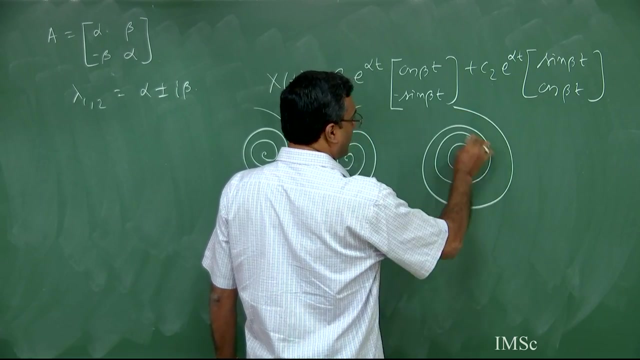 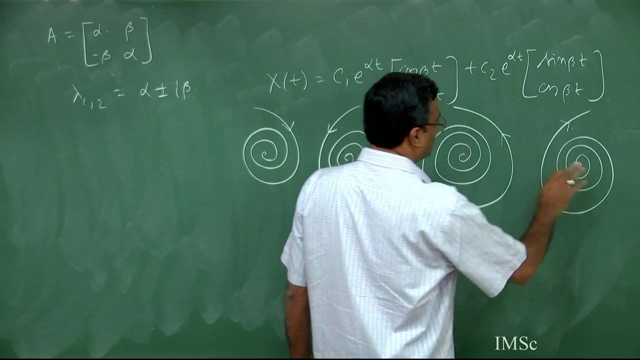 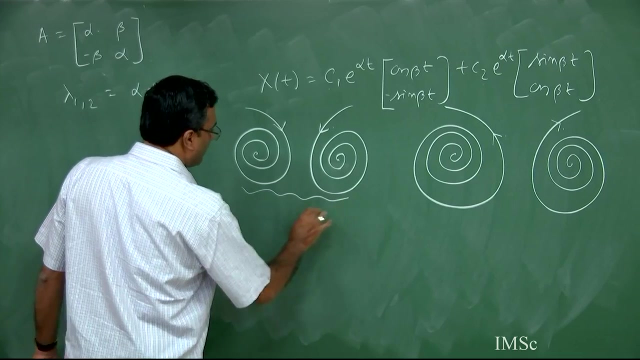 One is like this: Okay, If alpha less than 0,, either this one or this one. in case of alpha less than 0, and in case of beta- whatever may be positive or negative- and alpha greater than 0,, then you will be having any one of these two structures, right? So these two cases for alpha less than 0,. 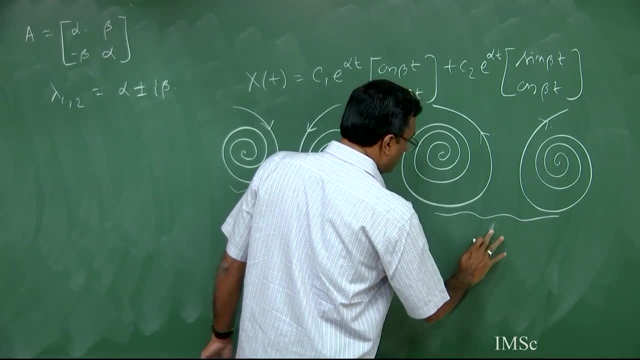 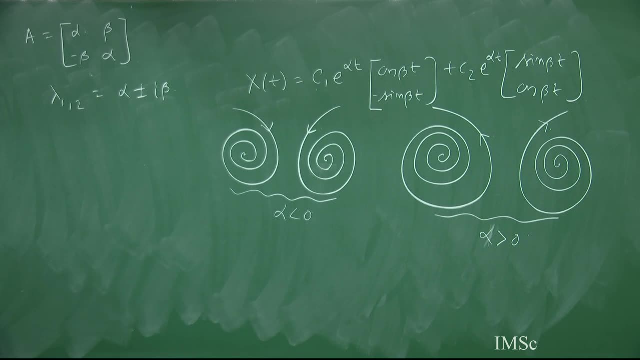 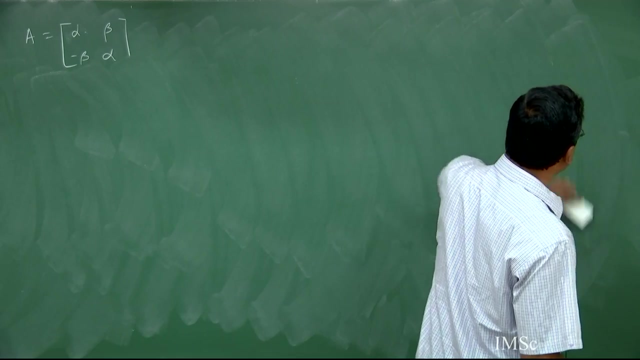 and these two cases for alpha greater than 0, right. So finally, we are left with only one more case, that is, where both the Eigen values are real and equal. If your associated Jordan canonical form is of the form that is lambda, 0, 0 lambda. 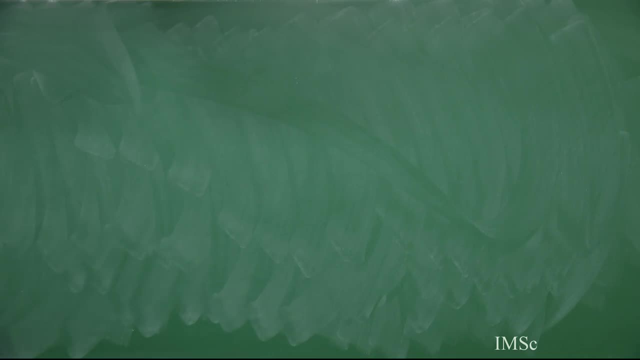 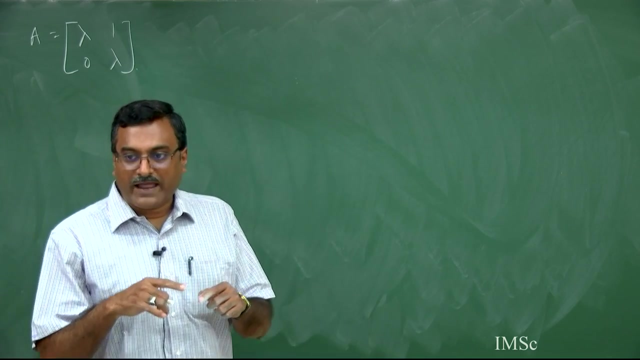 You can apply the first approach in order to find out the general solution. But in case your Jordan canonical form is given by lambda 1, 0, lambda this one, then that particular technique of e to the power, lambda t into v, as a solution of the given system will not work only for. 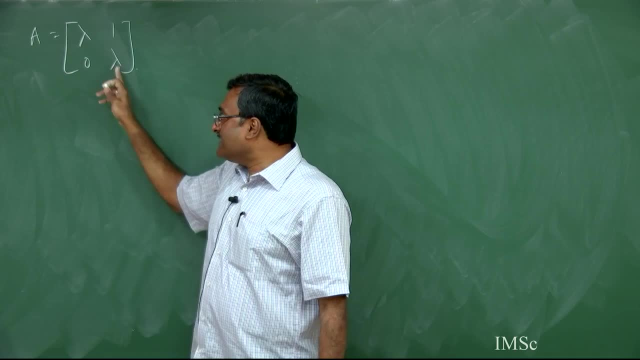 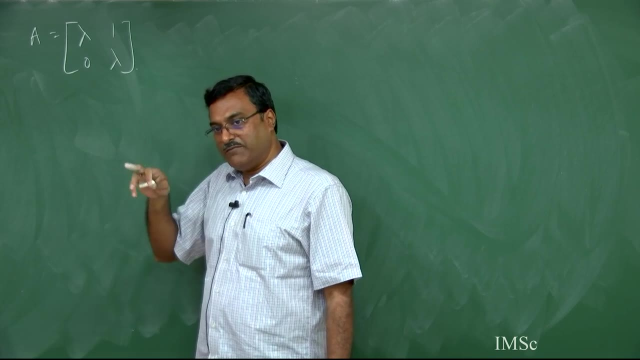 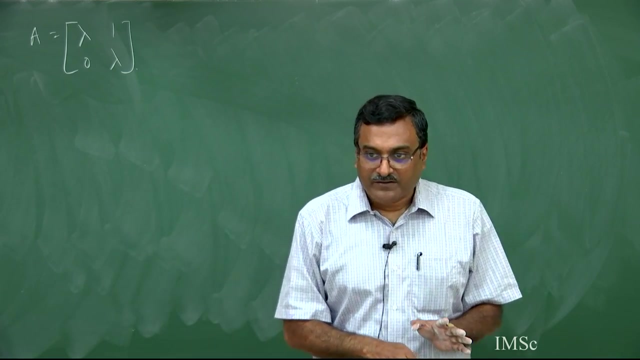 the reason? because here lambda is a repeated Eigen value And you can verify that. if you solve the Eigen value Eigen vector problem, that is a v equal to lambda v, you will be able to find out only one Eigen vector. So there is a concept of generalized Eigen vector. 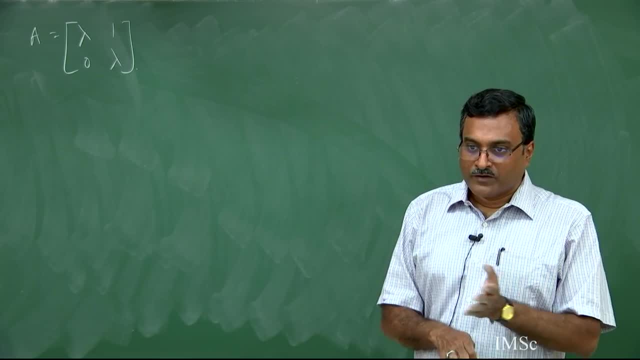 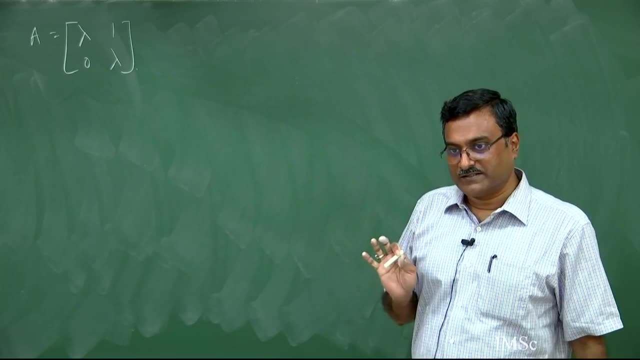 I am not going into the mathematical details because this is a part of the course on mathematical biology itself. So I am giving you the straight forward way out to find out a general solution for this system. It is in some sense very nice structure because x dot t is equal to. 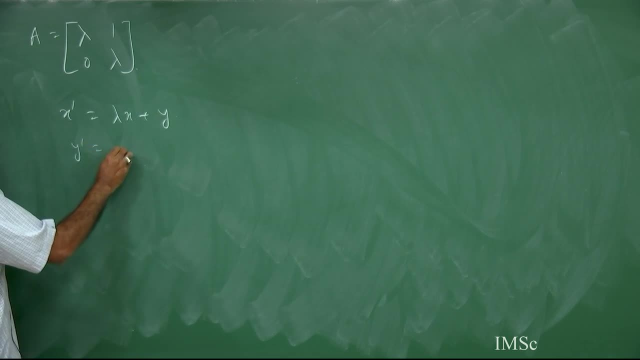 lambda: x plus y. Okay, And y dot t that is equal to y itself, correct? So if you solve the first this equation, y dot equal to y. So this implies y t that is equal to c 2, e, to the power t. Sorry. 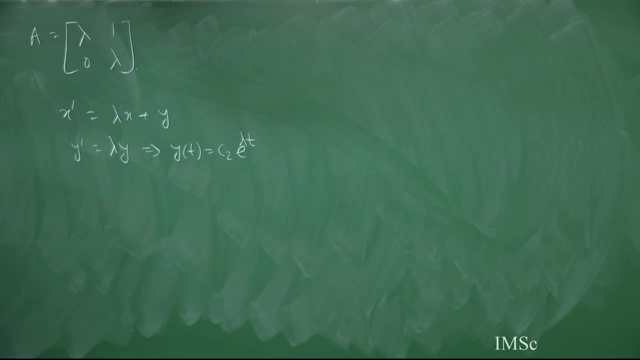 this should be lambda, this should be lambda, right. So you can easily solve this equation: y dot equal to lambda, y equal to this one. Now, if you substitute this solution into this equation, so then you will be having x dot is equal to lambda x plus c, 2, e to the. 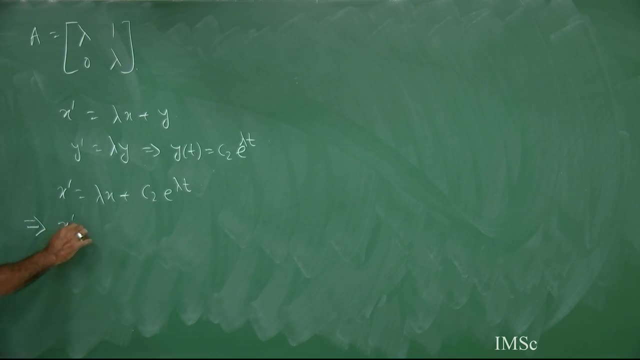 power lambda t. So then you can write down: this is x dot minus lambda x is equal to c 2 e to the power lambda t. Then you can write: d d t of x e to the power minus lambda t, this is equal to c 2 because it is a standard, first order linear, non homogeneous equation. You 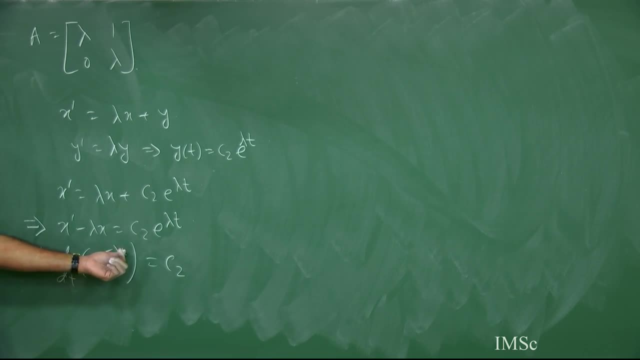 can find out the integrate Okay factor as e to the power minus lambda t. So multiplying both side by e to the power minus lambda t and rearranging term on the left hand side, you can have this expression: And then, if you solve this equation, then you will be having x, e to the power minus lambda t. 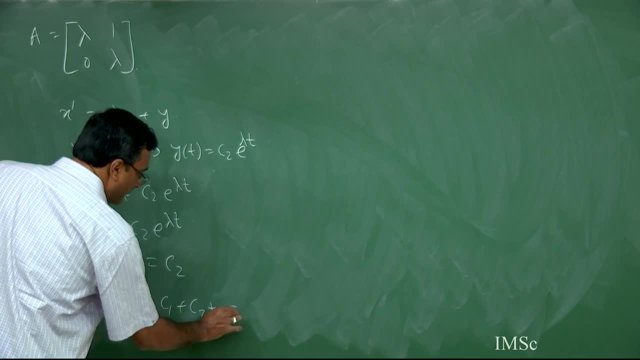 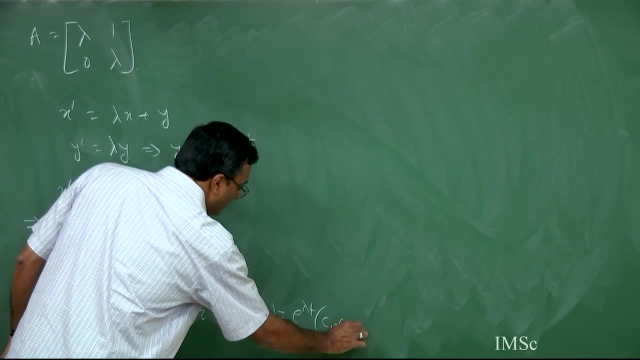 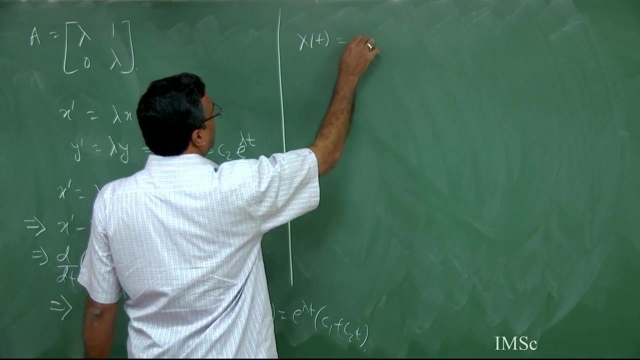 that is equal to c 1 plus c 2 t. So from here you will be having x t equal to e, to the power lambda t times c 1 plus c 2 t. So therefore, what is the general solution? So x t equal. 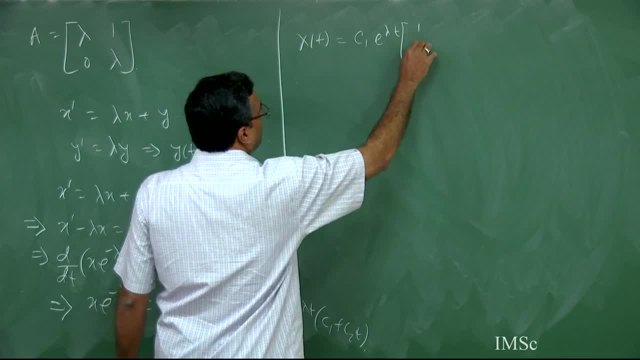 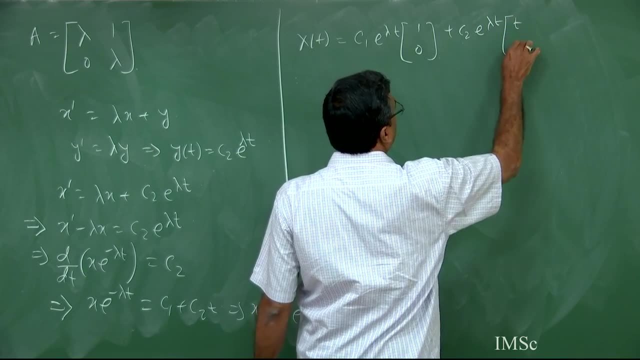 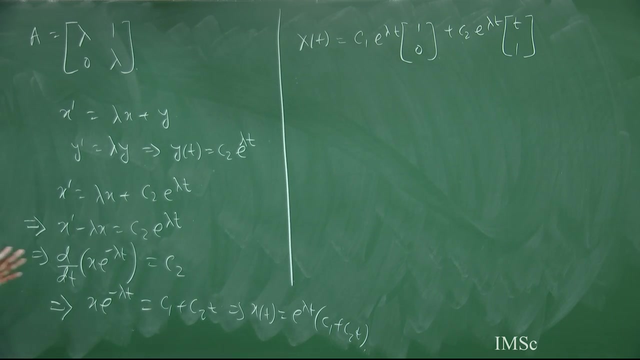 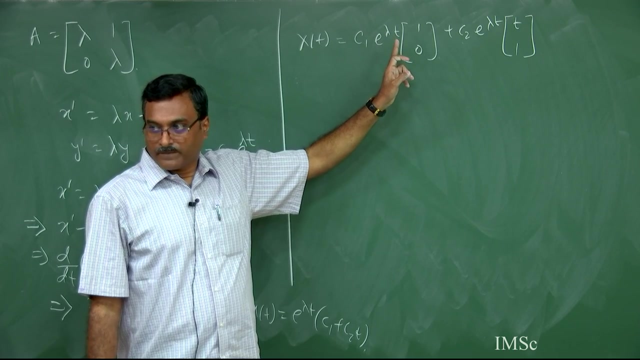 to c 1 e to the power lambda t 1, comma 0, plus c 2 e to the power lambda t t 1, right. So in this case you will be having only one straight line solution That is given by y equal to 0, correct? because if you choose c 2 equal to 1, c 1- non-zero. So 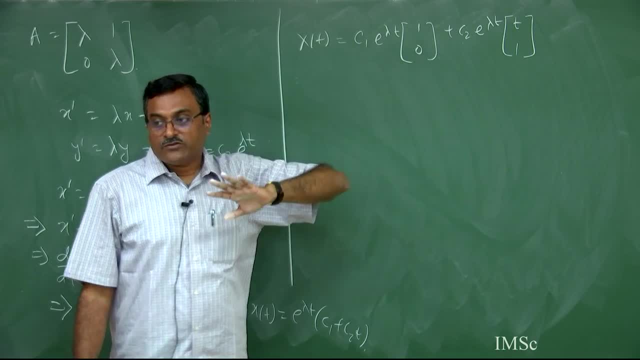 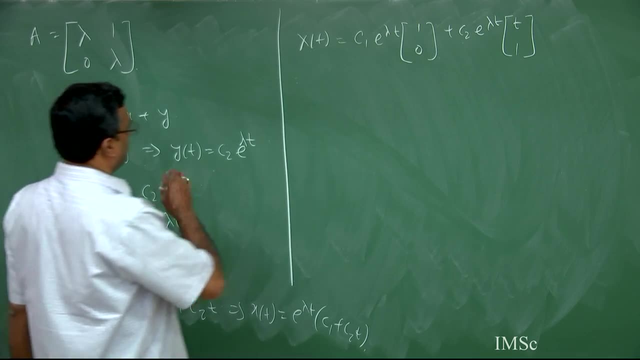 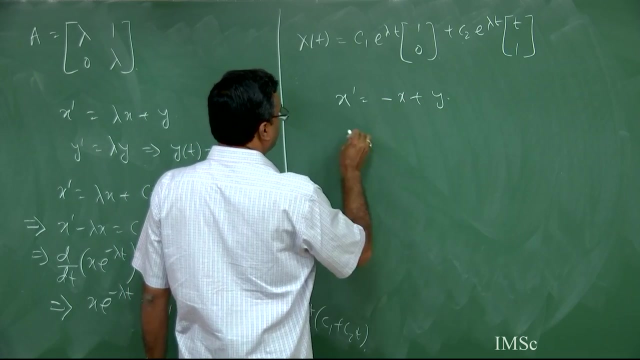 this is not a straight line solution, But the interesting question is that how the solution trajectories looks like for this kind of system. It is a very not a straight forward system. So just consider a specific example: x dot equal to minus, x plus y and y dot equal to. 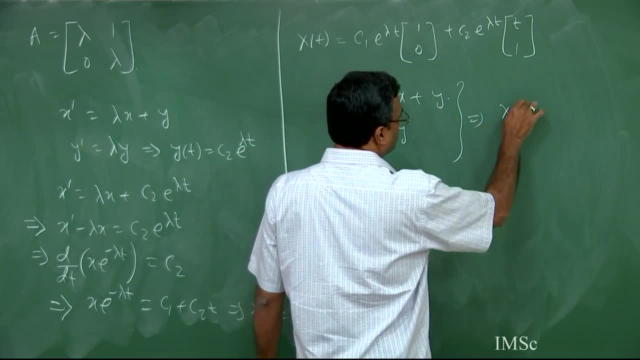 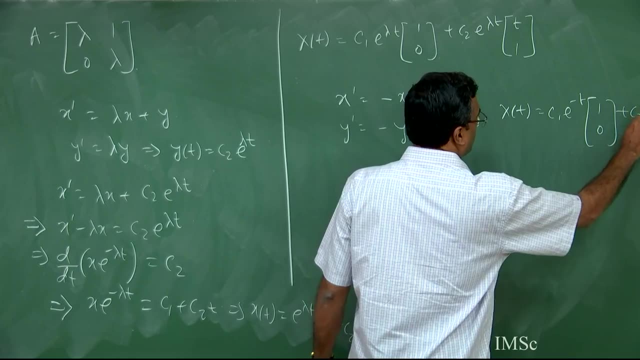 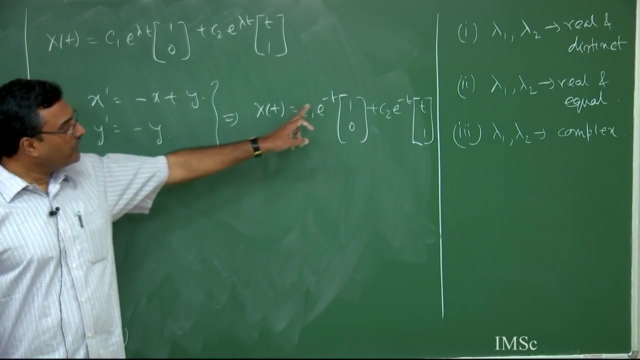 minus y. So for this system solution is x. t is equal to c 1, e to the power minus t: 1, 0 plus c 2 e to the power minus t, this is t, 1.. So you have one solution that is y equal to 0 along. 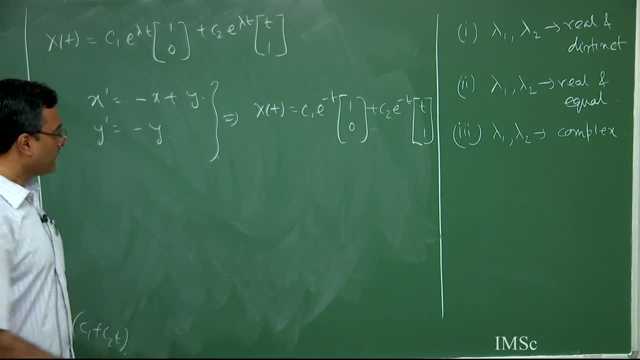 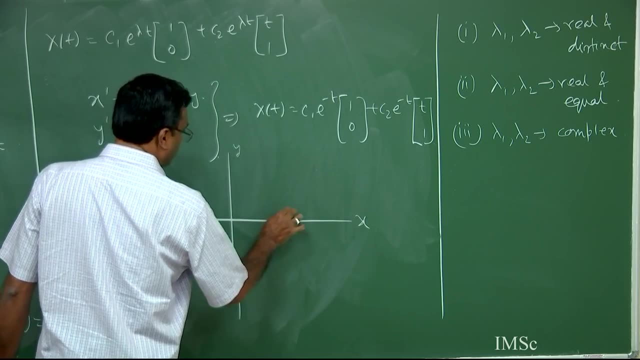 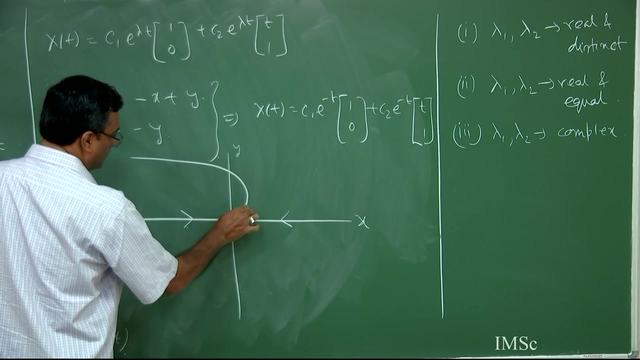 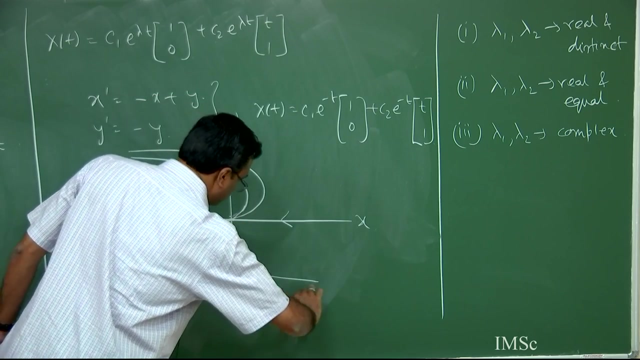 this line solutions are approaching towards the origin. So therefore in x- y plane you will be having this straight line solution x- y. This is approaching towards the origin, But rest of the solution trajectories they looks like this one and this one. Now the question is that how can we speculate that trajectories? 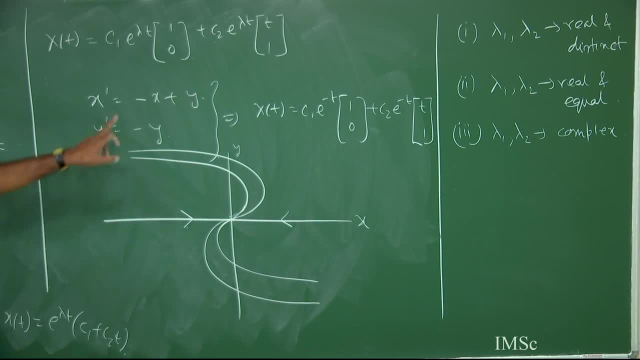 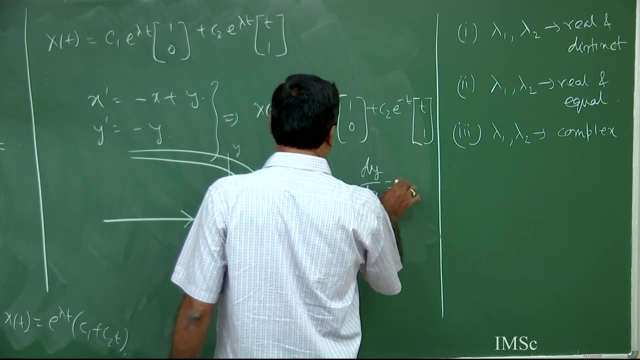 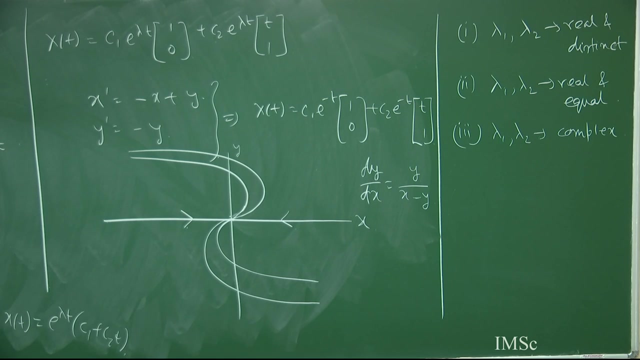 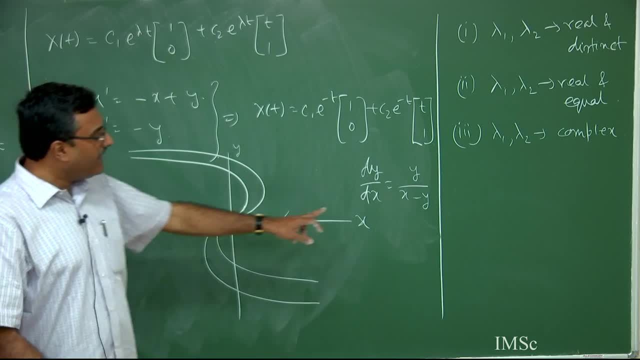 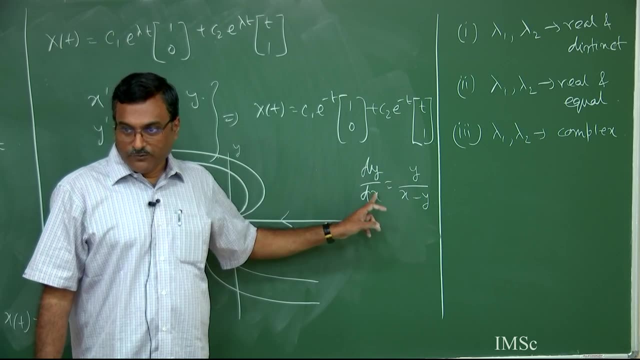 y axis whenever they intersect the line x equal to y, Because if you take x plus x minus y equal to 0, if you take x minus y equal to 0, then d, y, d, x is undefined. So that means tangent to the y axis. 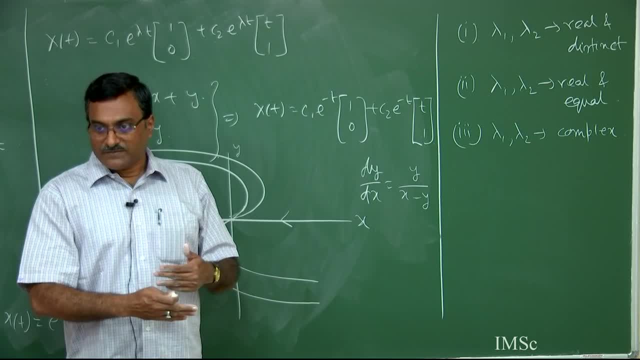 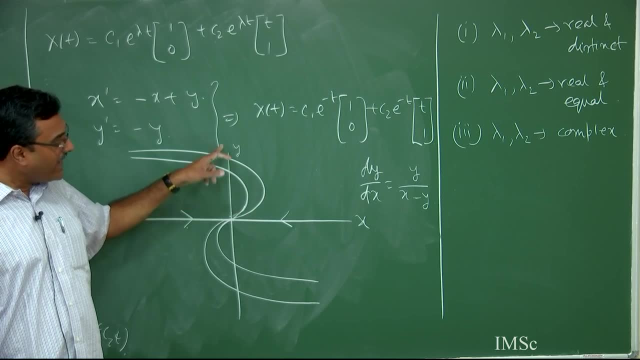 So the solution trajectories, they are parallel to the y axis. So therefore you have a turning point here. Similarly, if you choose some points on y axis, on the positive direction and as well as negative direction, you can find that there is a tangential direction. 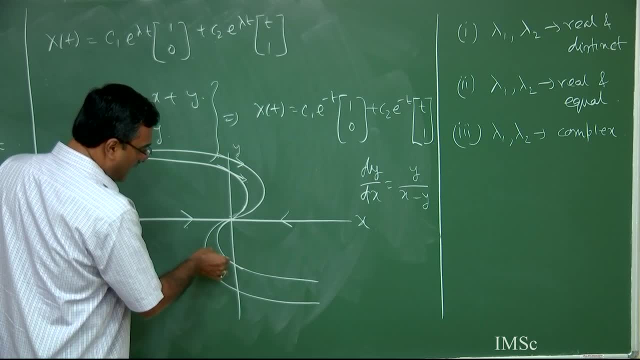 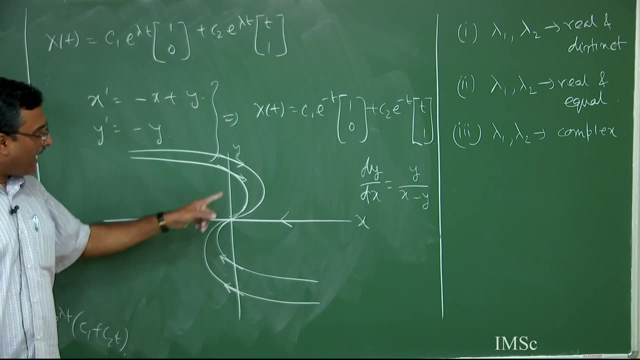 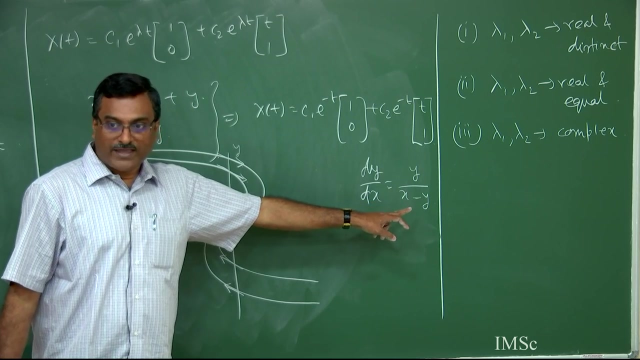 they are pointing towards this direction And, in this case, you will be having this direction. So, therefore, combining this idea and the fact that tangential direction they are pointing to the solution, trajectories are parallel to the y axis, along the line x equal to y. 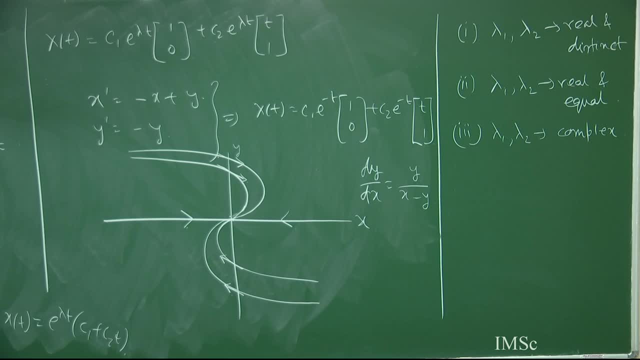 we can speculate. this is the phase portrait for this system. So now if we summarize the solution for two variable linear system, then we can say that any matrix capital A, that is of the form alpha, beta, gamma, delta, that can be converted to: 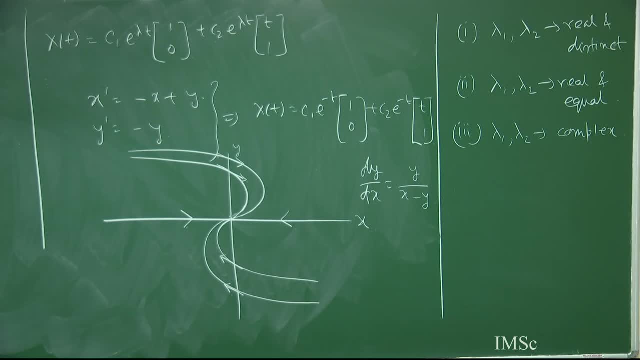 any one of these three forms, This one or lambda, 1, 0 lambda and number 3, that is alpha, beta minus beta alpha. So we have the idea of the finding solution for any one of these three system And Jordan canonical form give us the opportunity to understand how the linear 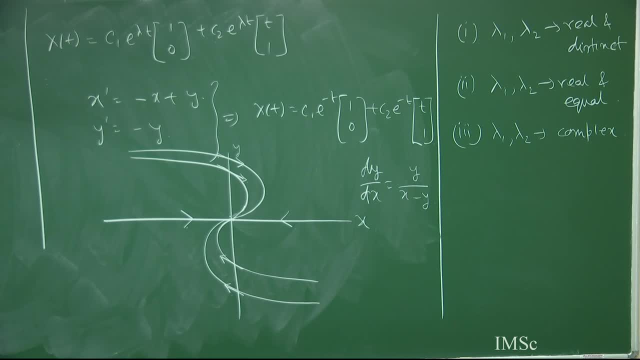 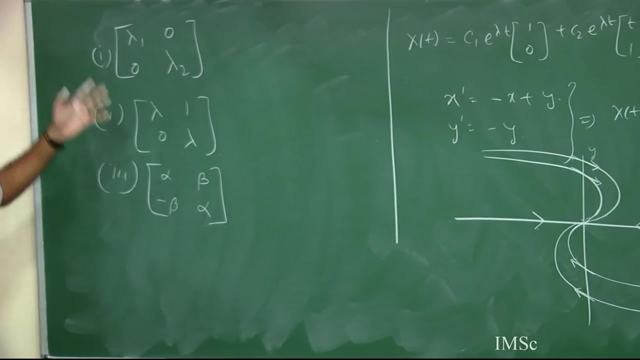 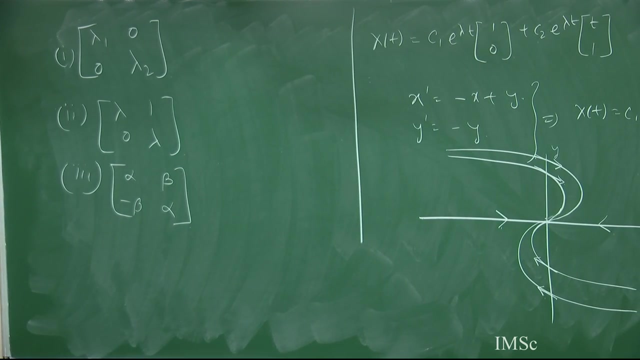 system can be converted to a transform system where the coefficient matrix is any one of these three Jordan canonical forms. So then you can find out the solution and accordingly you can find out the nature of the solution trajectories, that is, the phase portraits, And this idea can be extended to three and higher dimensional system also, And here I 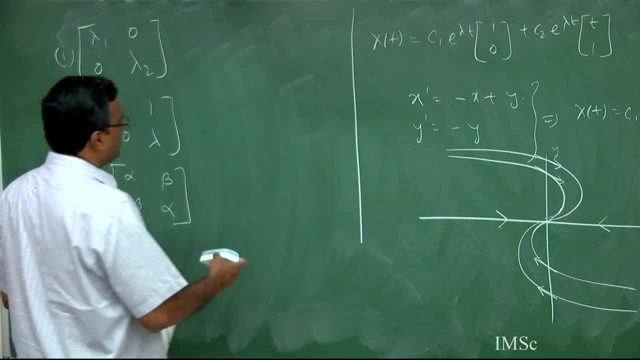 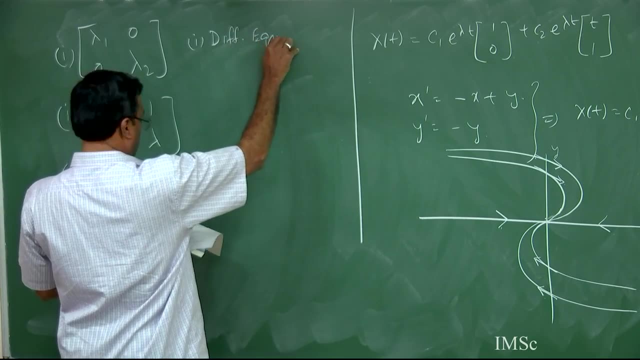 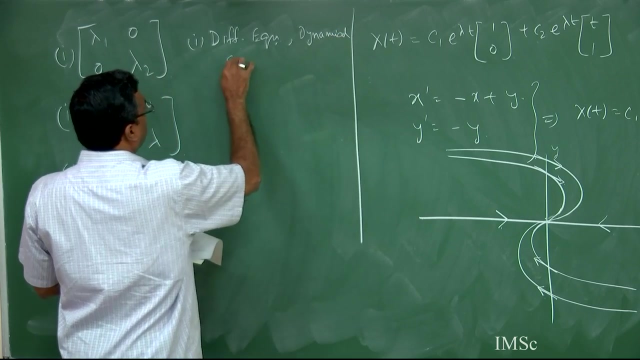 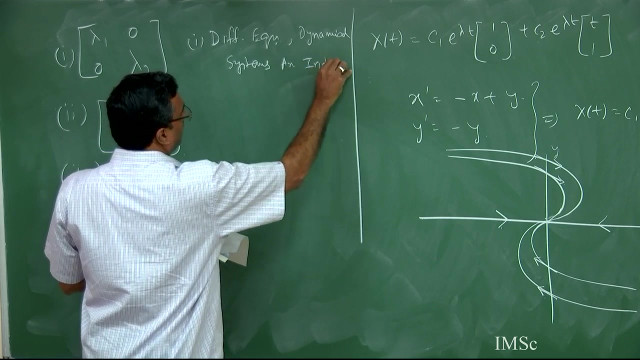 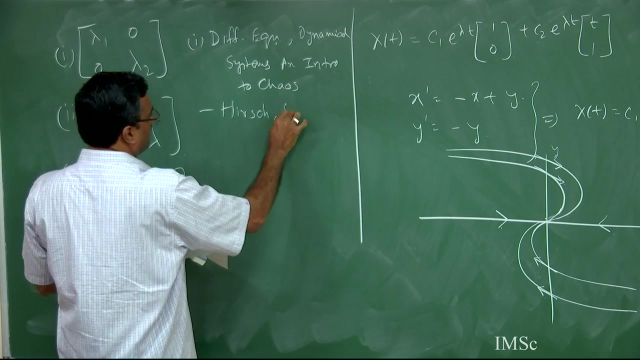 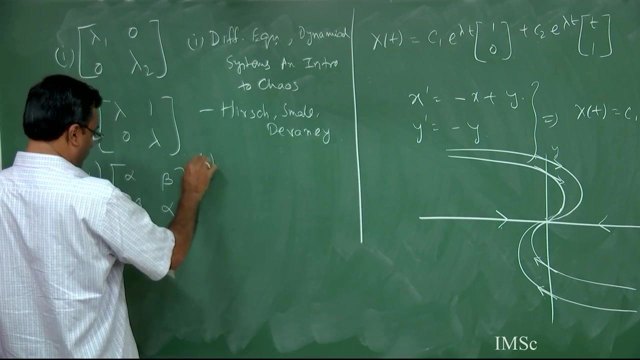 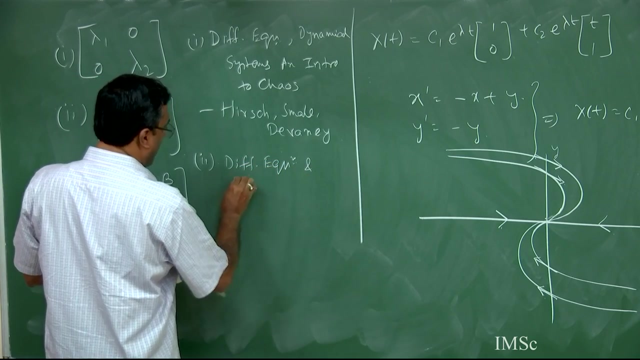 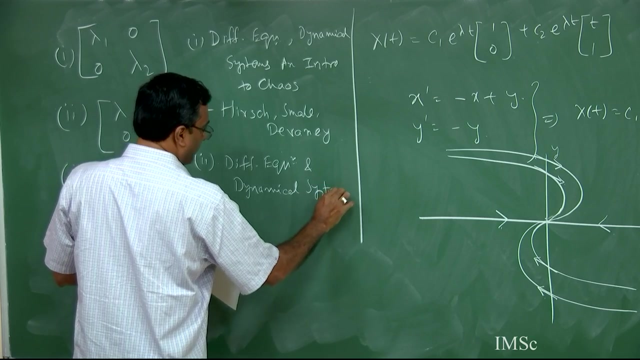 just give you two references that you can see for further details: Number 1, that is, differential equation, dynamical systems and introduction to chaos by Heath's smell and device, Page 1 of 15, bye bye 1 a. and number 2, differential equations and dynamical systems by L Parkour, for further 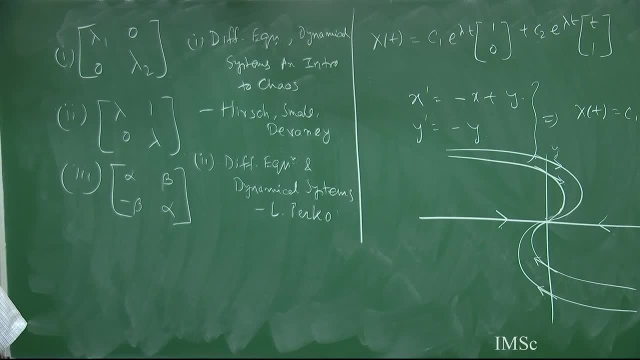 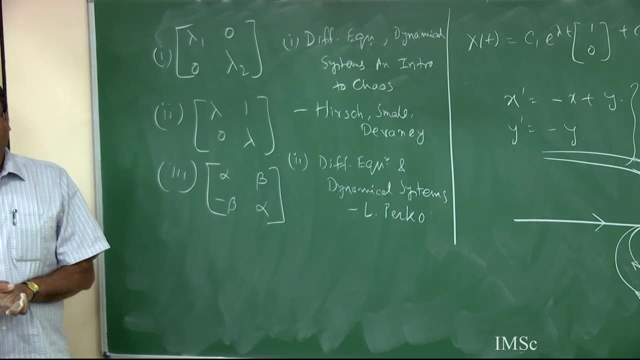 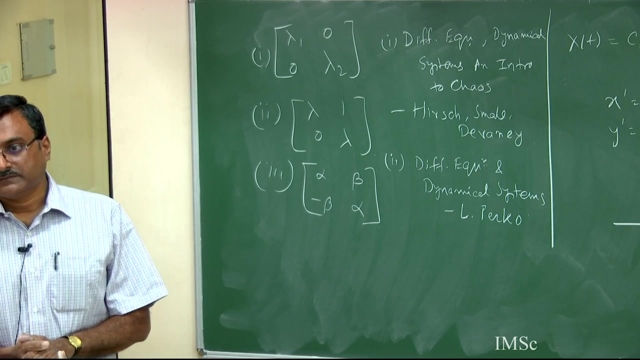 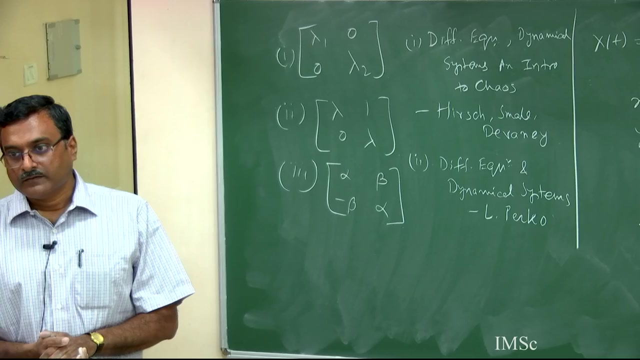 details right. So do you have any couple of one or two quick questions? Yeah, So there is a case that both the things are real. one is distinct somewhat. Yes, So in the case for the post phase, for real and distinct, we get somewhat of time. 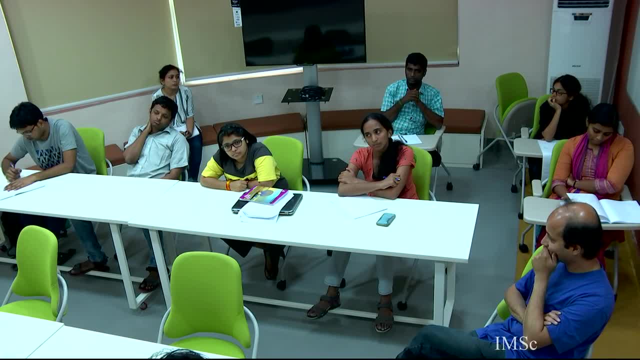 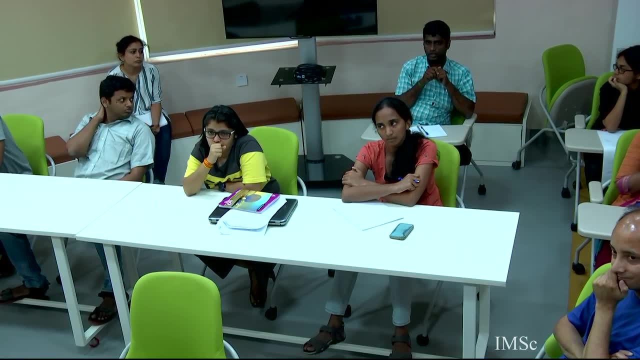 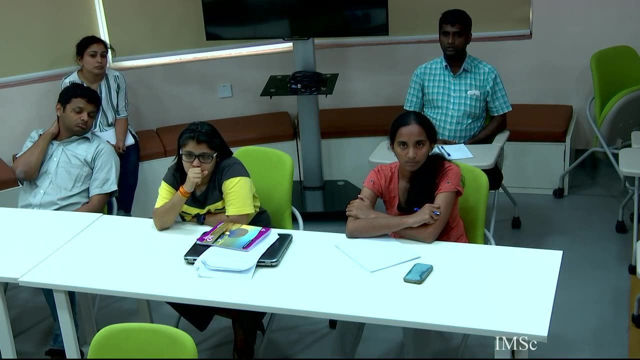 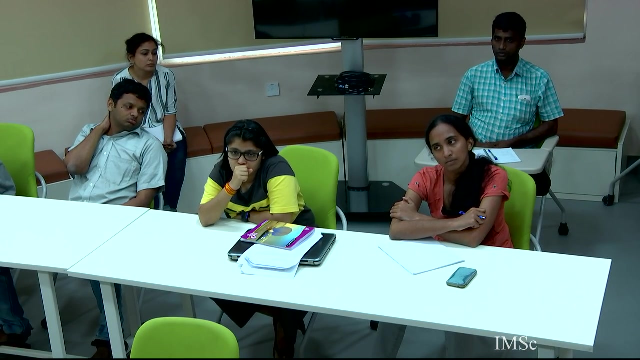 Yeah, For real and equal. we get Yes. 3 by 3 matrix. 3 by 3 matrix. the idea is that, first of all, you can find out the general solutions and there are different types of combinations Because in case of 3 Eigen values, all of all 3 of them- they are real and distinct. real. 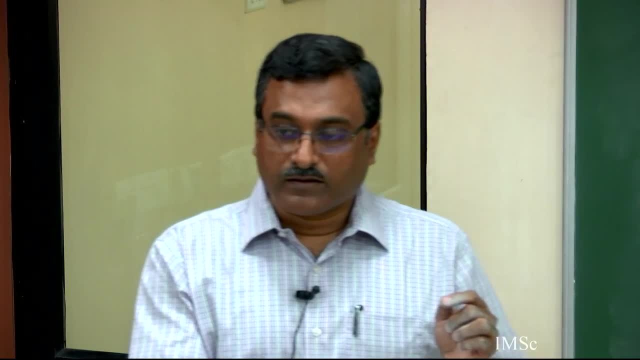 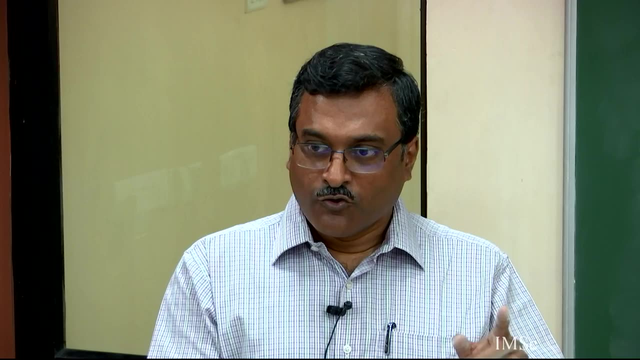 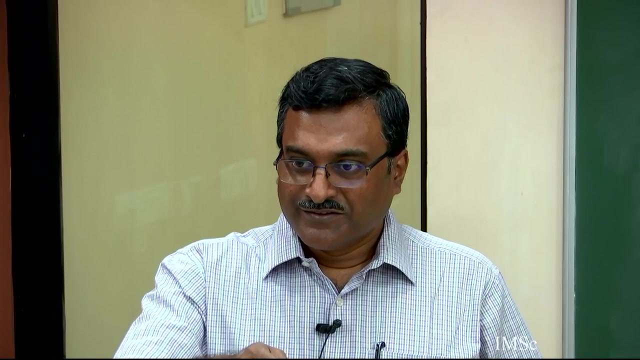 and distinct, but that will be combined with other different cases. That means 2 Eigen values are negative, 1 positive, 2 positive, 1 negative. So first of all you need to find out again the straight line solutions right, Because your transform system will be lambda. 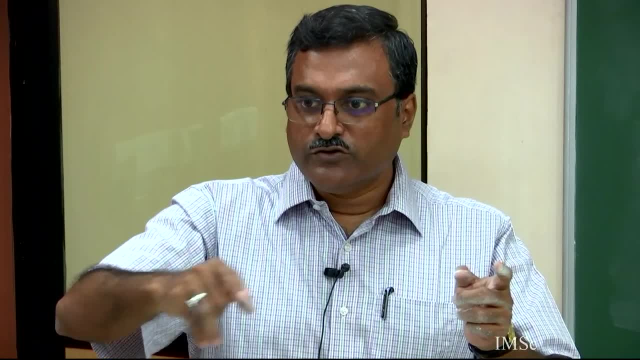 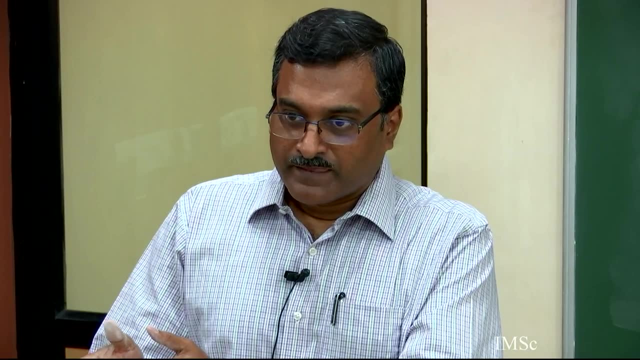 1, 0, 0, 0 lambda 2, 0, 0, 0 lambda 3.. So then, your 3 straight line solutions are x axis, y axis- Yes, And z axis. Then you can consider the case. lambda 1: negative lambda 2: negative lambda. 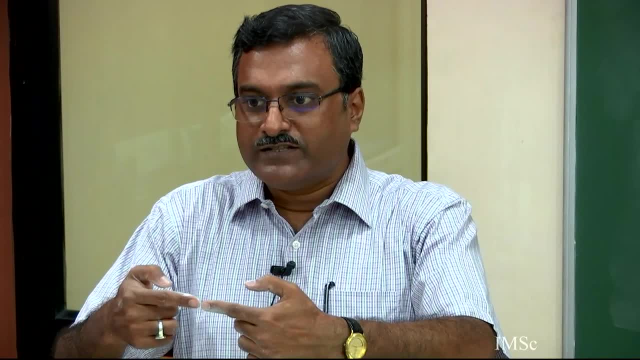 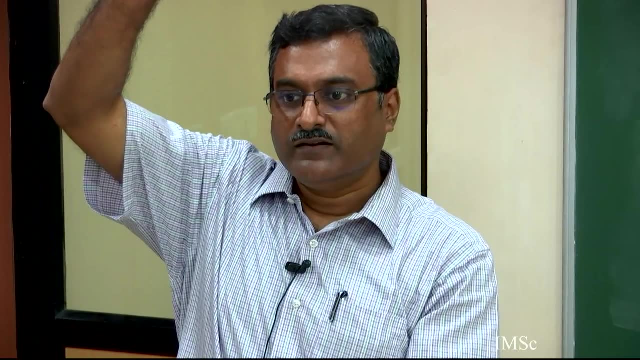 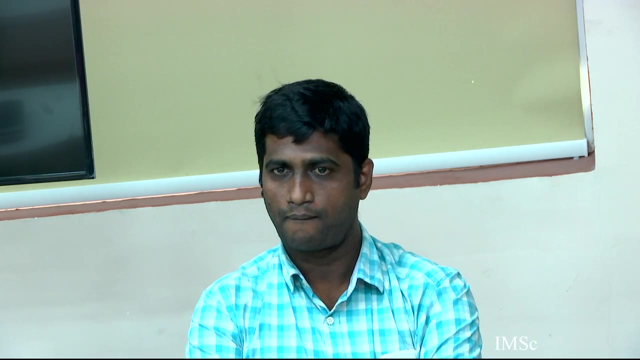 3 positive. So along x axis trajectories will be converging towards origin, along y axis trajectories will be converging to origin, but along z axis solutions will be diverging from the origin. And then you need some preliminary ideas about the curve and surfaces in 3 dimension. 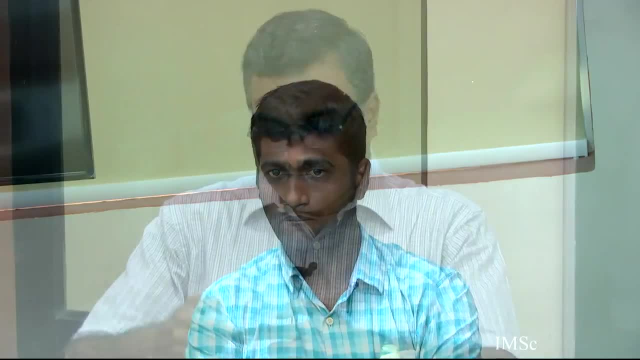 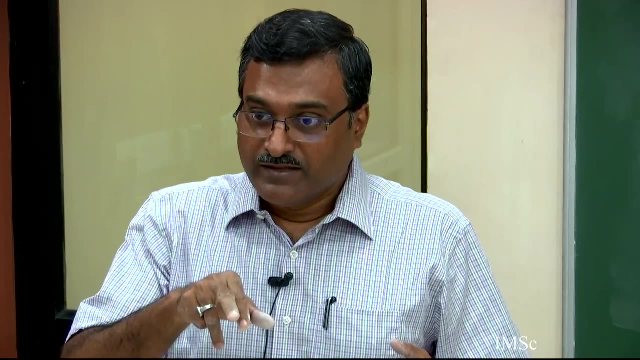 that is, 3 dimensional geometry. What will happen? That in this case, what you are having: 2 Eigen values. there are 2 different cases. That means those 2 Eigen values which are negative, they are equal or not. If they are not equal, then you will be. 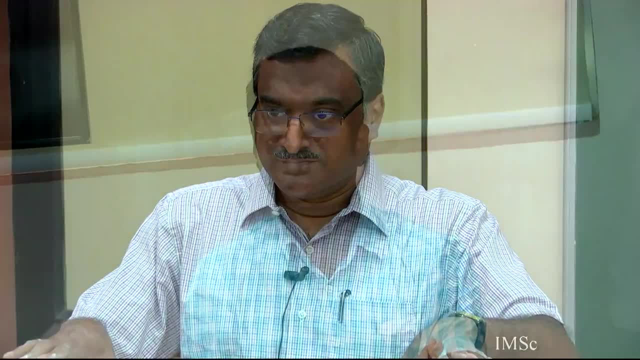 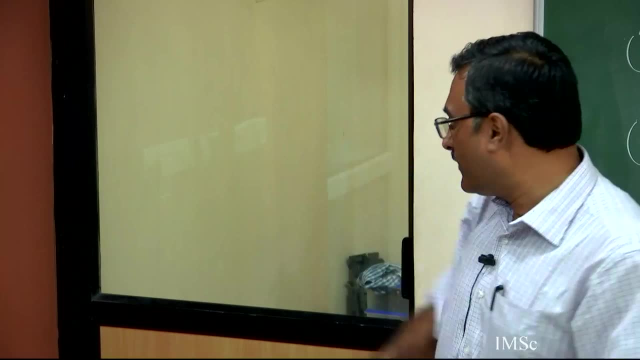 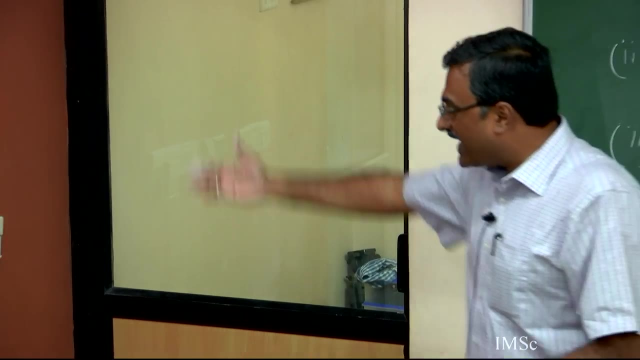 having some parabolic like structure on x- y plane, right, But as along z axis, the solutions are diverging towards infinity. So then you can just try to think about: this is your z axis, this is your x axis, this is your y axis, So plane will be looks like this one. 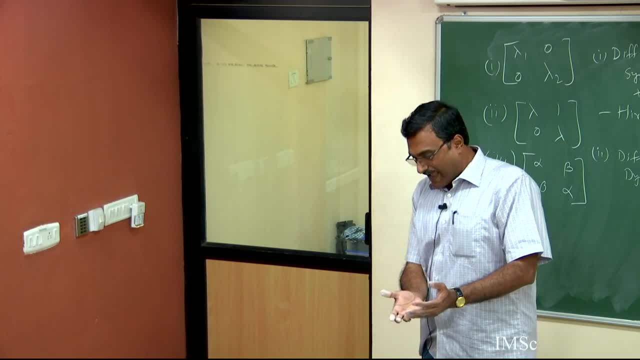 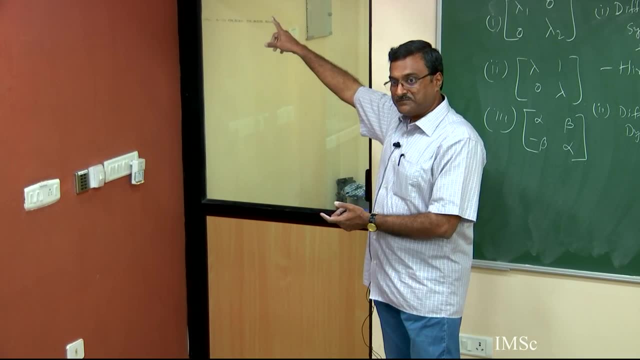 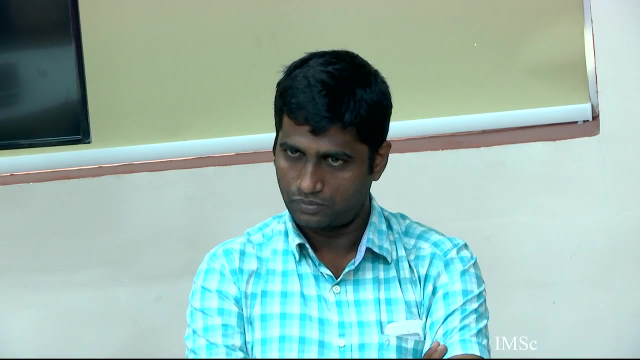 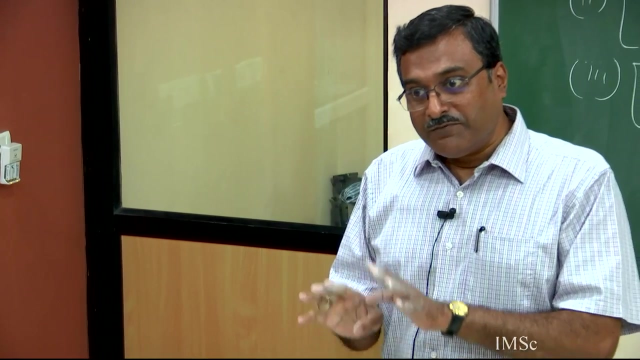 Right, Because it is approaching towards origin along x axis and y axis, but diverging towards infinity along z axis. right, Similarly, if you have both the Eigen values- real, distinct, negative and equal. real, distinct, negative and equal- but able to produce 2 linearly. 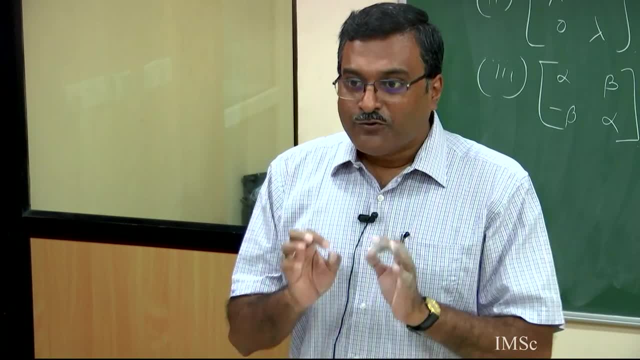 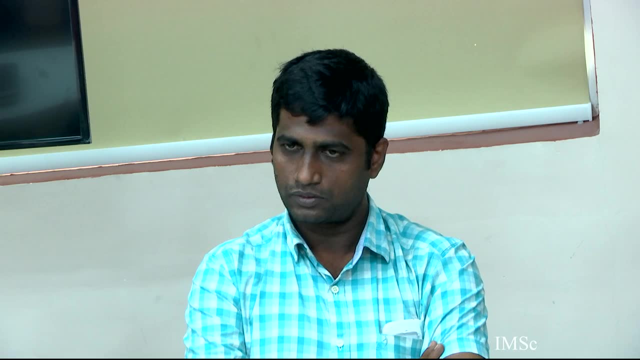 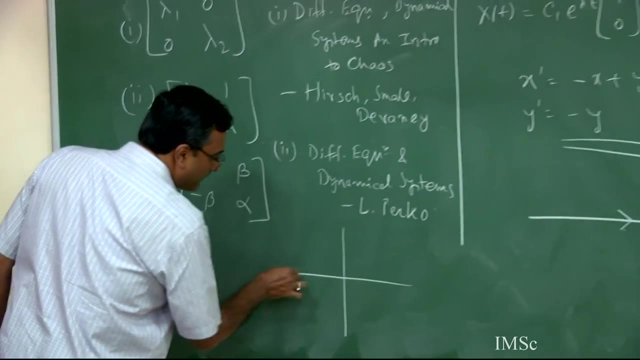 independent Eigen vectors. Can you tell me what will be the phase portrait in 2 dimension? Just 2 dimension. that I have not covered in my lecture. It is a very good question. You just try to understand that in that case solution trajectories will looks like this one, Because all the solutions they 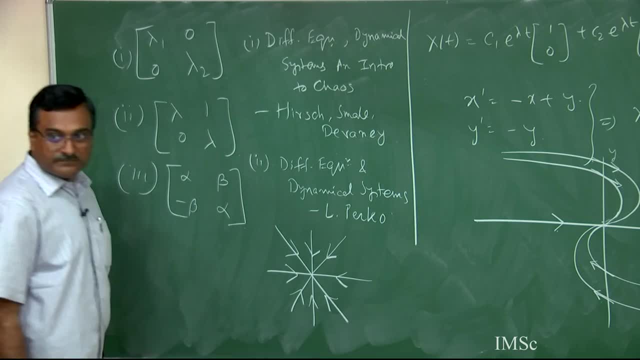 are actually straight line solutions: 2 real equal negative and equal right. So this is the square one, which is straight line solution. That means you have got a curve, you are having an x- y plane and then you are having a union. 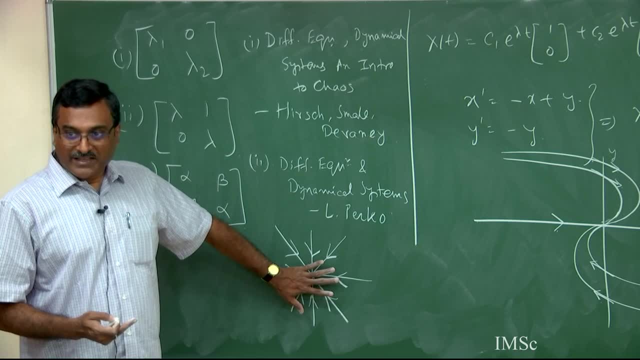 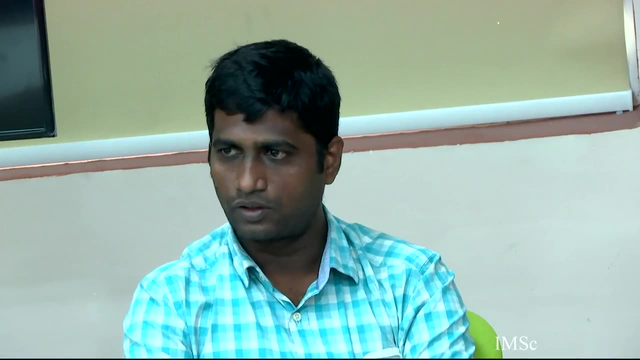 of two kind of vectors or an, even a linear face portrait. So you have the x- y plane with negative Eigen values. Yeah, Both are negatives, Both are negative and they corresponds to 2 linearly independent Eigen vectors. Then you are having this kind of structure, So along x- y plane. maybe you are having this structure along z axis. it is repelling outward, So then you will be having the corresponding face portrait. Not You are going for diagonalization, but you are using aelos. Not It is a diagonalization, rather it is a method of Jordan canonicalization. 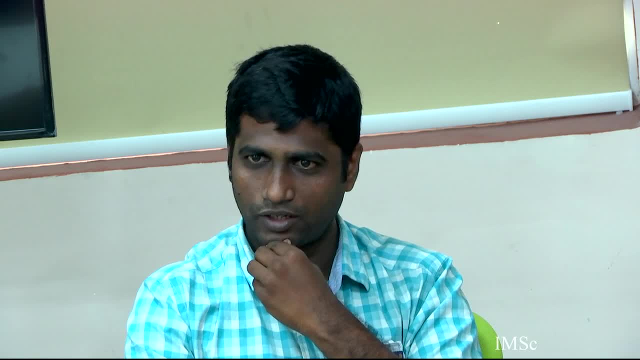 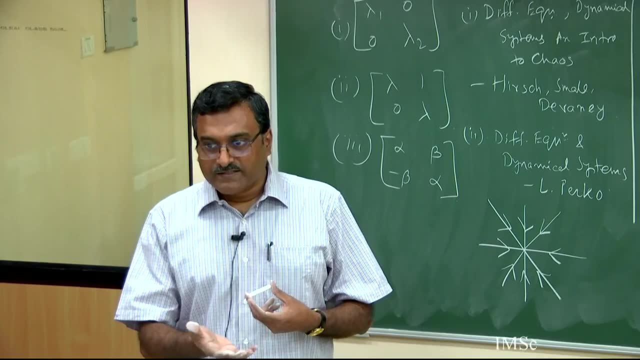 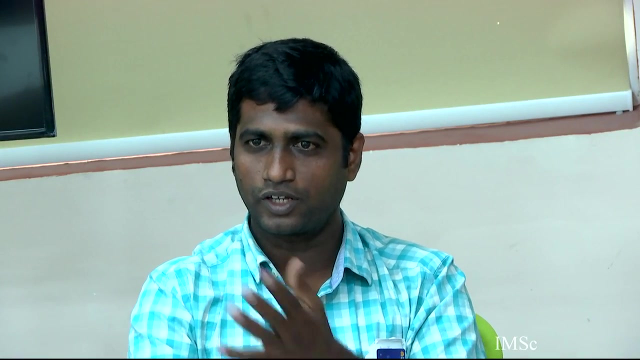 Correct. Okay, So it is a diagonalization of the. It is a diagonalization of the z axis. It is a method of Jordan canonicalization. In case of singular matrix, Jordan canonical form will results in some matrix with some of the Eigen values that is equal to 0. That is possible. that is possible. 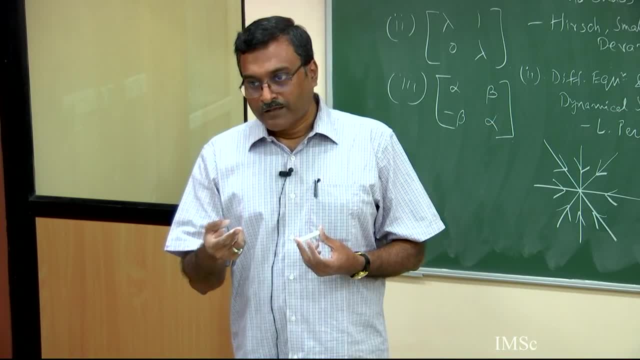 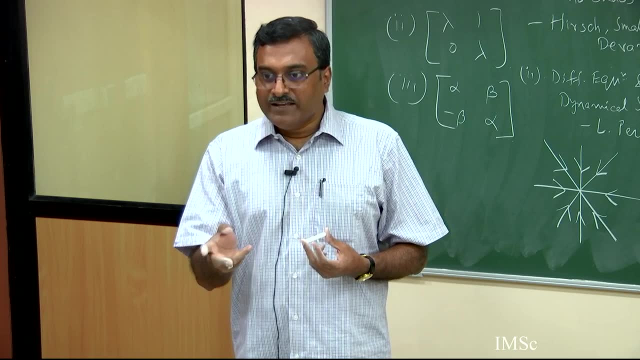 Because if you have one Eigen value, 1, and another Eigen value is 0, so two real Eigen vectors, they are real and distinct. So corresponding Eigen vectors are linearly independent. So once they are linearly independent, so by construction, your matrix T is invertible.